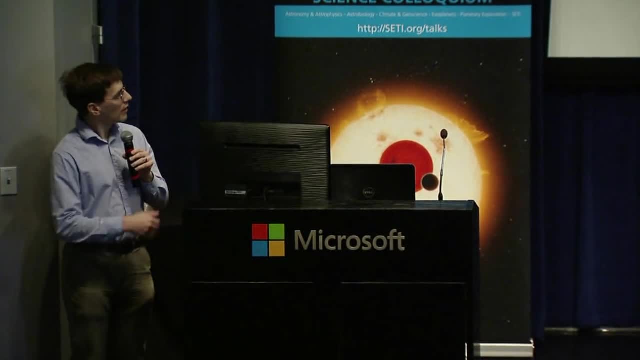 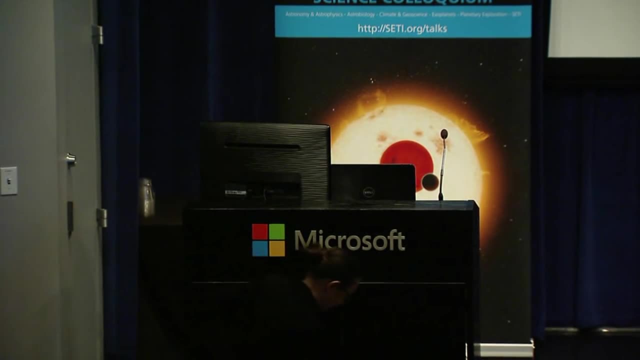 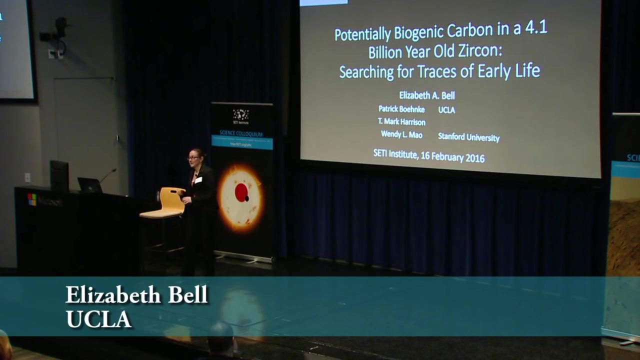 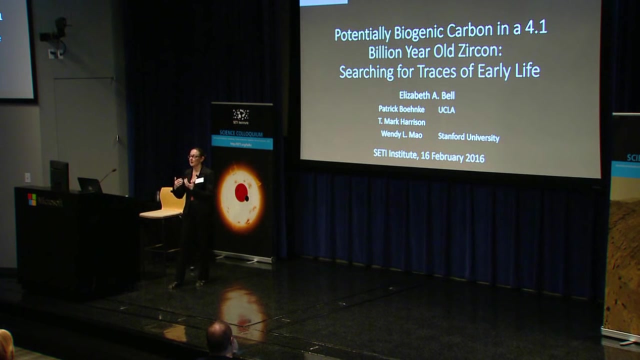 And she'll be talking about one of her most recent projects, which suggests interesting things about the history of life on earth. All right, Well, thanks for inviting me out here today, And I'm really excited to share with you some recent results we've gotten looking at carbonaceous materials in Hadean zircons and indeed pushing back the earliest evidence for life on earth. 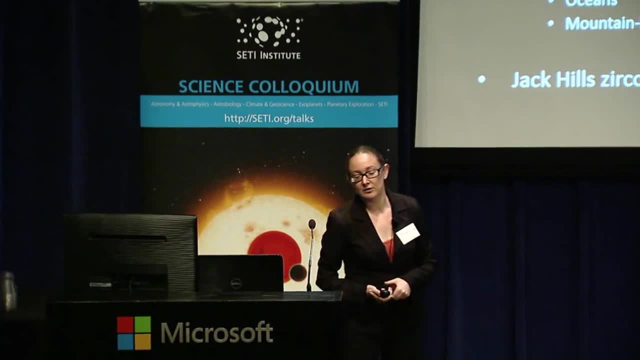 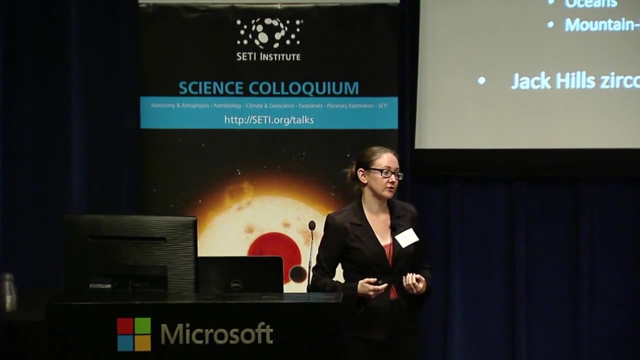 So what I would like to do right now is I'm going to start off with a brief history of what we know about the very early history of our planet and of our solar system, And so we know that the oldest solids in our solar system formed around 4.57 billion years ago. 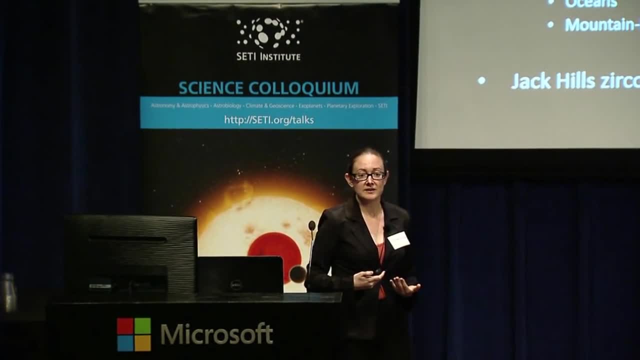 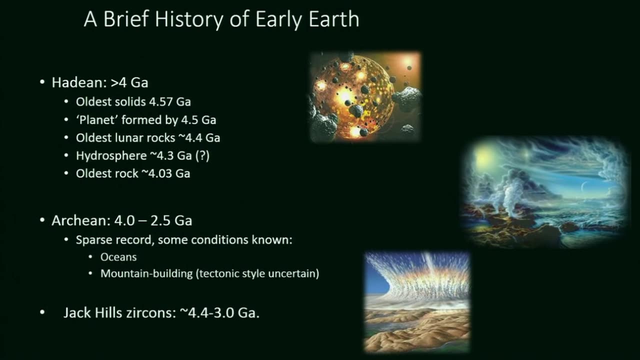 And the earth formed And, however, the oldest rock that we have yet found on earth today is only around 4 billion years old. These are the Acosta gneisses in Canada, So we have this around 500-billion-year period, for which we don't really have a rock record on earth. 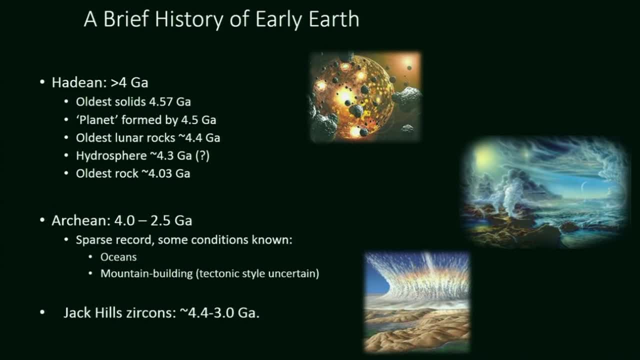 We call this the Hadean eon, So when I say Hadean, I mean older than the rock record, older than 4 billion years, And so this is a sort of mysterious eon in which we don't have all that much information that we can glean from having a rock record. 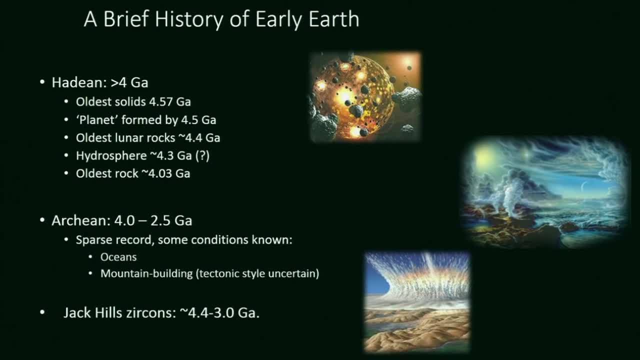 We do have some sparse samples from this region. These are detrital zircons from the Jack Hills locality in Western Australia that I'm going to be talking about for the rest of this talk. Now, following the Hadean period until about 2.5 billion years ago is what we call the Archean eon. 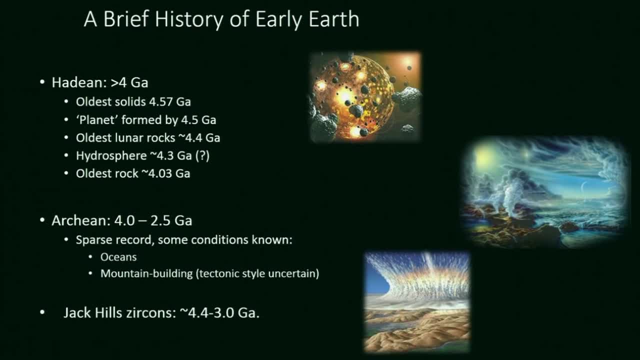 And we do have a geologic record, though it's quite sparse. It gets sparser with increasing age in the Archean. But we do know some of the conditions on the earth during this period. We know that there were oceans And we know that there was mountain building events of some type, although the tectonic style is uncertain. 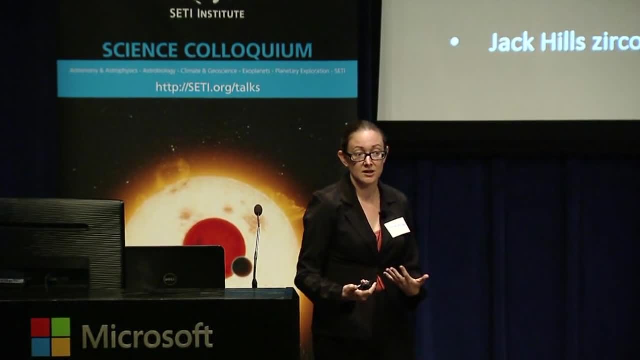 And indeed throughout the Archean and the Hadean. the existence of plate tectonics or potentially other alternative tectonic regimes is still a source of controversy, And one other thing that we're not entirely certain about is when life began. 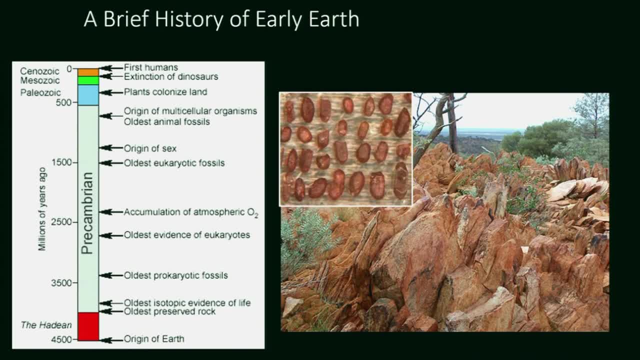 So we do have some ideas about the early history of life And in particular I'm showing you here we have. the oldest fossils have yet been found are a little less than 3.5 billion years old. These are microfossils in the Pilbara Craton in Australia. 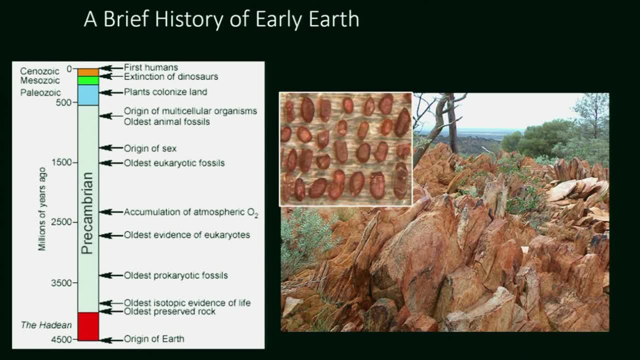 And the oldest isotopic evidence for life. these are carbon isotope ratios that are also going to form. much of the basis of my talk- is just a little older, at 3.8 billion years ago. Now, if you think about this number- 3.8 billion years- 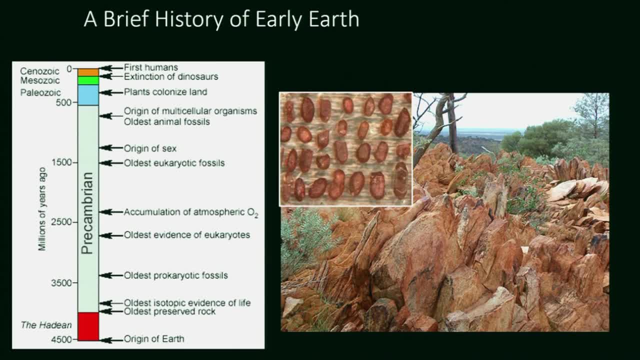 whereas the oldest rock that we have yet found is 4 billion years old. is this a coincidence that we're finding the earliest evidence for life so soon after the rock record begins? or is this more of a preservation effect? In fact, do we have the origin of life? 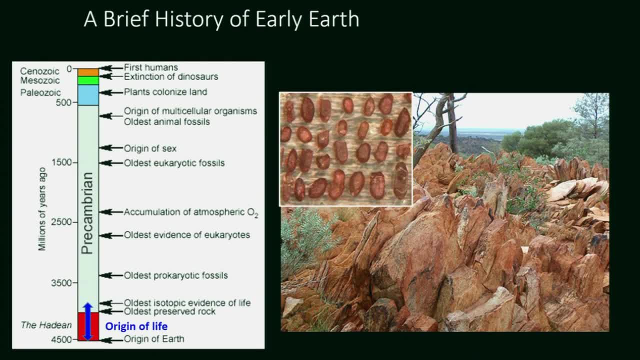 occurring somewhere much further back into the deep Hadean and we simply don't have the rock record to tell. Now, I mentioned that we do have some record of the Hadean, and what I'm showing you here is the Jack Hills locality in Western Australia. 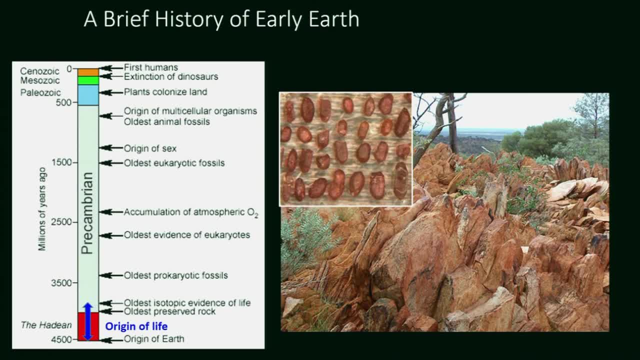 What you're looking at is a 3-billion-year-old sandstone, So it was deposited 3 billion years ago, And when I'm talking about detrital zircons, so that This is an example, These are actually zircons from this rock. 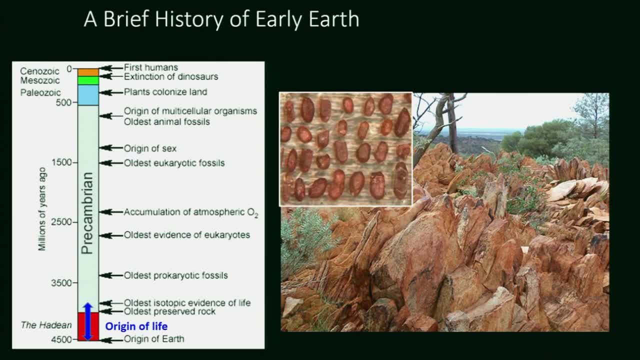 from the Jack Hills. So zircon is a mineral that is very useful for many geochemical purposes, and detrital just means that it has been eroded out of its original rock. It's taken out of its original context and we now find it in this sedimentary rock. 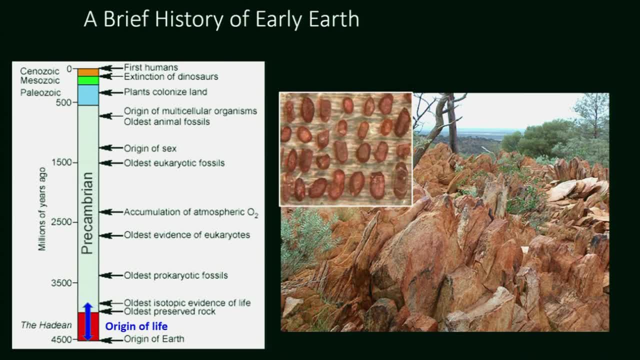 So each of these grains, they are, imagine, about 100 or 200 microns long. 100 microns is about the width of a human hair for scale there- And so this 3-billion-year-old sandstone hosts zircons that range between 3 billion years. 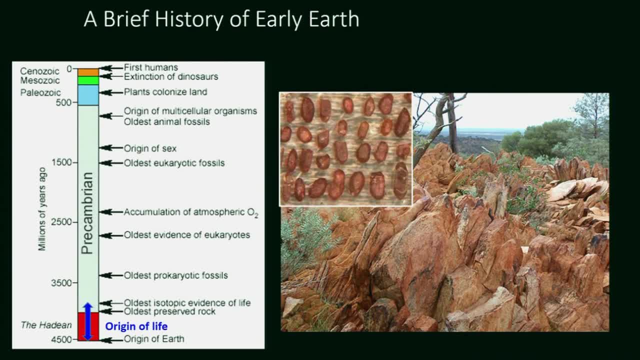 and nearly 4.4 billion years in age, And somewhere between 3 and 5% of the zircons in this rock are older than 4 billion years, and they are our best-known window into this Hadean period, And so these zircons. 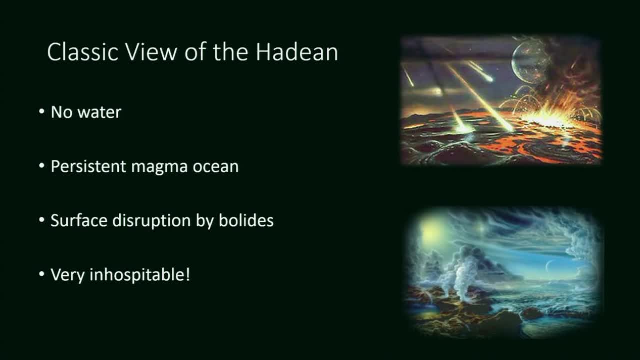 since they've been really thoroughly investigated geochemically over the past decade or so, have really changed our view of the Earth's first few hundred million years. So we're going to think now about the classic view of the Hadean, the very early period of Earth's history. 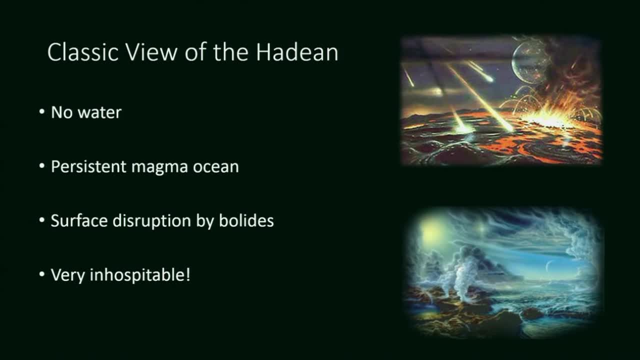 This is something that you can find often in textbooks today. It's also sort of been propagated into popular culture in many ways, if you think about the Fantasia movie and sort of the origin of Earth's sequence. So the classic view of the Hadean is that 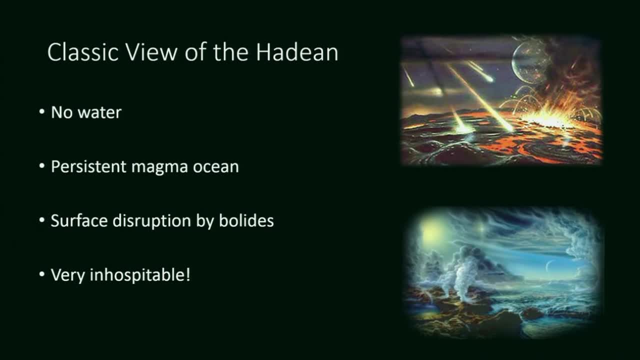 there was no water available on the surface. You have a persistent magma ocean hanging around for a very long time, a surface-disrupted ocean, very strongly by bolides, that is, meteorite impacts in some very inhospitable and not the sort of environment. 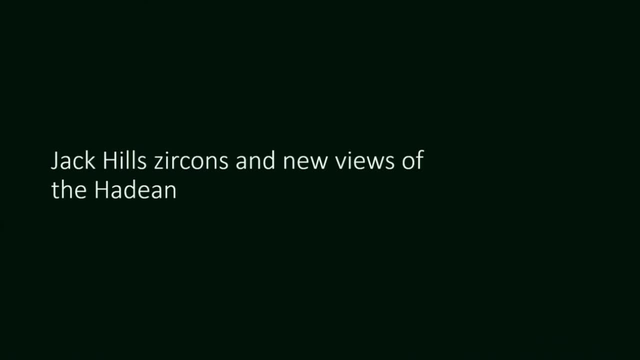 in which you would expect to find life. So the Jack Hill zircons have given us a very new view of the Hadean, and I'm going to go briefly over many of the lines of evidence that have been used to tell us that the Hadean 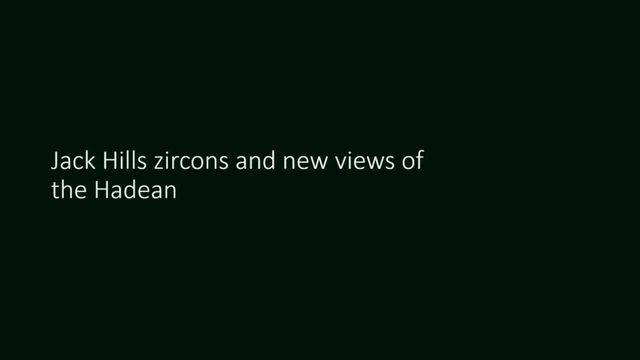 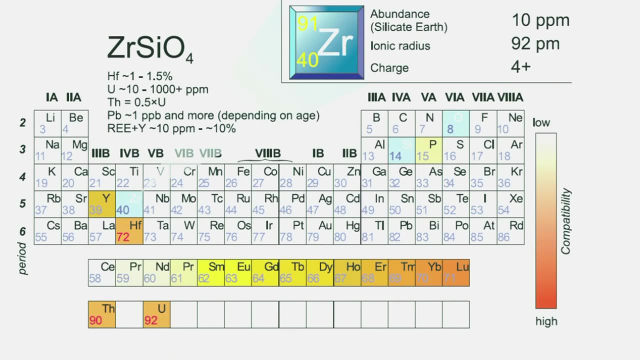 may have looked a lot more like the modern Earth than we had originally thought. So first I am going to go over what we know about zircon and why zircon is really an ideal mineral for many of these investigations. So I'm showing you here a periodic table. 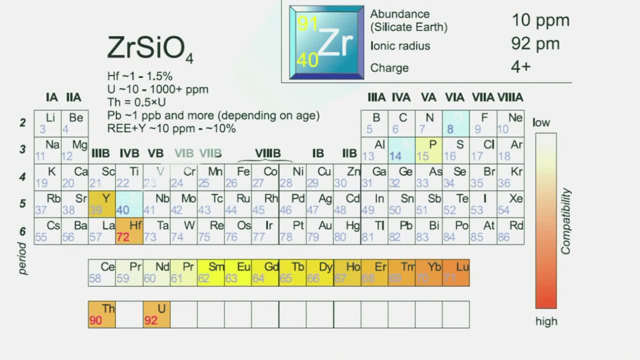 that is color-coded based on something we call compatibility. So when a geochemist talks about compatibility, we're saying: we have zircon, it's growing in a magma and if an element is very compatible in the zircon, then as the zircon grows it's going to. 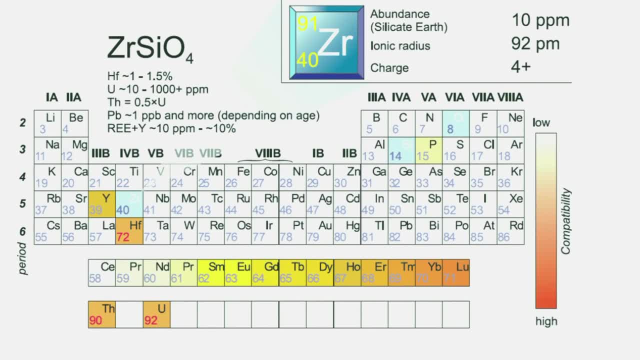 tend to be found in the zircon rather than in the magma. So we've got low compatibility to high compatibility with high compatibility, notably uranium with lead having low compatibility. So what this does is this leads to very high uranium-lead ratios. 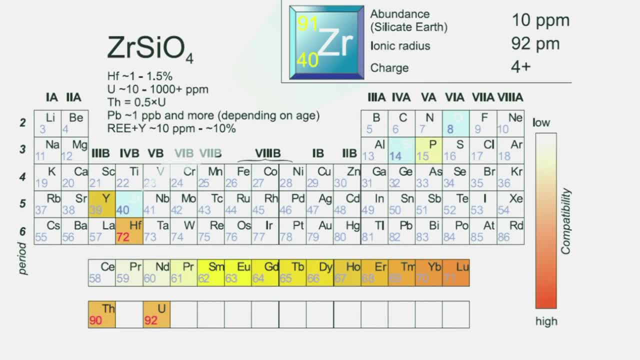 as zircon grows, and this is very helpful for geochronology, So uranium decays to lead to long-lived isotopes of uranium. these decay at known rates, and so zircon is really the premier geochronometer in a lot of geologic systems. 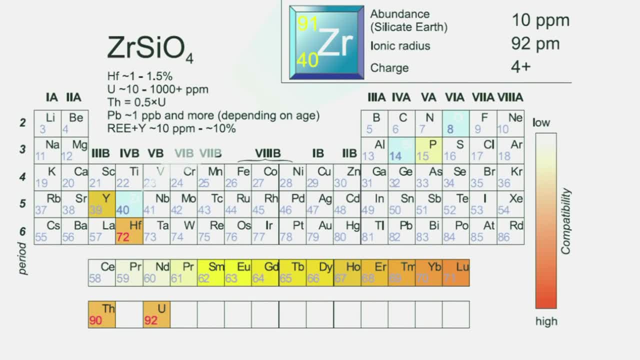 it's widespread in many igneous rocks and metamorphic rocks on the Earth and it is also very chemically and physically tough, So there aren't really planes of weakness through the zircon structure. it is very difficult to break it up Once it gets eroded out of its 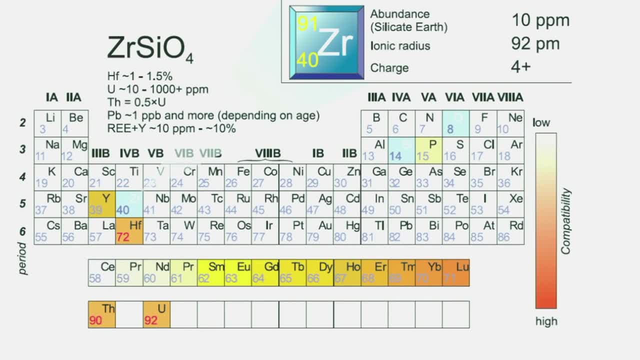 parent rock. you can often find it hanging around in the sedimentary environment for billions of years. Witness the fact that we still have 4 billion year old plus zircons on the planet. Now some other useful things about zircon we're finding out here: titanium. 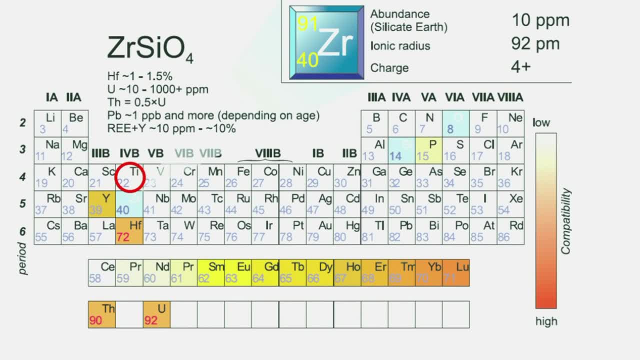 which is one of the elements which is not very compatible in zircon, but it tends to the extent to which we find titanium in zircon is very sensitive to temperature, So the concentration of titanium ends up being a very good thermometer for zircon. 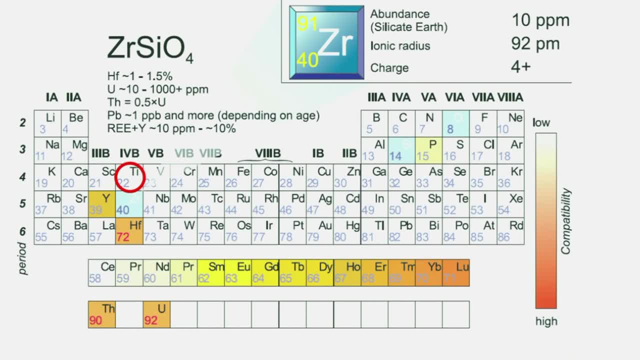 and we can get the crystallization temperature of that particular grain- Another thing that's useful. so we have the structural components of zircon here. we have zirconium, silicon and oxygen Abundance in zircon. we can look at oxygen isotope ratios. 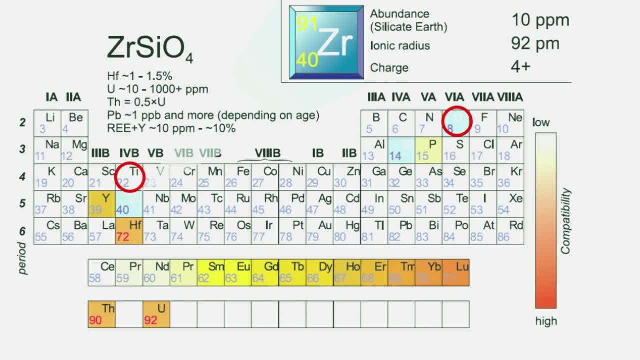 in zircon at very high precision, and this can tell us something about the materials that went into forming this magma that grew this zircon. Another thing that you'll notice is that carbon is also not very compatible in zircon. we don't find it at very high levels. 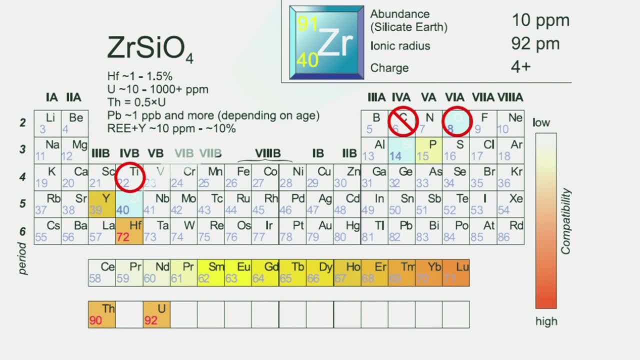 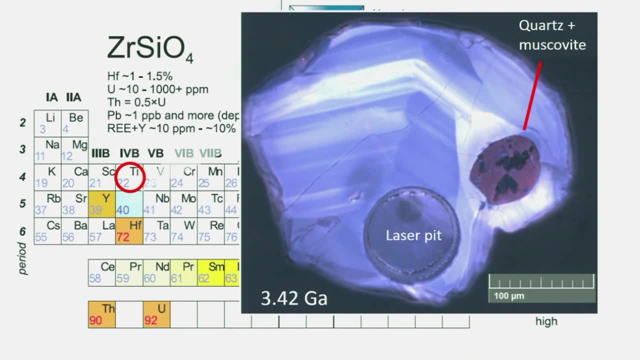 in zircon. so when I'm talking about looking for carbonaceous materials in the Hadean, what do I mean? And to answer that, I'm going to put up this image. so this is a cathodoluminescence image of a Jack Hill zircon, this particular one. 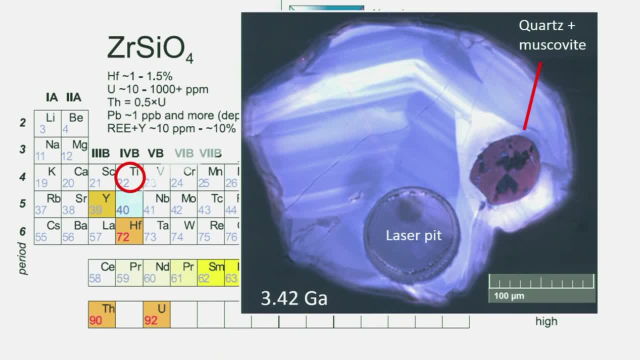 is around 3.42 billion years old, so it's one of the younger ones. But so what you're seeing here, this is this hole here. this is a laser pit from a previous study and this is a cathodoluminescence. 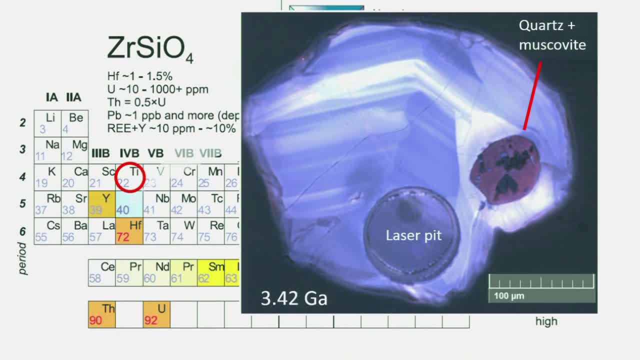 image, which means that we have bombarded this zircon with electrons and it is giving off visible light, And one thing that you can often find in magmatic zircons is this nice sort of growth zoning. So we've got. so this is called. 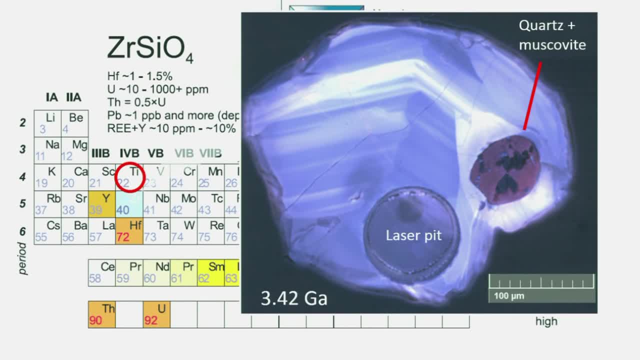 regulatory zoning and it's a bit disrupted up in this region, but this is often characteristic of magmatic zircons, and one other thing that you can see very nicely in this cathodoluminescence image is that we've got something over here that is not zircon. 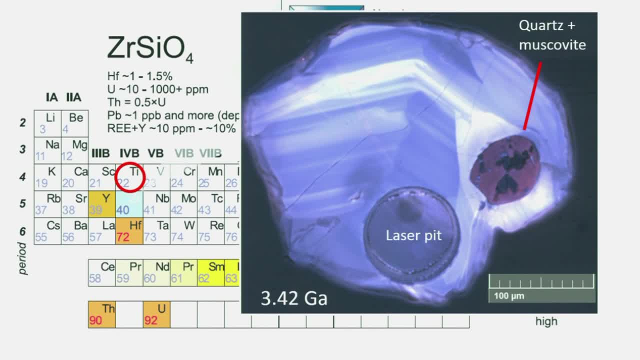 So this is what we would call an inclusion of, in this case, quartz and muscovite. so in this case we had a crystal of this quartz with some muscovite in it that the zircon grew around as it was growing. 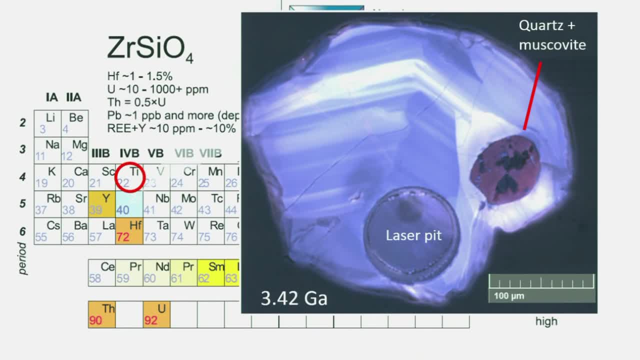 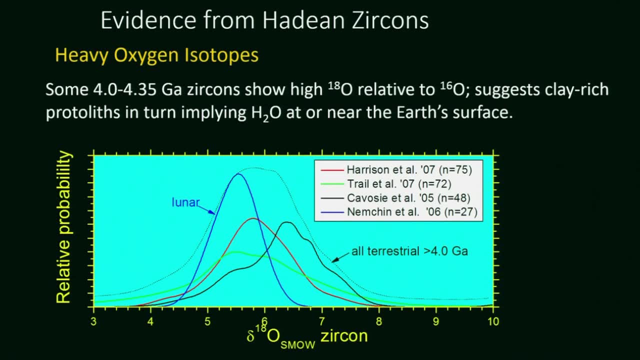 in the magma, and so what we propose to do is we are going to go through the Jack Hill zircons and see if we can find inclusions that are, in fact, of carbonaceous minerals. Now we're going to go over some of the other evidence. 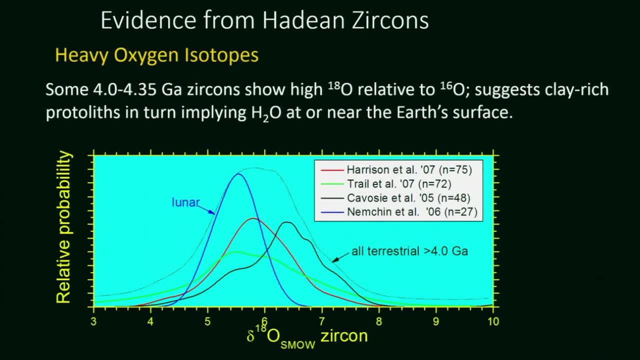 from the Jack Hill zircons. that has really given us this very new view of the Hadean. So I'm going to talk first about oxygen isotopes and what they can tell us about water on the early Earth. So I'm showing you this: 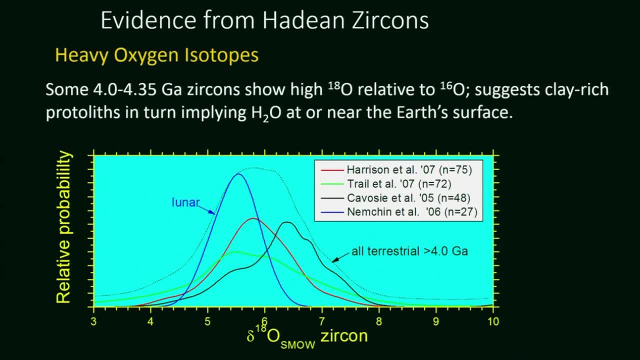 quantity here, which is delta-18-0,, and this represents the ratio of oxygen-18 to oxygen-16.. So oxygen-16 is the most abundant isotope of oxygen and the oxygen-18 to oxygen-16 ratio in Earth. 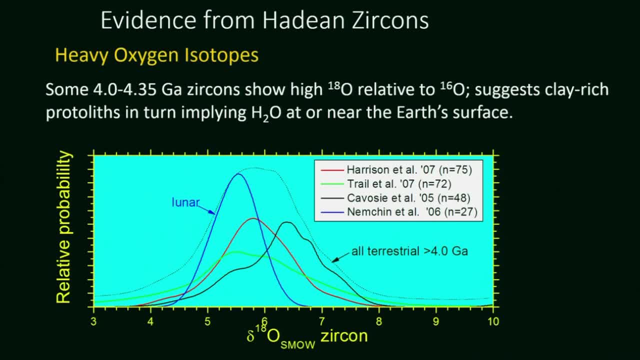 if you look at materials erupted out of the Earth's mantle, say at a mid-ocean ridge or at Hawaii or Iceland, they fall into a relatively narrow range of values at around 5. this is a parts per thousand or per mil scale here of 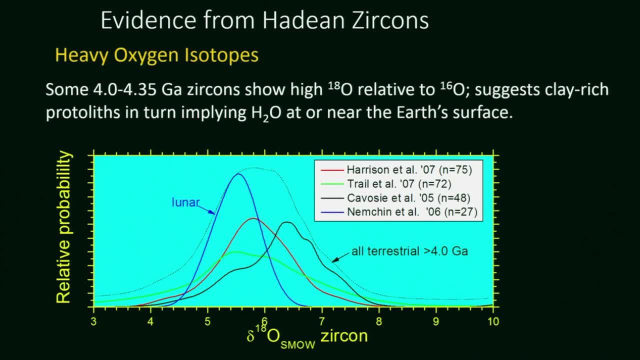 delta-18-0, and unless they had been contaminated by materials from the surface. Now, the reason materials from the surface can contaminate these mantle lavas is that when you alter or when you weather rocks in a relatively low temperature, aqueous environment, like near the surface. 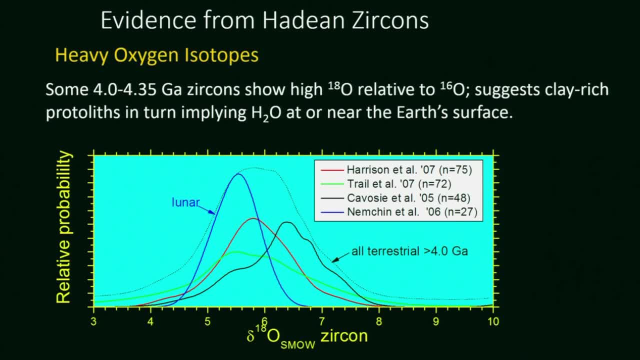 you form clays, And clays tend to be very rich in oxygen-18 relative to oxygen-16. And so when you start finding these high delta-18-0 signatures such as: so these are compilations of Hadean Jack Hill zircons. 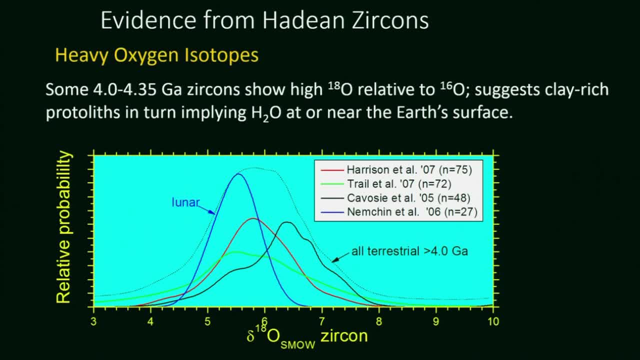 you can see we're stretching away from 5 up to 1008 per mil. This, when we see it in the modern day Earth, is indicative of sediments, And so if you were to go out on the modern day Earth and you find a, 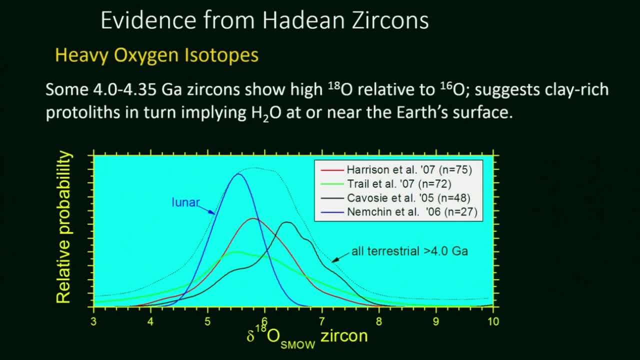 magma that was melted from sediments, you're going to find these high delta-18-0.. And so, around 2001, when people started looking at oxygen isotopes in the Jack Hill zircons, they find these high delta-18-0. 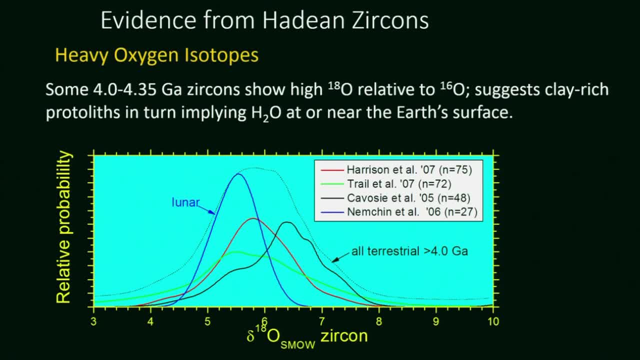 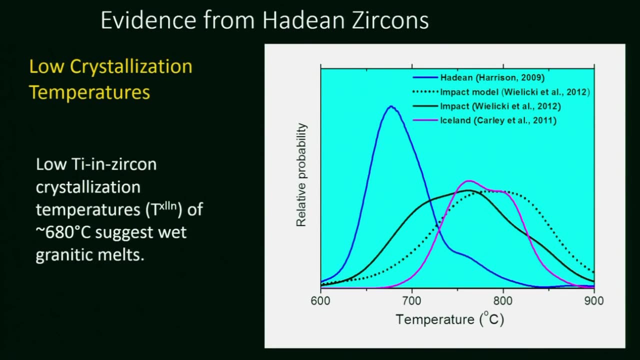 signatures in a substantial minority of the zircons, suggesting that there was a bit of sedimentary involvement in their formation. Moreover, these low temperature aqueous reactions suggesting a hydrosphere as early as 4.35 billion years. Now there are other. 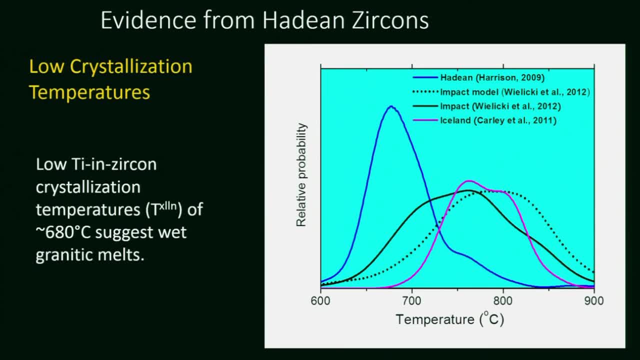 pieces of evidence that there could have been water involved in the formation of these zircons, And what I'm going to show you now this is that titanium and zircon thermometer that I mentioned before. So we've got this titanium and zircon thermometer. 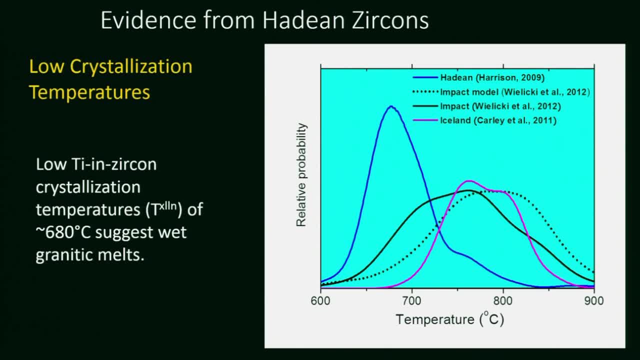 This is in degrees Celsius. Again, probability density functions In blue. here we have our Hadean zircons from Jack Hills And they cluster very tightly around an average value of around 680 degrees Celsius. So when you're looking at magmas on Earth, this is a very, very 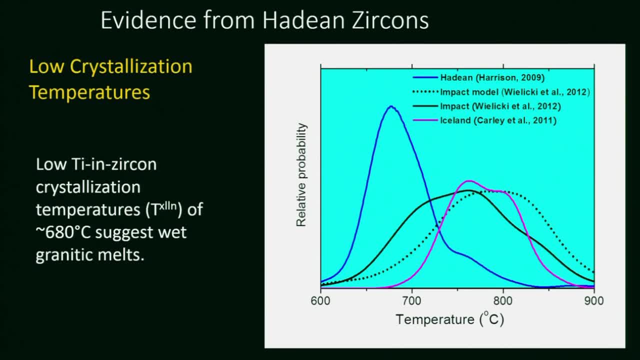 low number. This is not something that you find in a very wide variety of environments. This really requires hydrous and granitic magmas, And so what's special about granitic magmas is if you are to, if you're going to, partially melt the Earth's mantle. 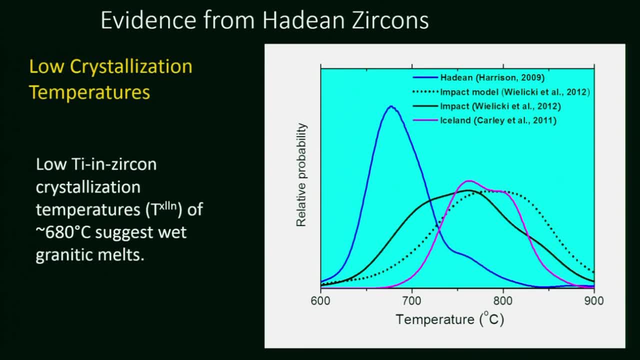 as you do at mid-ocean ridges, as you do at ocean islands like Hawaii, as you do at Iceland. you are the majority of material that you get out of. there is going to be something called basalt. It is takes extra evolution. 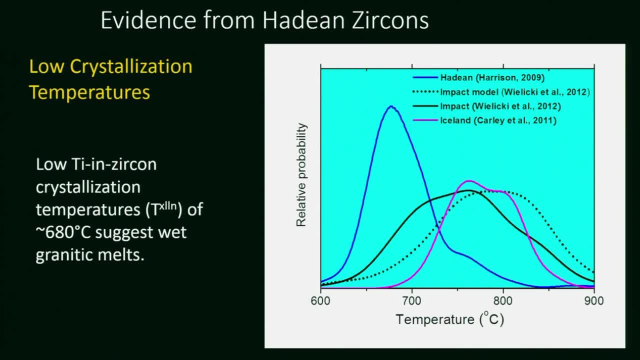 steps or evolutionary steps in magmatic processes. to get something like a granite, You have to either remelt the basalt or remelt another crustal material like sediments, And so the fact that we have, and you actually have, this relatively low temperature. 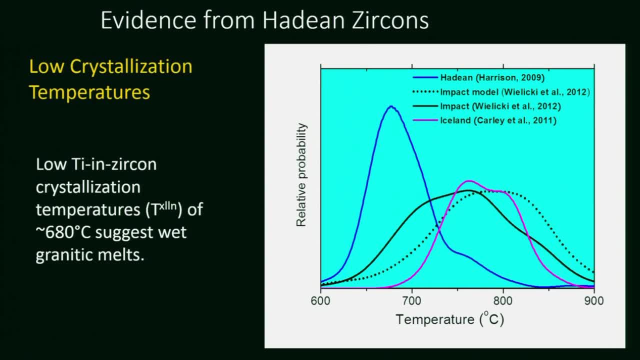 you need hydrous granite magmas. So this is another piece of evidence that we have water involved in the formation of these zircons And, moreover, that we might have some more evolved, almost continental-like crust early on. Now I've shown another couple of 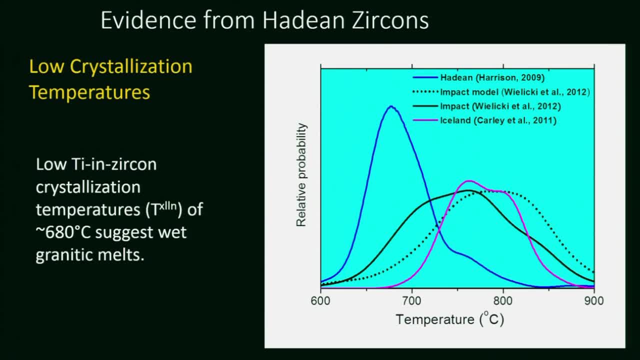 distributions here for comparison. So we have Iceland, So these are zircons from more evolved lithologies from Iceland. So you have basalts in Iceland and then a very sort of late-stage remelting of the basalts, You can get zircon-bearing. 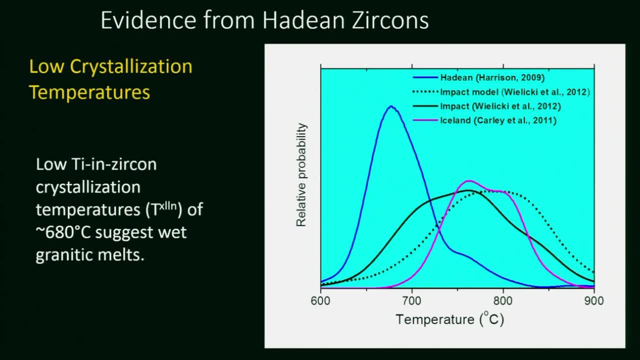 rocks. However, they do still tend to be at relatively high temperatures. You see, this is a broader distribution: relatively high temperatures. And I'm also showing you in the black curves here, zircons that are grown in impact melt sheets, So a large meteorite impact. 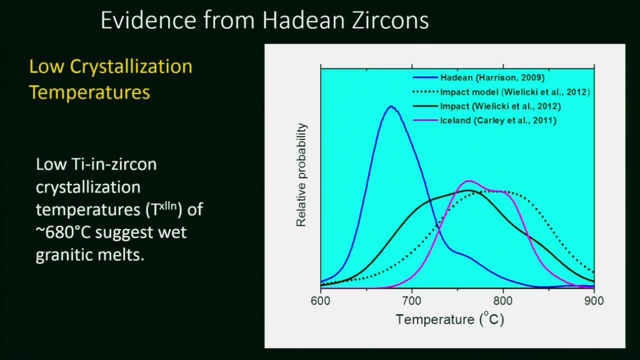 comes in, melts, the rocks that it hits and zircons grown in that sheet are going to have relatively high temperatures, Especially compared to these Jack Hills Hydian zircons. So it looks like either a basaltic sort of terrain like 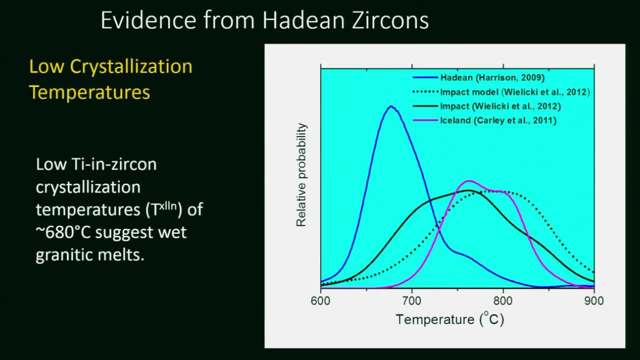 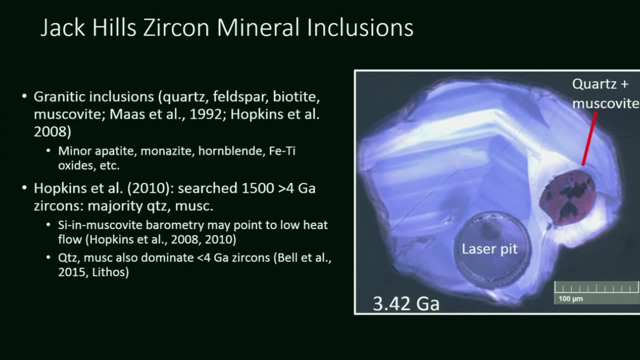 Iceland or impact melt sheet origin is really not going to dominate the Jack Hills zircons. Now. mineral inclusions: we've talked about a little bit, but these also play a very important role in looking at the origin of the Jack Hills zircons. 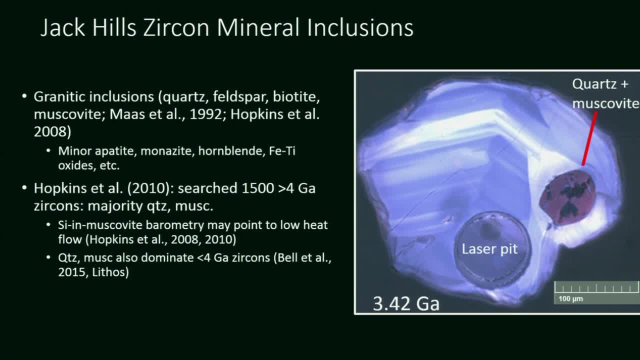 For instance, here's this nice quartz and muscovite inclusion that I showed you before. So the inclusions in the Jack Hills zircons have been looked at since the early 90s And very consistently the studies find very granitic looking. minerals. So if you're looking at a granite- one of the chemical differences from granite to basalt- so the more primitive basalt is going to have, it's going to be much more rich in iron and magnesium. Granite is going to be proportionally much more rich in. 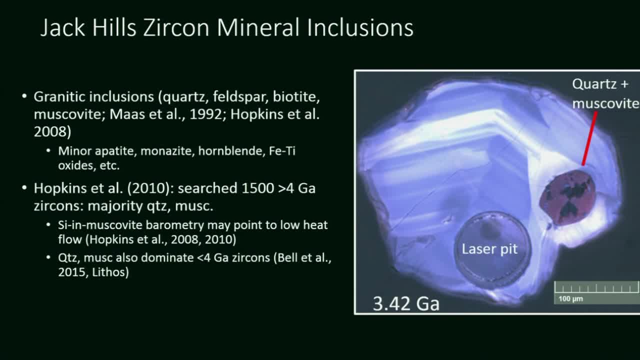 silicon and aluminum And various alkalis are also important. So we have things like quartz, which is silicon dioxide. it's a very common mineral. you can find Feldspars and micas are things that we see dominating the assemblage in these. 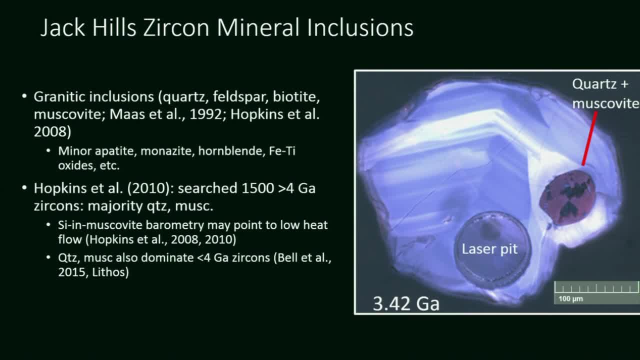 zircon inclusions, And they're also characteristic of granites on Earth throughout the period in which we can see granites in the geologic record, And in fact, at UCLA we've done quite a lot looking for inclusions in the Hadean zircons, In fact. 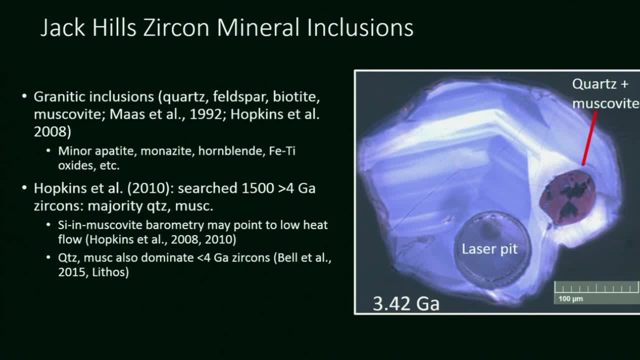 Michelle Hopkins, who's a former graduate student at UCLA, looked through 1500 of these zircons older than 4 billion years And she found that, in fact, the inclusion assemblage is dominated by the minerals quartz and muscovite. So what is muscovite? 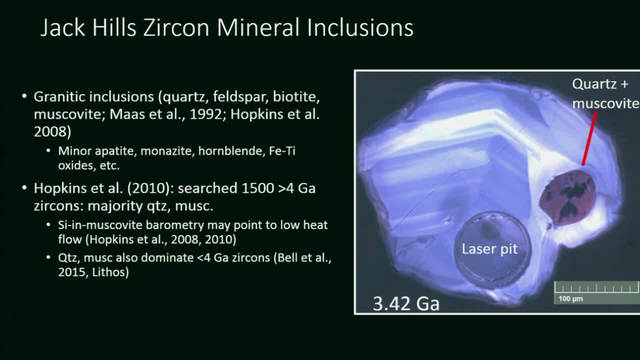 Muscovite is a mica and it is important for several reasons. One, it is characteristically found in highly aluminous magmas. So the way you get a highly aluminous magma, the easiest way to do that is to melt sediments. So this is. 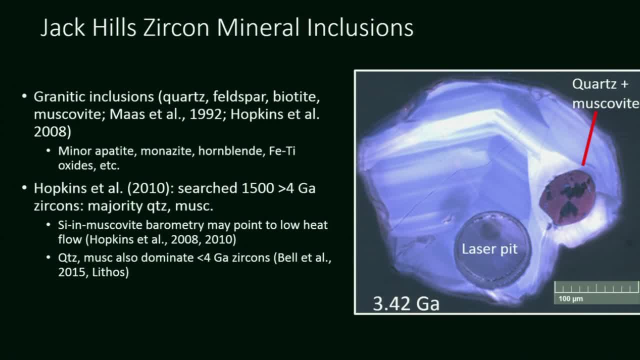 another line of evidence for this melting of sediments and this sedimentary origin for a lot of these zircons. Another thing that's very useful about muscovite is that the silicon to aluminum ratio of muscovite can be used as a barometer. That is it. 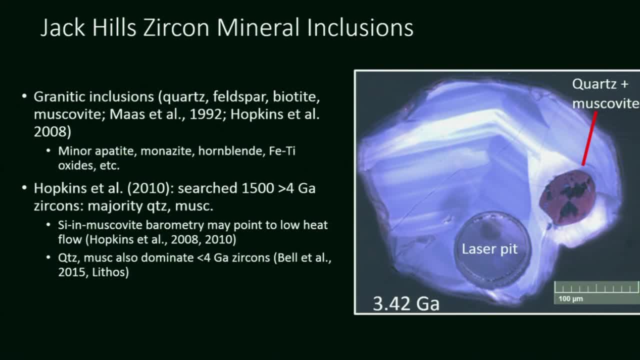 can tell you something about the pressure at which that muscovite crystallized and then, if you also have the temperature at which the zircon hosting it crystallized, from that titanium and zircon thermometer, you can start talking about the pressure and temperature conditions. Pressure- 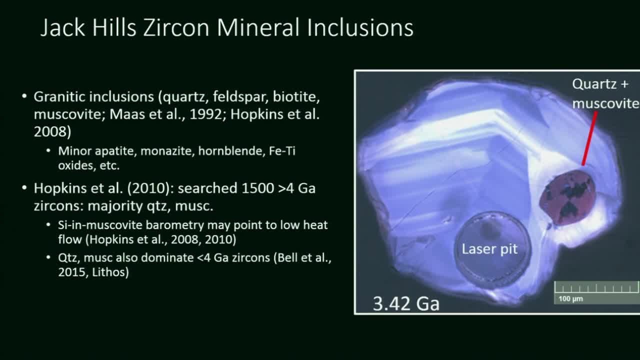 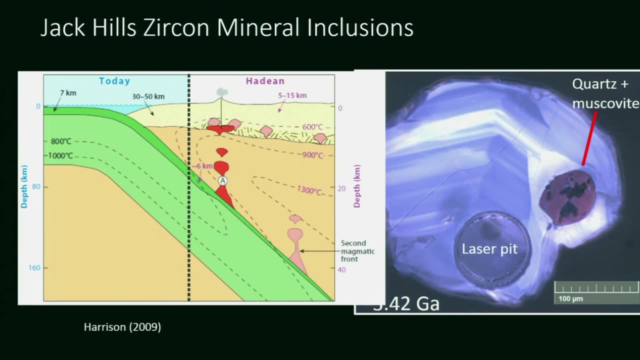 being relative to depth in the earth at which these samples formed, And then you can start making inferences about tectonic environments, And so one of the conclusions that Michelle came to is that a possible environment for many of the Jack Hill zircons might be a sort of 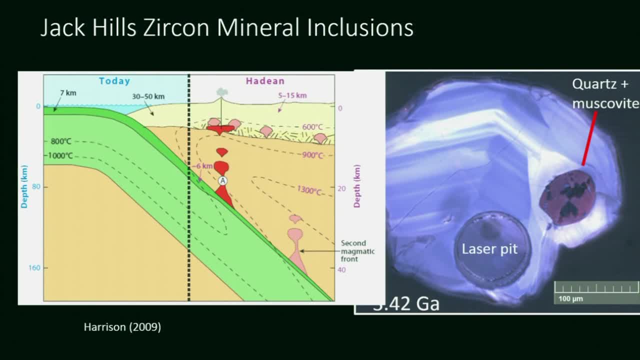 plate boundary under thrusting environment similar to modern day subduction zones, although it's not clear exactly how this would have manifested in the Hadean earth. But I would be very happy to answer more questions about this later, but what you can see overall, 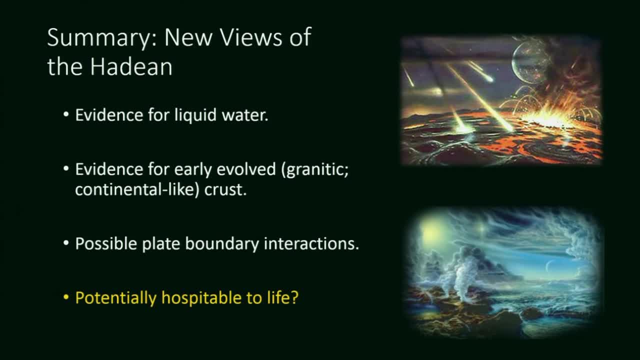 is that we have a very new view of the Hadean coming out of these zircons, from looking at the evidence. now that we have this geologic record for the Hadean, There's several lines of evidence that there was liquid water involved in their formation. 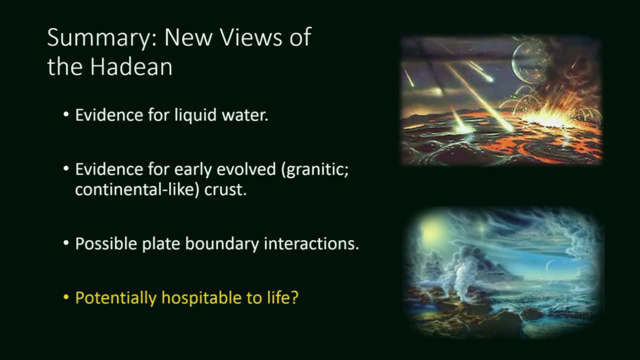 There's evidence for early evolved granitic looking crust. It's hard to say how much it was if there were like full continents or not, but these do appear to derive from a granitic type evolved crust. There's the potential for plate boundary interactions during the Hadean. 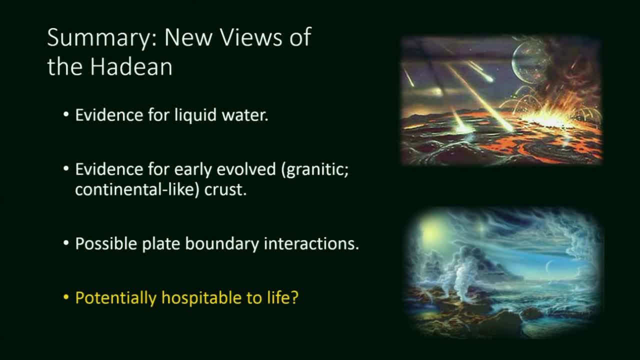 And so we start to look at a early earth that was a bit more like this than like this. And so if we have these more clement conditions happening early on, we have the oxygen isotope evidence as early as 4.3 billion years- we can start to ask. 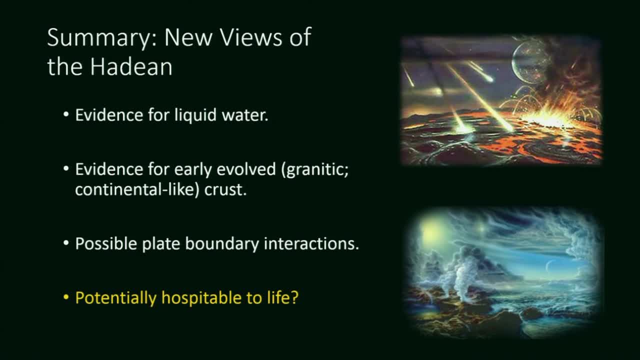 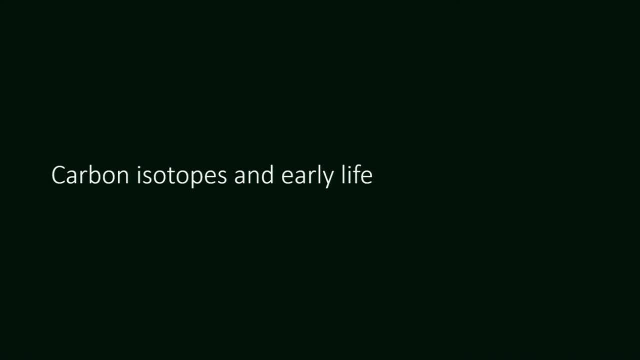 was this very early earth hospitable to life? So, first off, how are we going to look for evidence of early life, especially if we don't have a rock record in which we could find fossils? Well, I mentioned that we have carbon isotopic evidence from 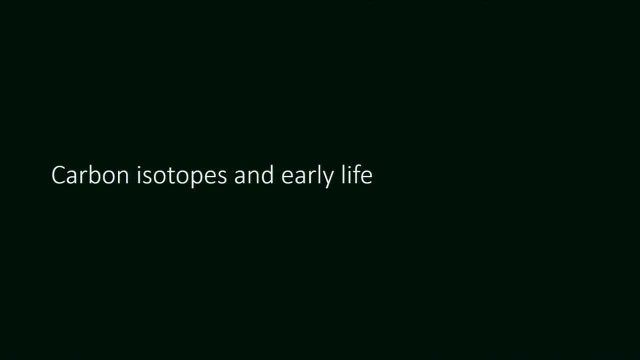 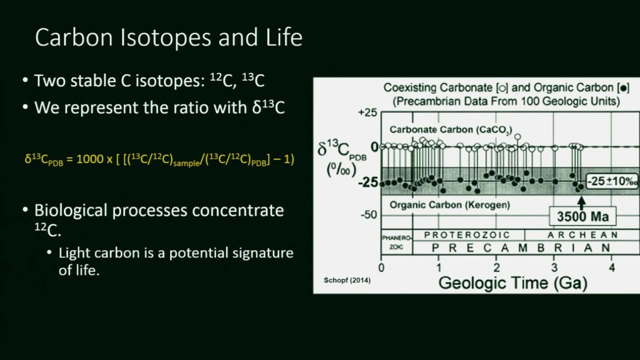 3.8 billion years. that suggests that there may have been life that early. So let's talk more about what this means. So carbon has two stable isotopes: carbon 12 and carbon 13.. And we're going to present this much like we did. 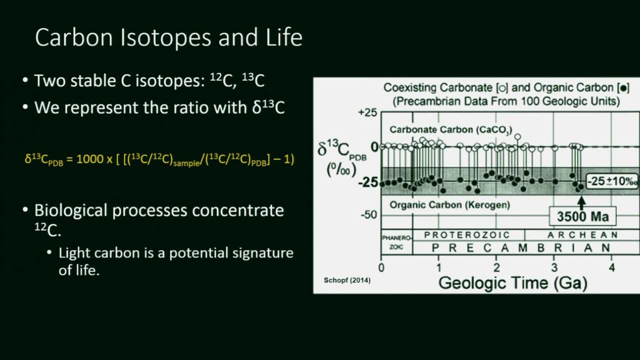 the oxygen isotope results. So we have this quantity, delta C13.. And so carbon 12 is the most common isotope of carbon, And the important point here is that biological processes tend to concentrate carbon 12.. Such that biological materials tend to 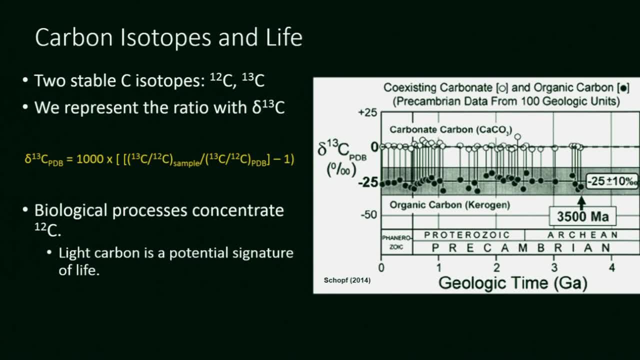 be very rich in carbon 12 relative to carbon 13.. And the offset in inorganic carbon versus biogenic carbon has really held steady over much of geologic time, for which we can see a fossil record. So this is a compilation put together by Bill Schaaf. 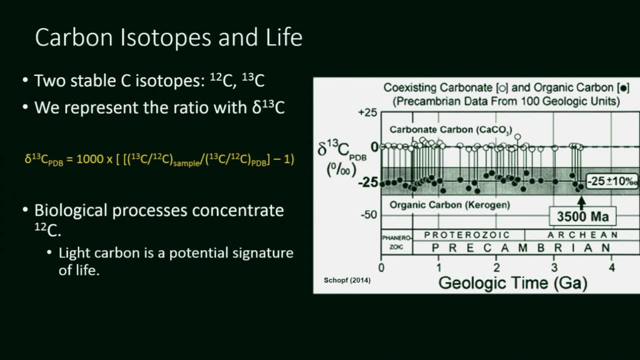 This is delta C13 versus age. We see the geologic record going back as far as we have fossils to nearly 3.5 billion years ago, the earliest microfossils, And what you're seeing? we have inorganic carbon that is here shown by: 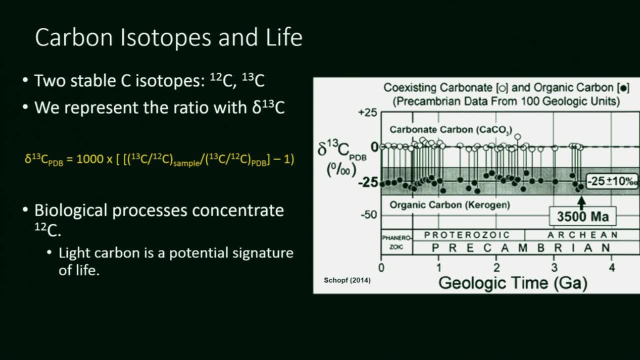 carbonate, which is averaging around 0 on this delta C13 scale. Again, delta C13, that's in parts, per thousand or per mil. So this is a 2.5% offset, or I'm going to be talking in per mil. so 25. 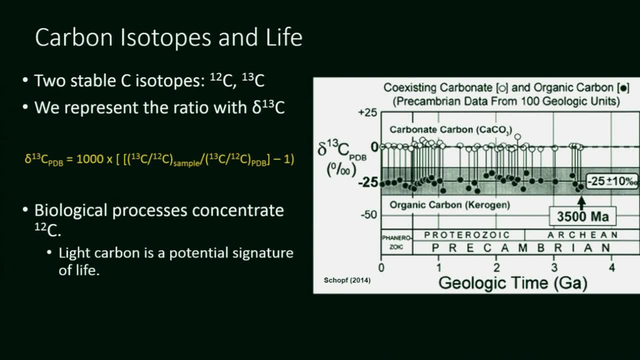 per mil And there's a relatively steady- although there are some excursions at various points in geologic time- offset of minus 25 per mil on average for these biologic carbon shown here by kerogens, And so we're seeing this very. 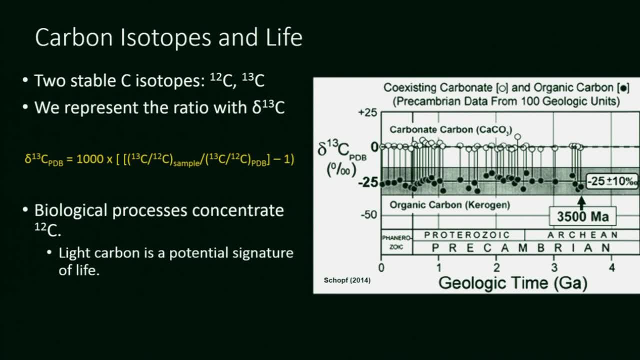 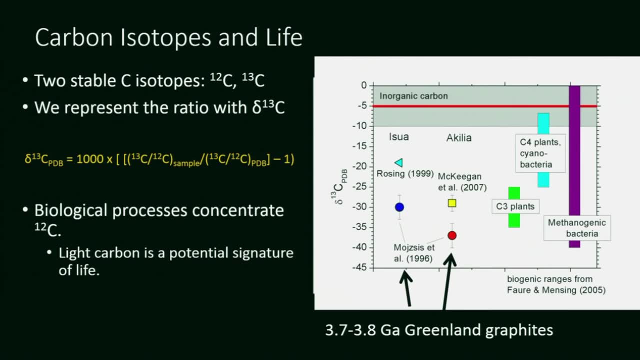 steadily throughout geologic time. So what happened at Greenland? What was found at Greenland? at 3.8 billion years, that tells us that we might see life there. Let's see. here we are Alright. so in Greenland, in several localities, 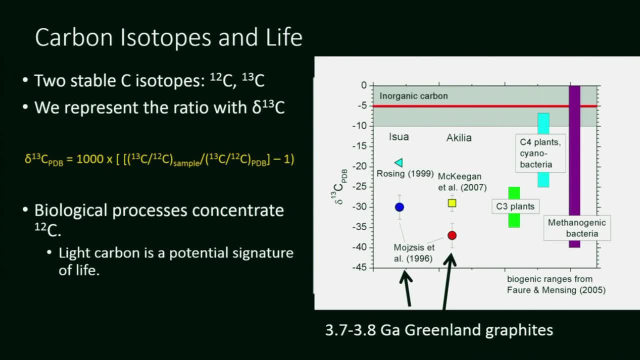 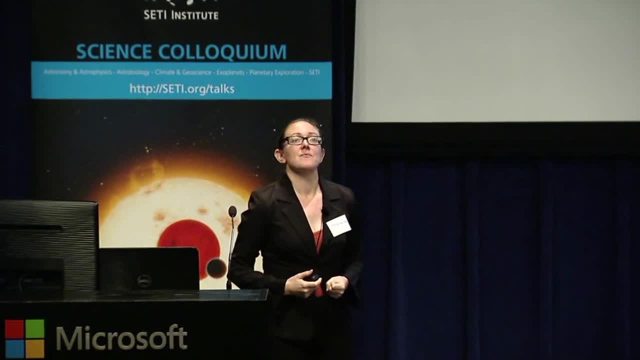 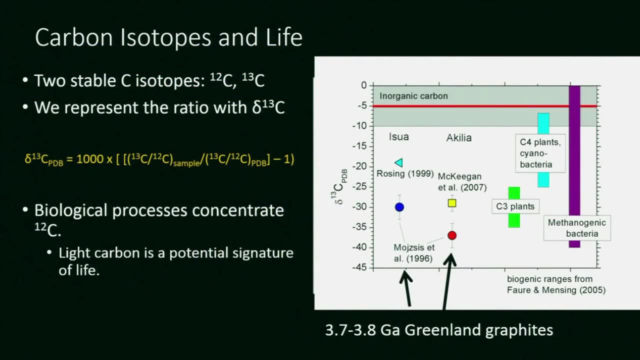 there are a series of marine metasediments and they contain graphite Graphite encased within other mineral grains, in this case a mineral called apatite, And these were studied in a series of studies, starting with Moise Chadel in 1996, and. 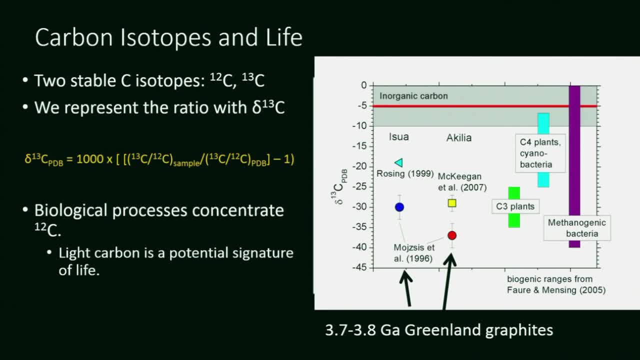 found to have very light isotopic signatures. So again we have a delta C13 and we're dimensionless here on the x-axis. What I'm showing you here is sort of the range of inorganic carbon you might get out of the Earth's mantle. 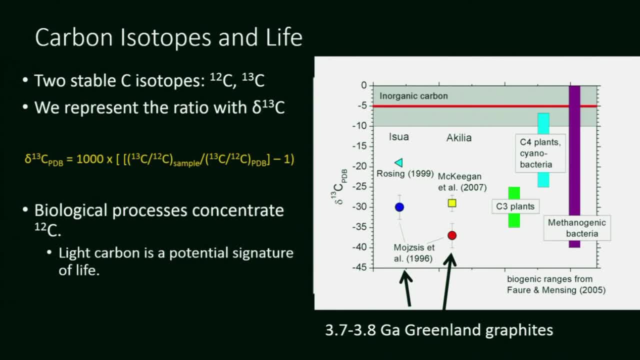 and the range in delta C13 from various metabolisms that you might find today, And so the very light delta C13 seen in many of these graphites from Greenland from 3.8 to 3.7 billion year old rocks was taken, as is interpreted. 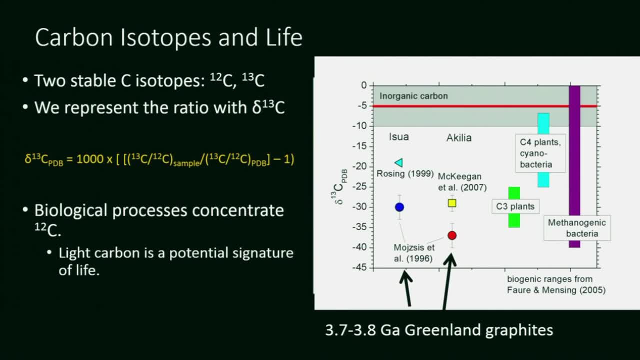 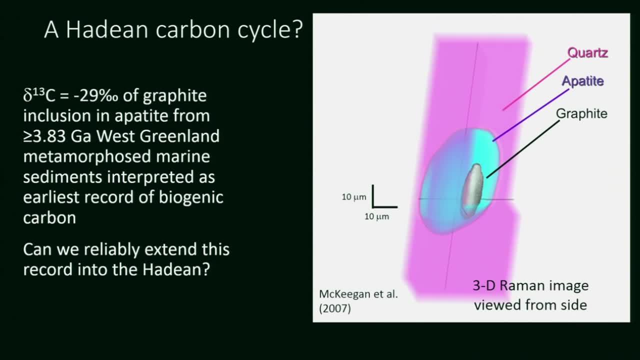 as evidence that there may have been life that early. Let's look more at some of these samples. So this is a follow up study by Kevin McKeegan from several years ago, and what we're looking here is a 3D Raman image. We've got a graphite. 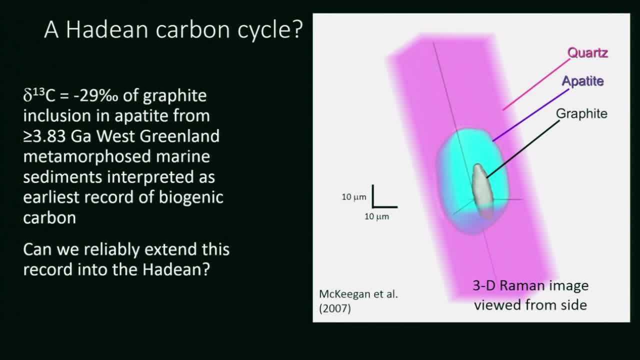 grain. it's encased within a larger apatite grain. We've got a 10 micron scale bar here And this is encased within a larger quartz inside these metasediments, And so the idea is you have the graphite. that's been. 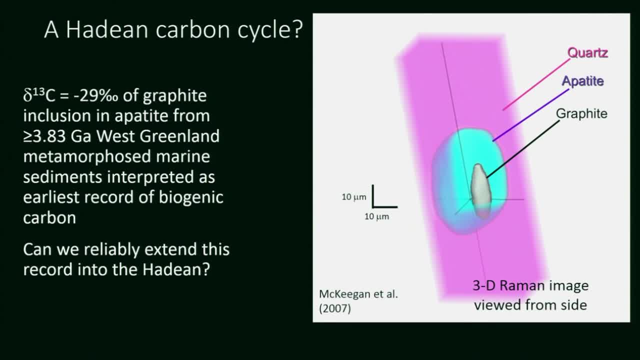 entrapped here and encased through geologic time, bearing this very light carbon isotopic signature. And now the problem with getting a definite age determination here. So these metasediments were dated by their by being cross cut by igneous rocks in which 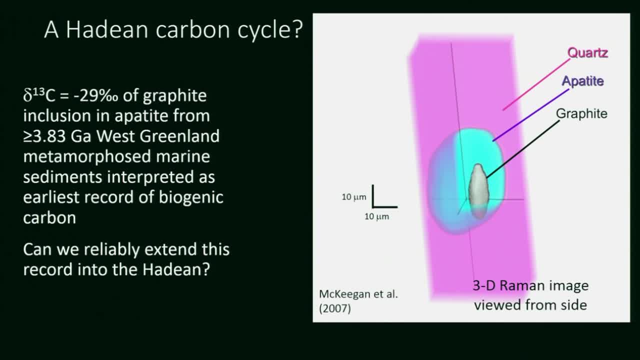 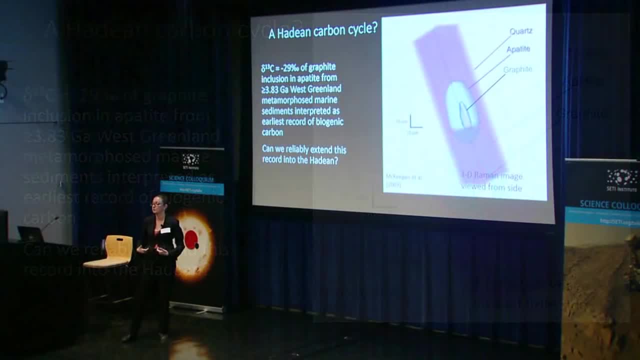 you could get a definite age. So we don't have a definite age determination. The graphite itself tends to not hold on to its uranium lead system very well. It tends to be reset by later reheating. So we couldn't get a direct age on the. 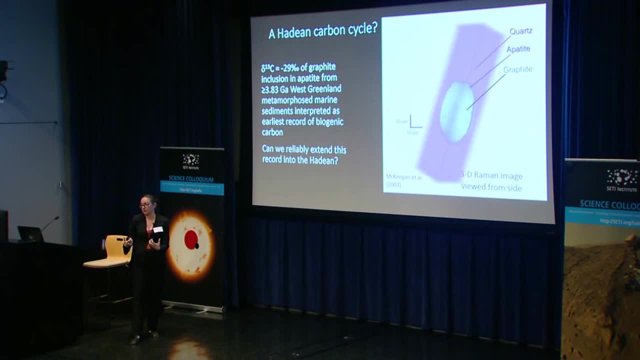 apatite that hosted the graphite. However, if we have the Jack Hill zircons, we have zircon, which is a great geochronometer. It holds steady over many billions of years And there are internal checks on the uranium. 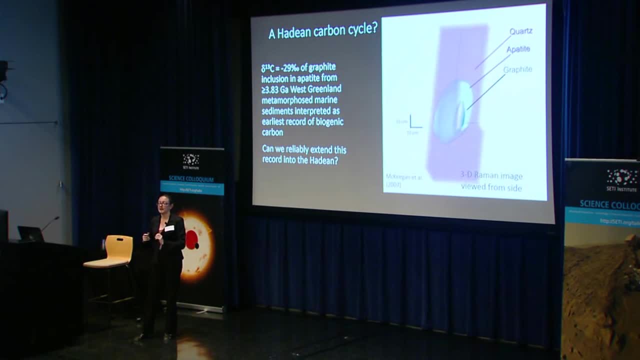 lead system to see if it has been disturbed. And so if we can find a graphite encased within these zircons, then we reliably extend this carbon isotopic record into the Hadean, beyond, where we even have a whole rock record. So there, 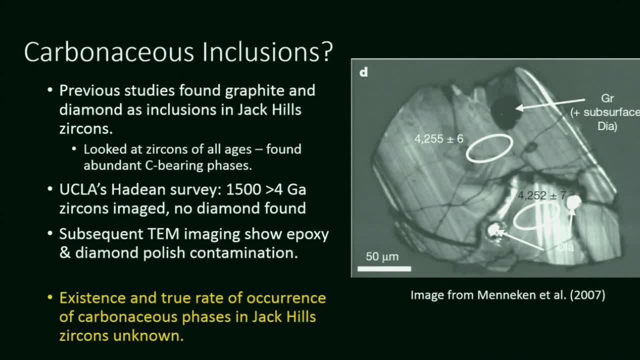 has been a long and a little bit sordid history of looking at carbonaceous inclusions in the Jack Hill zircons. So two studies came out in the mid-2000s that were quite exciting at the time, claiming to have found abundant graphite and also. 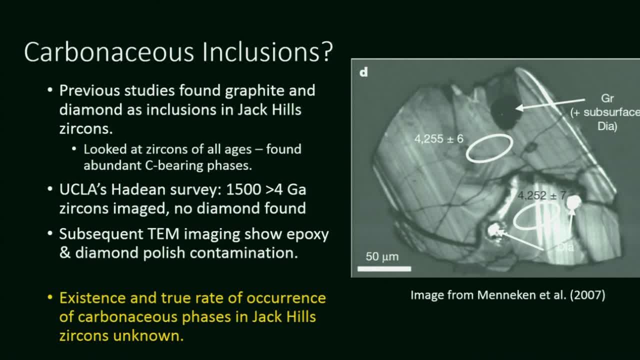 diamond in the zircons. So this is an image from one of the studies. This is two diamonds and graphite that are reported here. So what the study did? they looked at zircons of all ages, from the Jack Hills I believe. they looked at about a thousand. 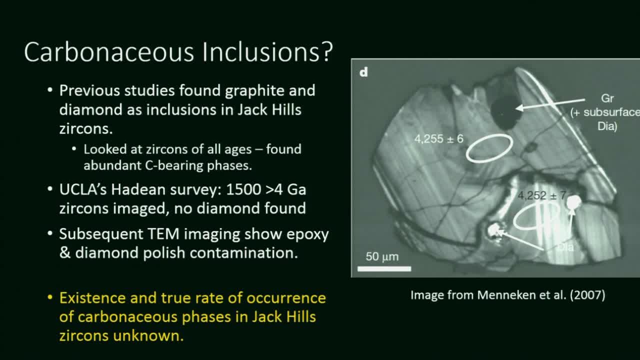 of them and reported a relatively abundant carbon or carbonaceous phases. Now diamond is surprising for a number of reasons in the zircons. So first UCLA- we had been looking through these Hadean zircons, looked at about 1,500 of them. 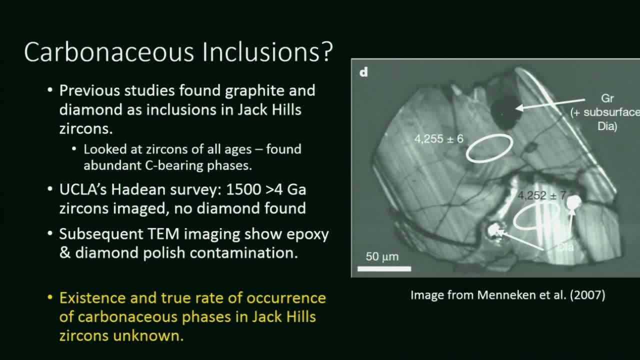 specifically those older than 4 billion years, and Michelle Hopkins had not found any diamond in her survey, And the ones that were reported in this study were largely sort of on the surface things that you might find with a scanning electron microscope, much like Michelle's study. 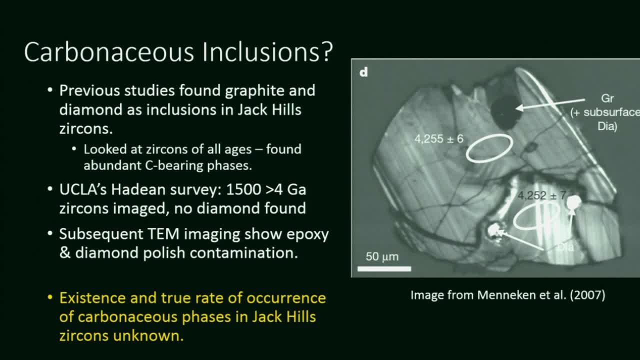 And now another interesting thing is that- remember there's only around 3-5% of the zircons in this Jack Hills population are older than 4 billion years, so there could have only been 30-50 of the Hadean. 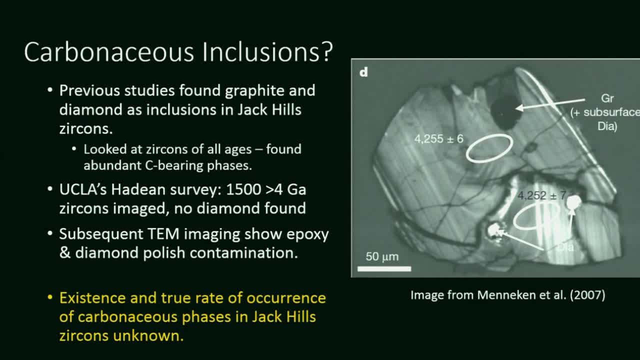 zircons in this study, which is interesting, that the very abundant graphite and diamond was found in them. Now, another thing that's interesting is that diamond is a very high pressure phase. We find it coming out of Earth's mantle, and so this sort of clashes. 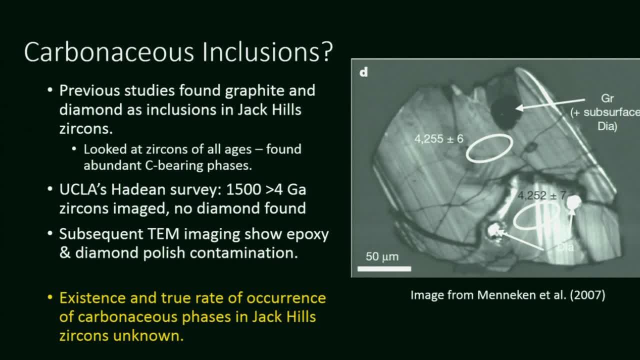 with the other pieces of evidence coming from the zircons, the idea that it would have been a relatively low pressure from the muscovite inclusions, the relatively low temperatures, the sort of granitic looking environment which you know, that's. 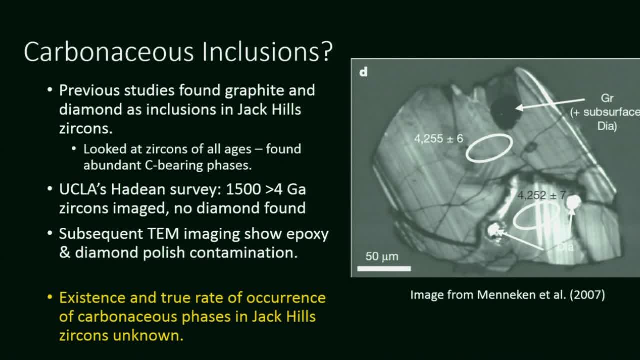 okay. if this is indeed what we're seeing in the zircons, we need to be able to explain it Now. as it turned out, subsequent TEM imaging of these inclusions turned out that they were contamination. So what I'm showing you here is: 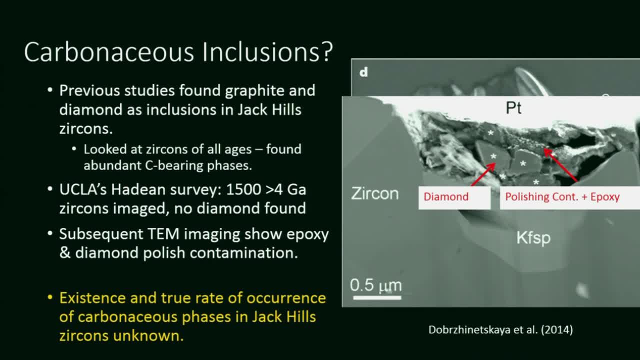 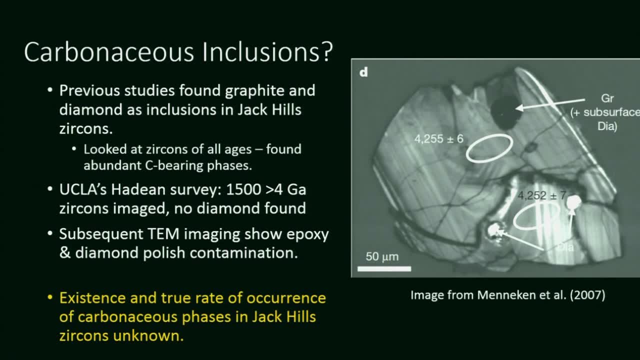 an image from this excellent study that came out last year, two years ago now, and what we're seeing here? we're seeing a cross-section so previously. so let's say, we're looking at one of these inclusions. this is a plan view. now we're looking in cross-section. 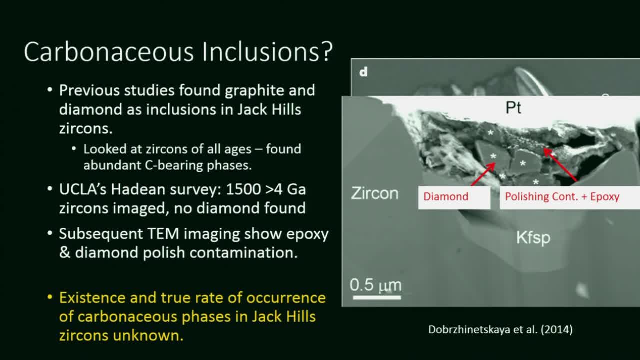 this has been sliced out looking at on a TEM. we have zircon here and we have- this is a potassium feldspar inclusion- in a little hole that's been dug into the inclusion, and into this hole had been stuffed diamond. so 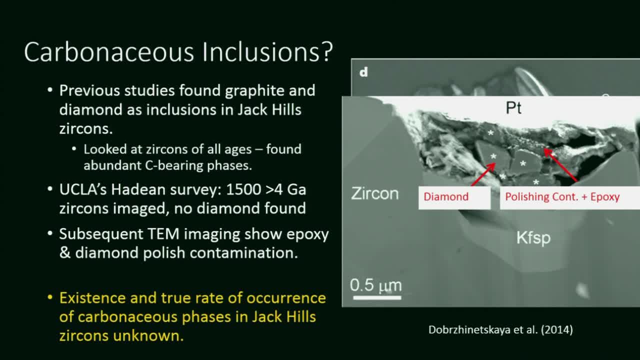 these particular samples underwent a polishing step using a diamond compound. so diamond polishing, which is often done for a lot of zircon studies, because it can give you a very nice polish, and there was also bits of epoxy that ended up in there. 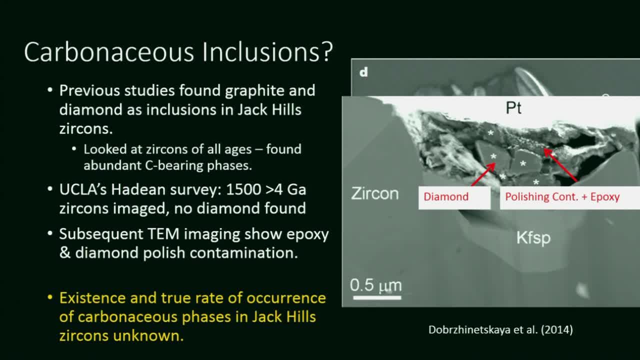 so these zircons are mounted in epoxy generally and which became fried in the laser beam that was used to do Raman spectroscopy and ended up giving the graphite signal. So unfortunately, these ended up being contamination. However, this leaves the existence indeed. 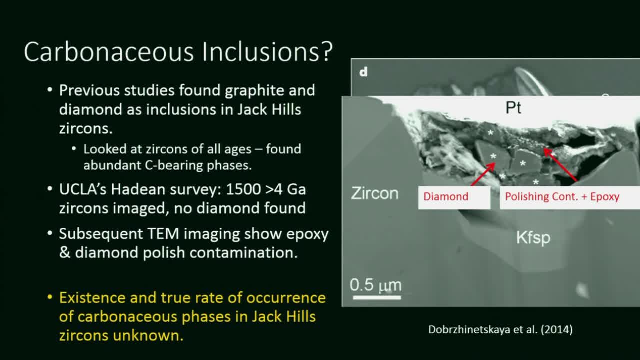 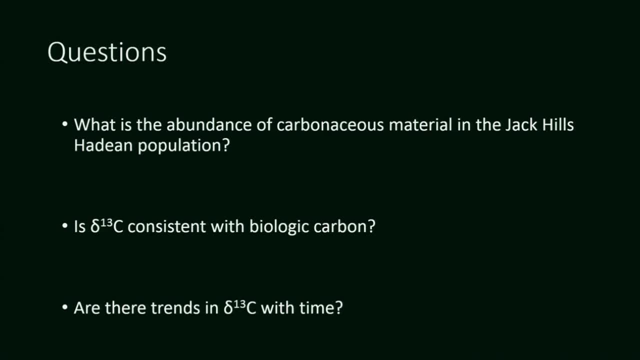 and true rate of occurrence, if they do exist, of carbonaceous phases in the Jack Hills zircons unknown, and so this leads to several questions that we wanted to tackle in our study. So what is the abundance of carbonaceous material in the Jack Hills? 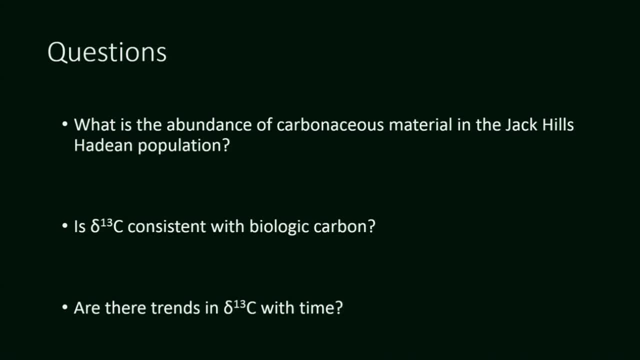 Hadean zircons. Is it there? Is it there at a relatively high rate, as these studies suggested, or do we find it very rarely or not at all? Second, is its delta C-13 consistent with biologic carbon or potentially with other processes? 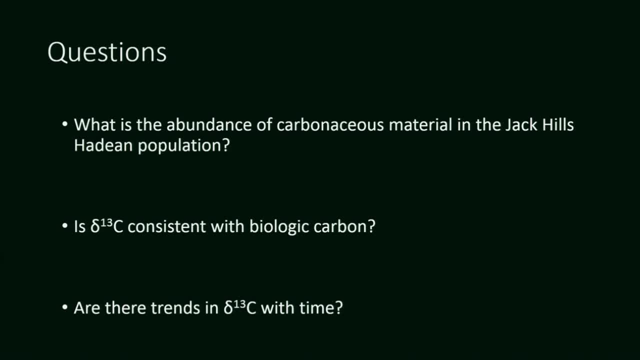 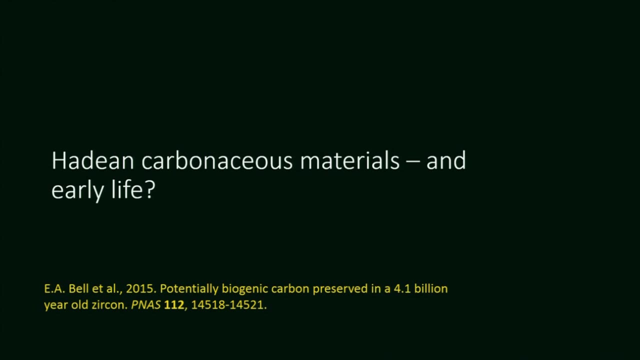 that might form a graphite inclusion in a zircon. And lastly, if we can find multiple such inclusions, do we see trends in delta C-13 with time that could tell us something about the Hadean carbon cycle? So we published this just last year. 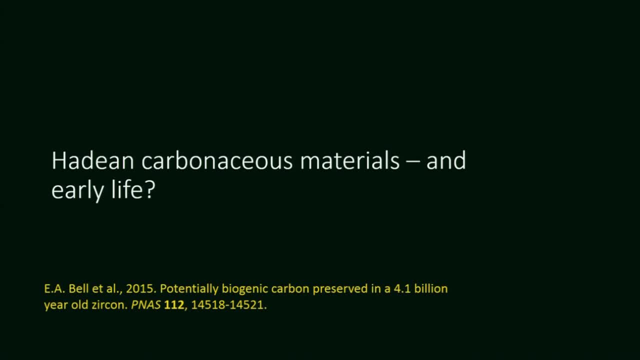 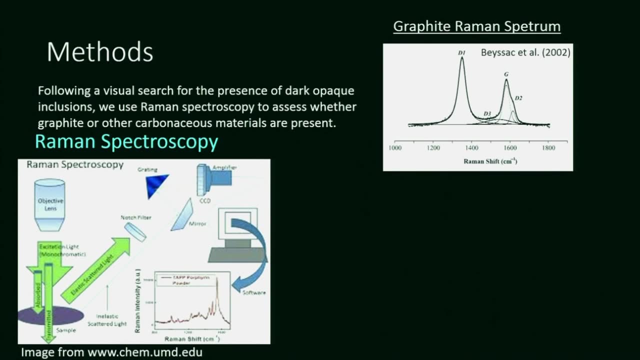 in PNAS looking at Hadean carbonaceous materials, And I'm going to start off with the methodology we used to go through our study. So at UCLA we have several thousand Hadean zircons from Jack Hills archives. So this has been a 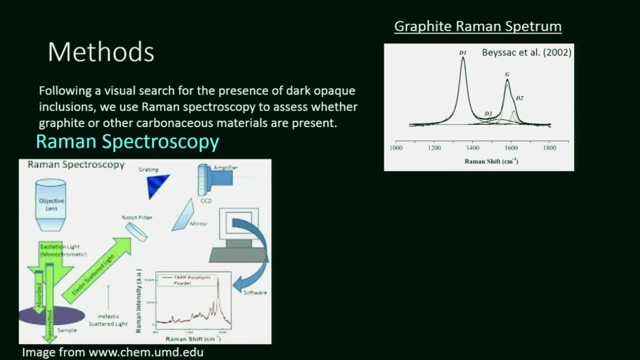 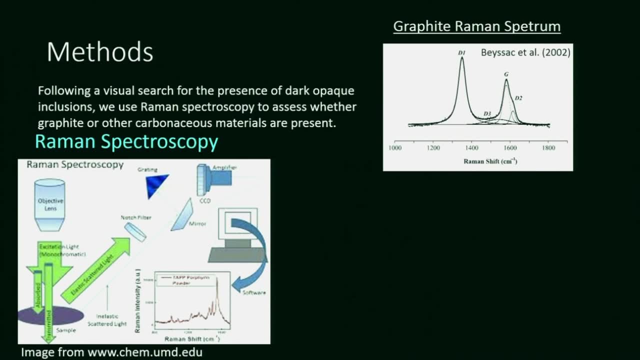 massive effort by my supervisor, Mark Harrison, and several scientists at the Australian National University. over the past decade or so They've gone through 200,000 of these zircons from Jack Hills at ANU And they've dated them and found. 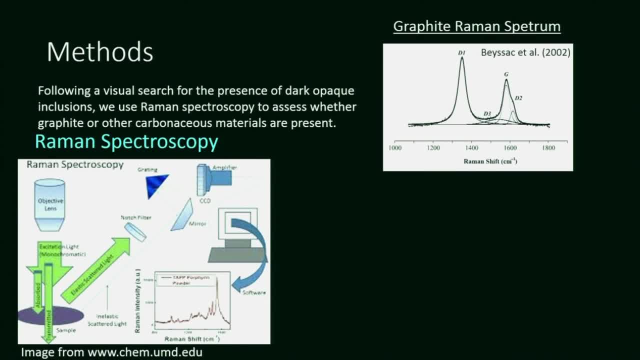 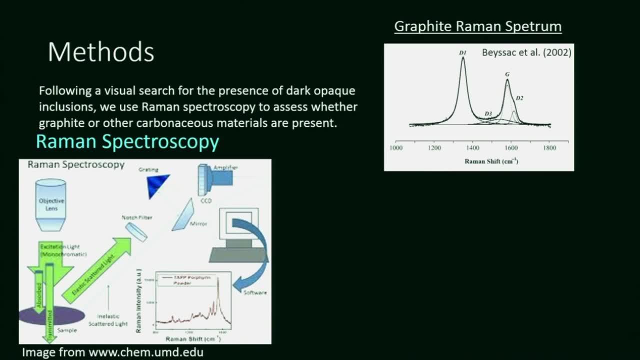 the ones that are older than 3.8 billion years, which again end up being about 5% of the population. So we have a set of about 300 mounts at UCLA with sort of marked out Hadean zircons in them. 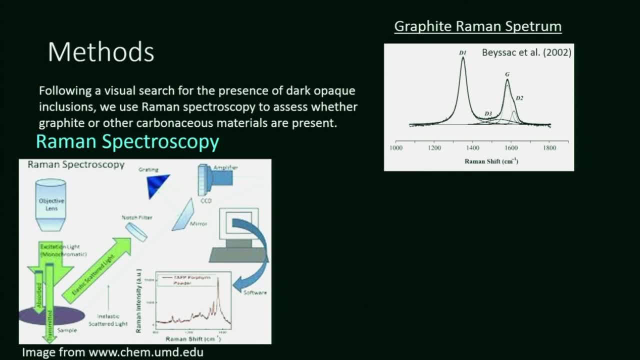 So we've systematically gone through and done a visual search with transmitted light microscopy to see if we could find dark specks in the zircons that might potentially be graphite. And once we find these candidate dark specks we then go to Raman spectroscopy. 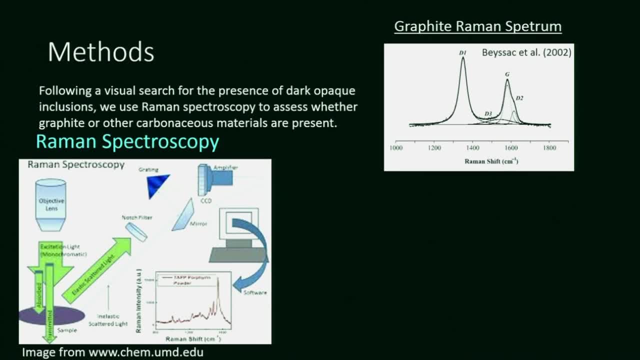 to see if it is indeed graphite. So briefly, the way Raman spectroscopy works. I am not an expert in it- I think some people here might be- But for those who are not familiar with it, we are going to shine. 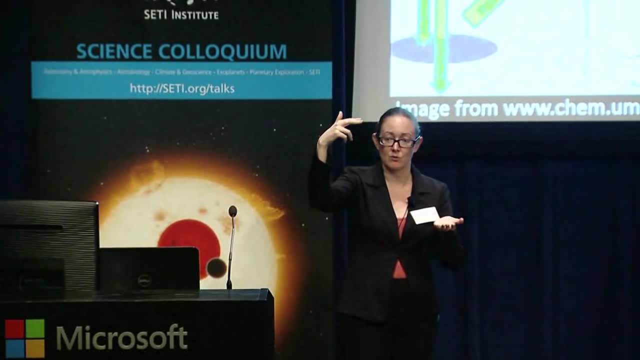 a laser beam onto a sample. So laser beam, coherent light, it's all one wavelength. And then when this light gets scattered back, it will have characteristic shifts in the wavelength that are characteristic to different minerals. And so, for instance, I'm showing 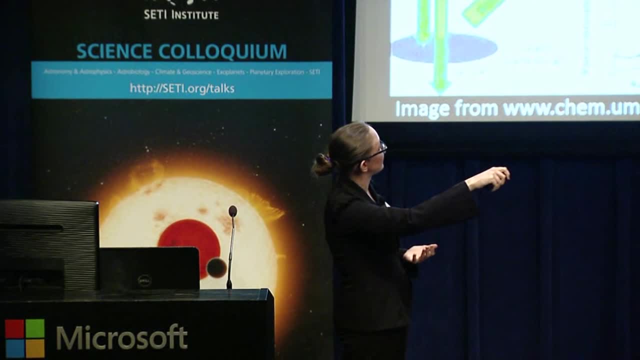 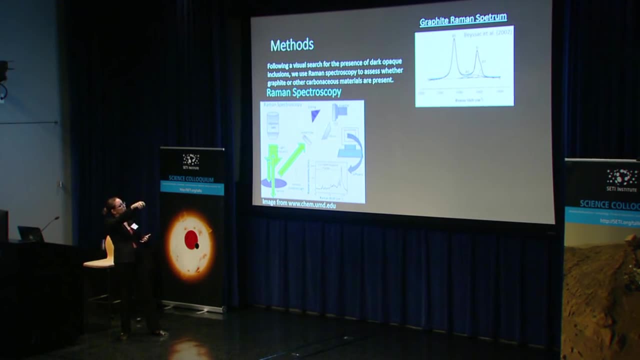 you the graphite Raman spectrum. here for probably the most diagnostic portion of it, There are these two main peaks, the G and D1 bands, in about 1600 and 1400 wave numbers. What's important is that here I'm showing you one of our samples where we have 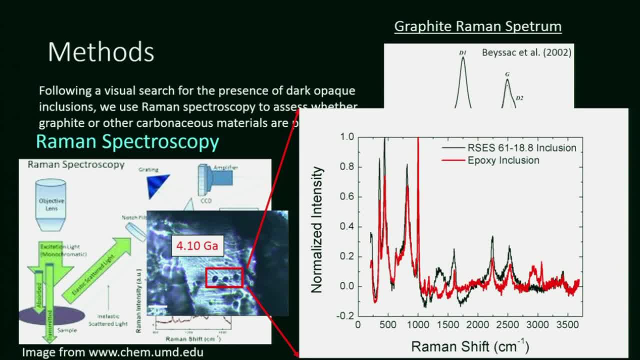 in fact, two graphite inclusions underneath the surface. here This is a transmitted light image of a 4.1 billion year old zircon, And in the black line here we are showing our graphite inclusion. So these are our G and D bands. 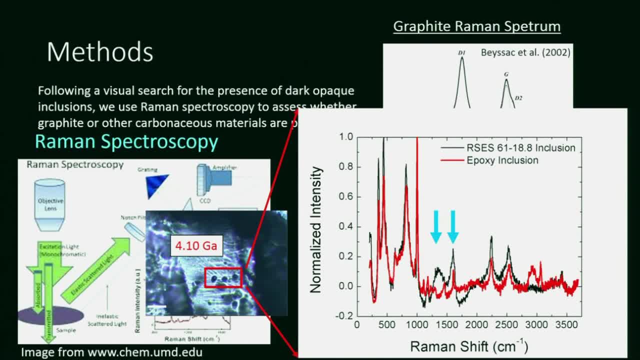 that you can see here And, for comparison, in the red we can see the difference between these two materials. So we are not graphitizing our epoxy to the extent that we could confuse them. So here's a third region that's very useful here. 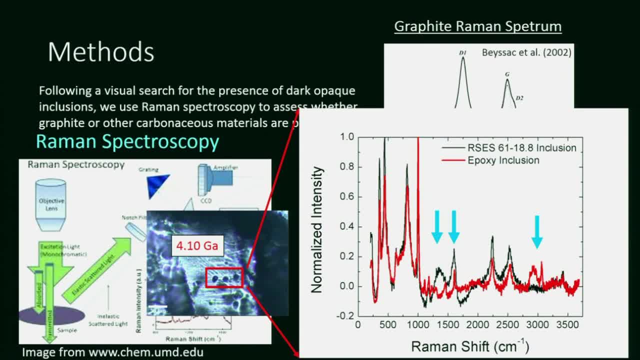 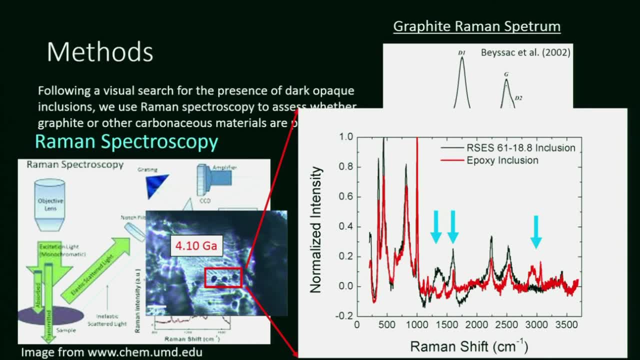 So these bands tend to be characteristic of CH stretching in hydrocarbon molecules. So we can see that in the epoxy, which still has quite a bit of hydrogen hanging around in its structure, but we're not seeing it in our graphite inclusion. 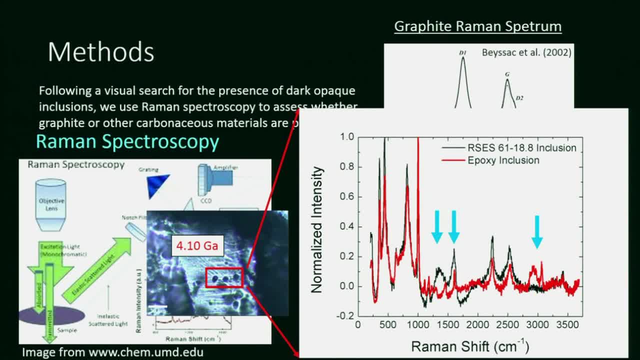 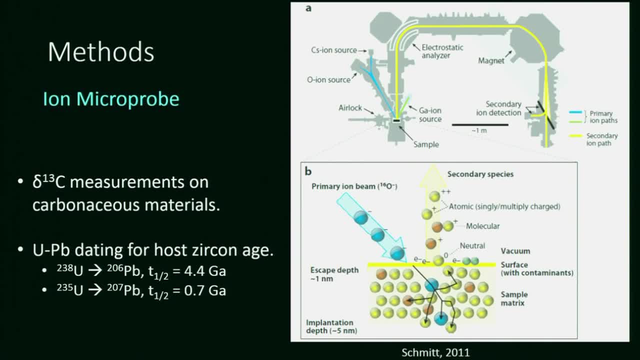 So we've identified some graphite in a 4.1 billion year old zircon. What are we going to do now? So we for our isotopic measurements. we measured the carbon isotopes using the ion microprobe. at UCLA We have a Kameka. 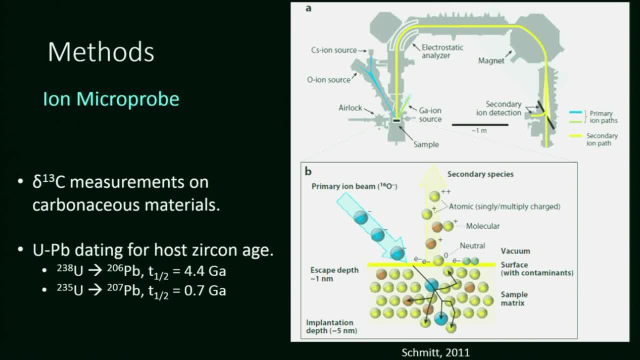 IMS 1270, which is very nicely diagrammed here in this review paper by Axel Schmidt. So the way secondary ion microscopy works is: you have a solid sample surface that has been polished, nice and flat. You have a primary beam of ions come in. 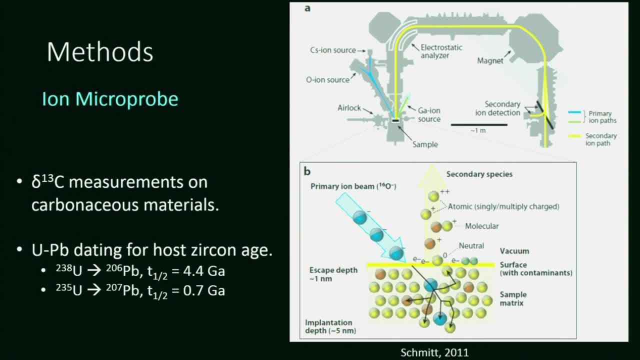 In this case it's showing a primary oxygen beam, but we used a cesium beam for this study because the carbon tends to ionize better in that manner. Then you have secondary ions come off and are drawn into the mass spectrometer for isotopic. 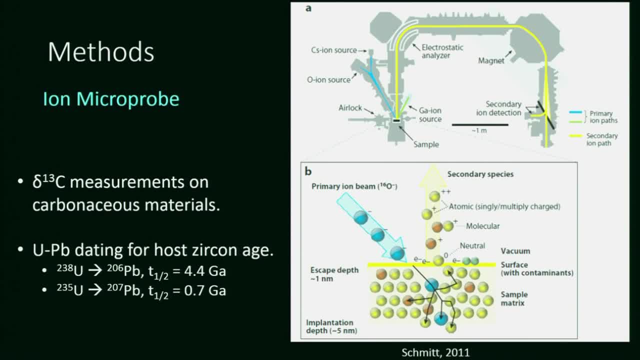 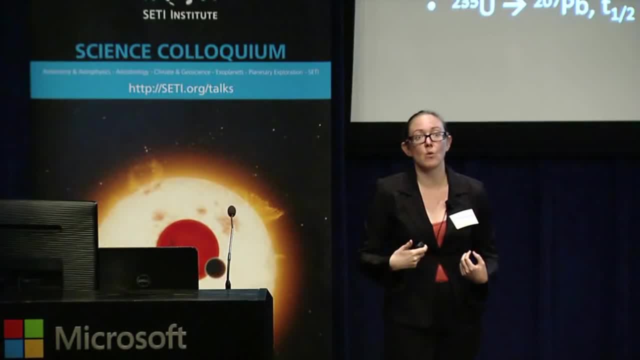 analysis. In a previous phase of this study at ANU I mentioned the very large 200,000 grain survey they've been doing. So this host zircon was uranium lead dated to get that 4.1 billion year old age at ANU. 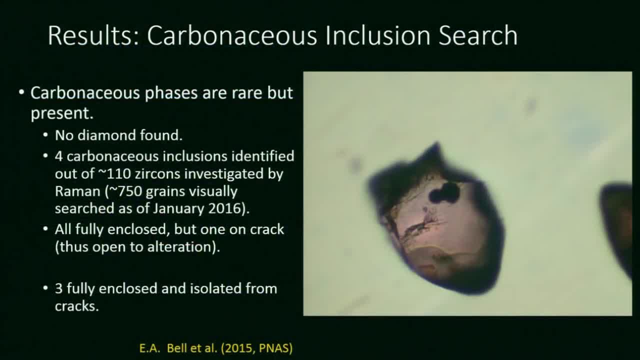 using a different instrument. So how many carbonaceous inclusions did we find? I've shown you that one zircon. So we ended up finding they are rare, but they are present In around less than 1% of the zircons we have visually searched. 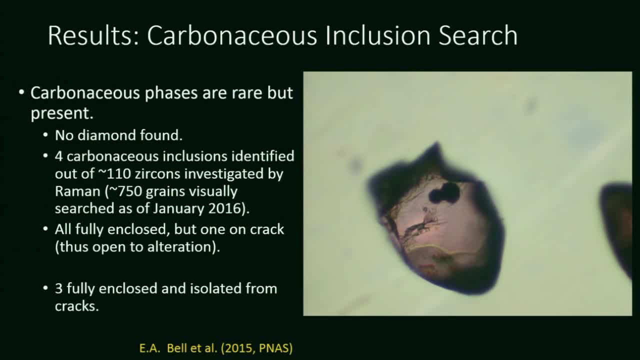 we found this material. We have not found any diamond so far, but our search protocol is tending to be leaning more towards graphite, So this is sort of a blind spot. if we want to say there's no diamond, We need to sort of work. 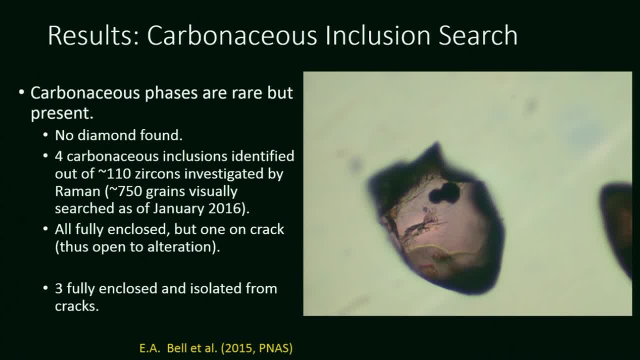 around to a different sort of methodology, But we can say that we found four carbonaceous inclusions that look like graphite based on their Raman spectroscopy. Now, all four of these carbonaceous inclusions, they're not found at the surface of the grain, They're found beneath. 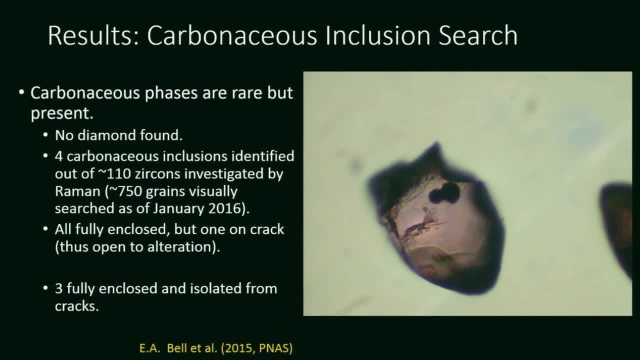 the polished surface, which excludes one possible avenue for contamination, And so three of these are fully enclosed by the zircon and also away from cracked regions. Now one of them is on a crack, and so we're going to exclude it from further consideration. 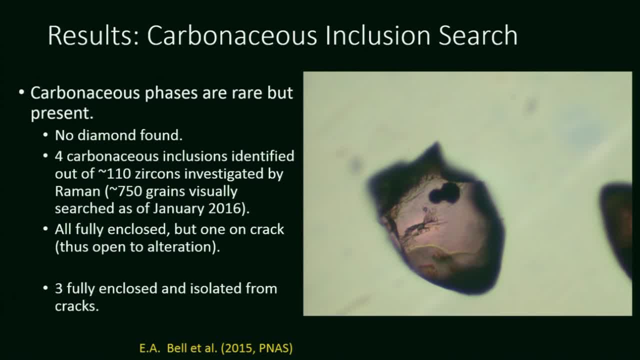 in this particular talk Because a crack, if it was open over geologic time, fluids could have gotten in there and contaminated and given us a different delta C-13 signature. that isn't telling us about the Hadean, So here's an example of a nice. 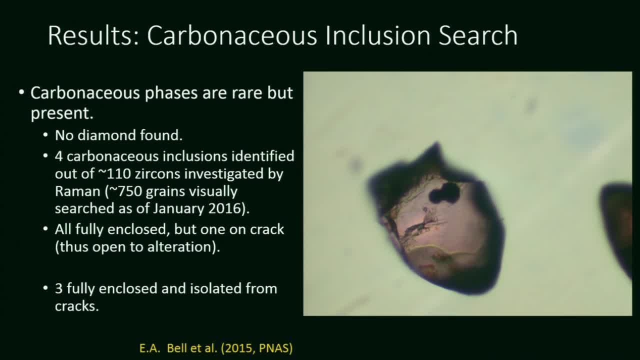 this is a graphite inclusion, as shown by Raman spectroscopy. We just found this one this past January in a new phase of Raman search. This is- unfortunately, this is an undated Jack Hill zircon, so we don't know if this is going to tell us about the Hadean. 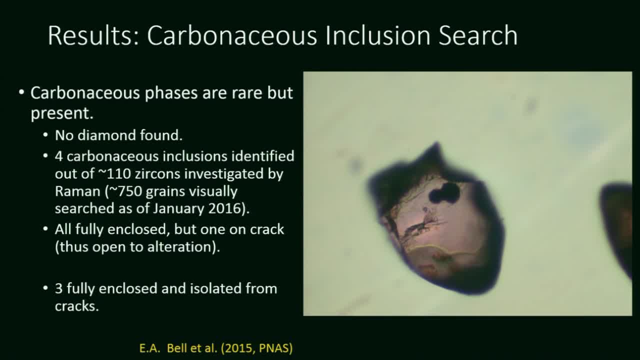 or about the Archean, but this will be a very exciting sample to look at. There's not a scale bar on here, but this is around 50 microns in this direction, so there's a fair amount of material there for an ion probe to look. 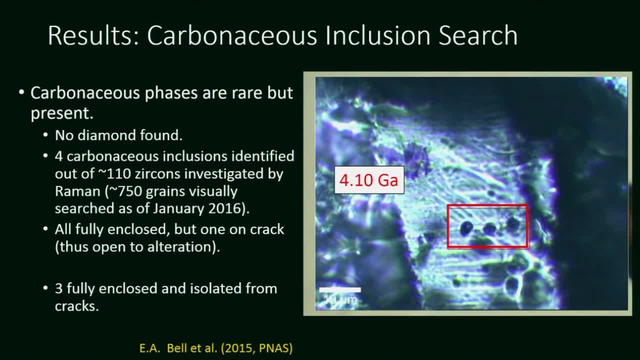 at- And this is sort of our star sample here- this 4.1 billion year old zircon with two graphite inclusions here. So I'm showing you this transmitted light image here, in which it does not look like there are any cracks, but 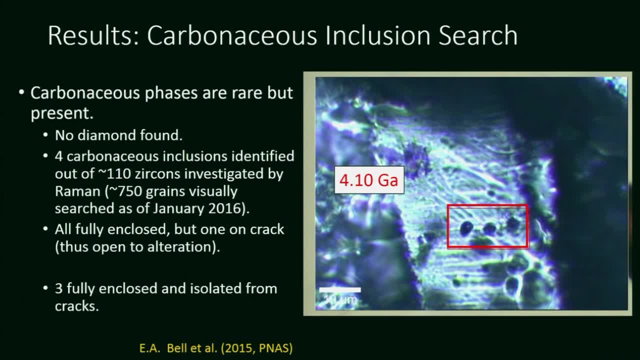 as I had mentioned before, cracks are going to be really dangerous for potentially bringing in fluids over geologic time, which could contaminate our signal. so we want to be extra sure of this. So fortunately we have collaborators at Stanford who work. 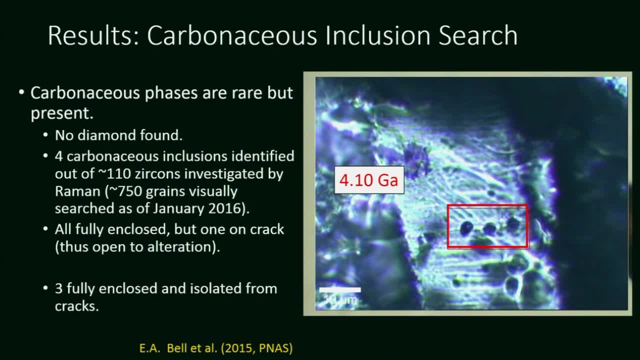 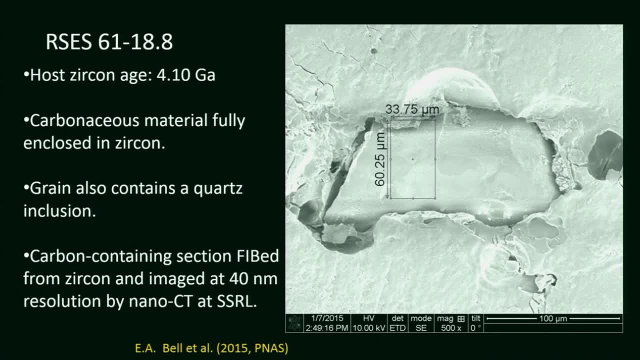 on the synchrotron at Stanford, regularly doing X-ray imaging at very high spatial resolution. So our co-author, Wendy Mao, generously allowed us to image our sample during some of her beam time last year, and what I'm showing you here this is a scanning electron microscope image. 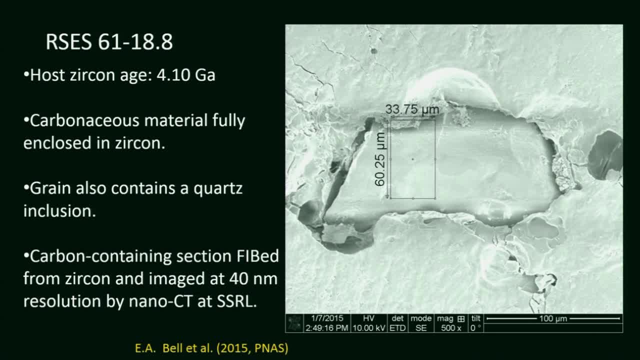 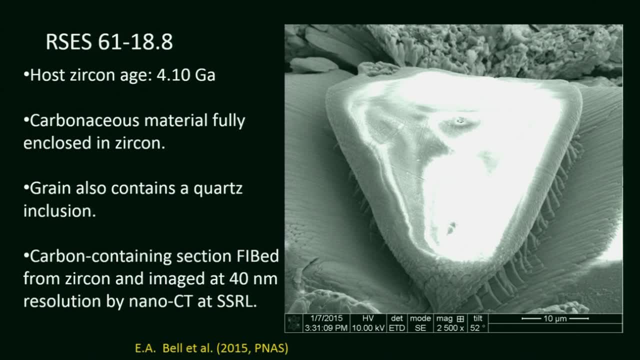 it's kind of fun to see how we milled this segment of zircon with the carbon out with a focused ion beam. we're looking from the top now. we're sort of looking from the side and you can see where the ion beam has come in. 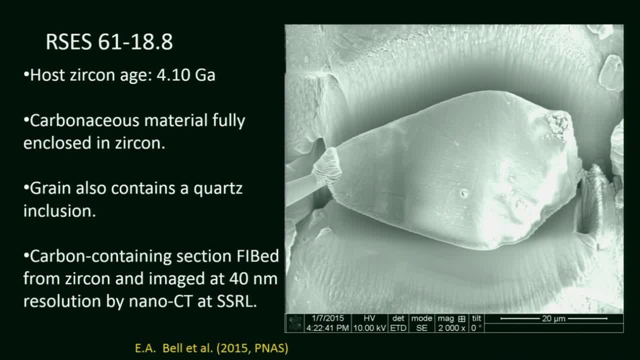 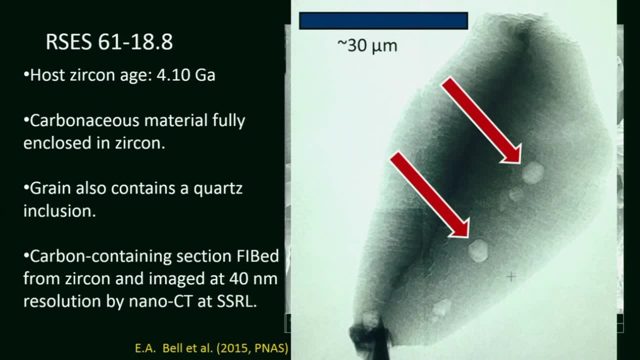 and milled out this section of zircon. now we're looking from the top again and a needle has been welded on here. we're going to lift this section out, and now this is a transmission X-ray image taken at the synchrotron. 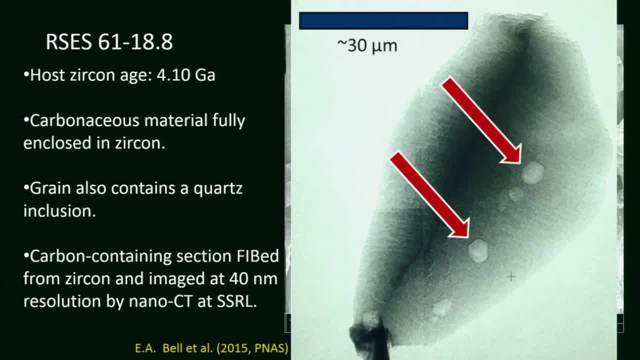 by Crystal Shi, who is Wendy's grad student, and what we're seeing. I'm pointing out the two graphite inclusions here. you can see several other inclusions also in this segment of zircon. we haven't definitively identified these yet and you can also see: 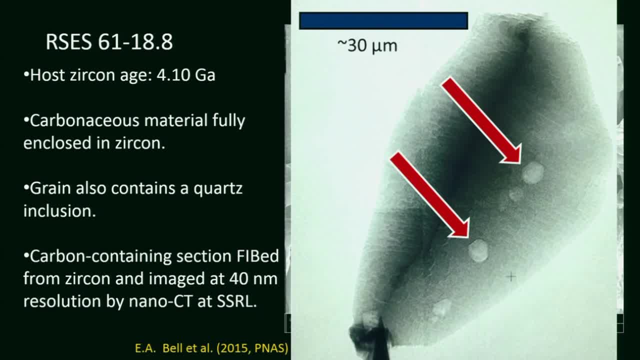 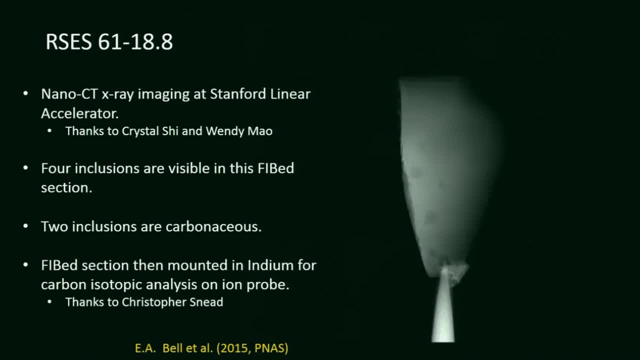 for reference. here at the bottom we've got the needle that was welded onto this segment of zircon. so because the needle was rotated to get X-ray images from many different angles, we are able to look at this in 3D. so we've got this movie going here. 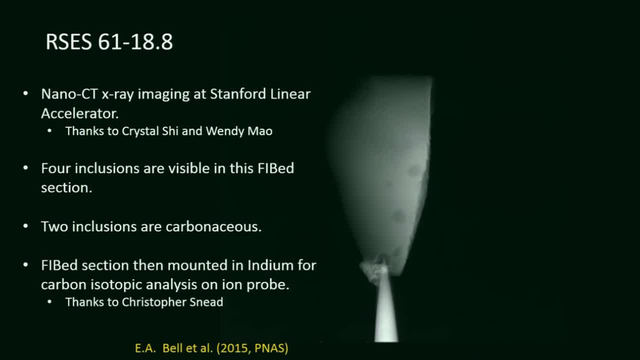 so we've got our two graphite inclusions here, but we've got, let's see, yeah, you can see, in this view it's very nice. you can see that these four inclusions are not coplanar, so it's not like a crack that came in and healed. 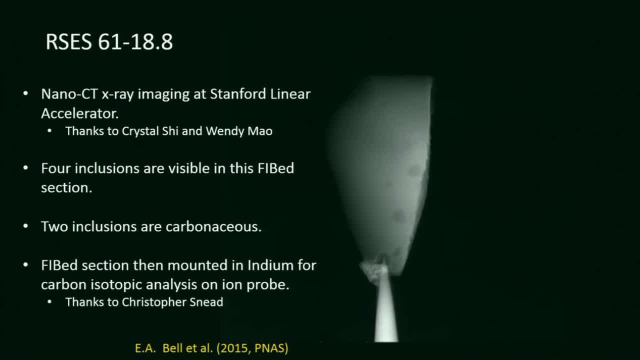 so, having identified these as not being coplanar, and seeing no cracks at this 40 nanometer spatial resolution technique, we then took this segment of our zircon. we mounted it in indium rather than epoxy to cut down on the danger of carbon contamination, and 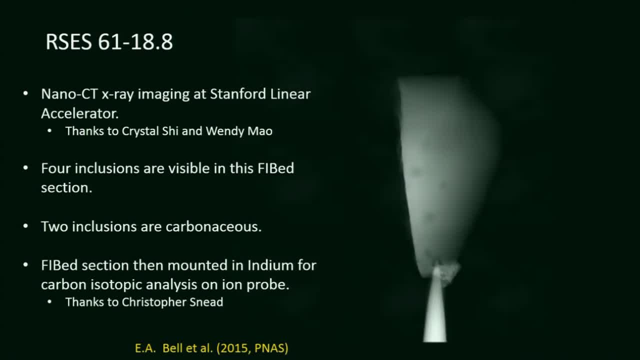 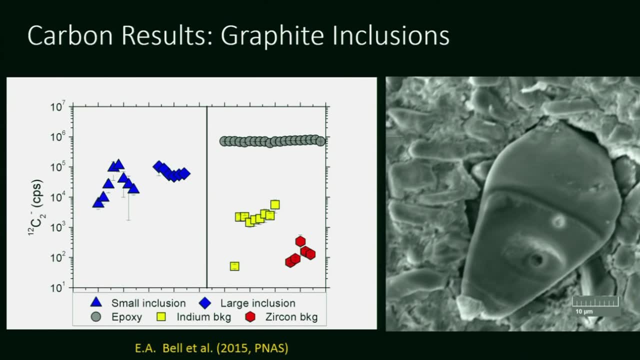 we went to the ion probe for carbon isotopic analysis and let's see, there we go alright. so what I'm showing you here. on the right, this is just an SEM image of our segment of zircon in its indium mounting medium, and on the right, I'm showing you some of 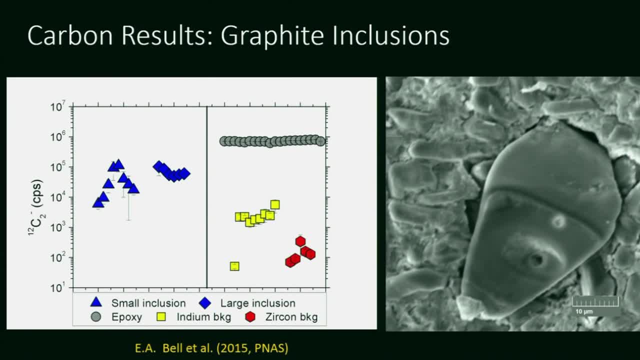 our results not in delta C-13, but actually in the intensity of the carbon, and then this is within these individual results. this is time on the X-axis. so what I'm showing you on the right here these are background measurements, both on the 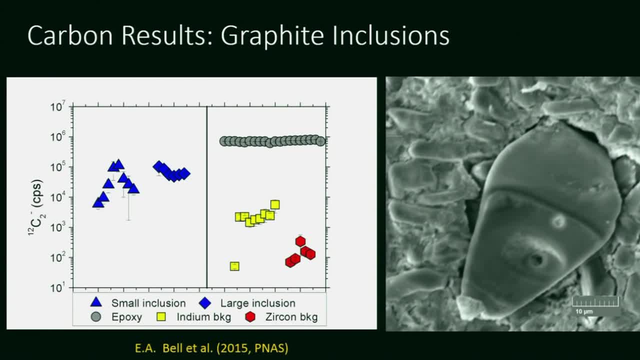 indium mounting medium and also on a clean segment of the zircon itself, showing that these are several orders of magnitude below what we're seeing within our graphite inclusions and, in particular you can see so we have a large segment of this zircon that is a little darker in this image. 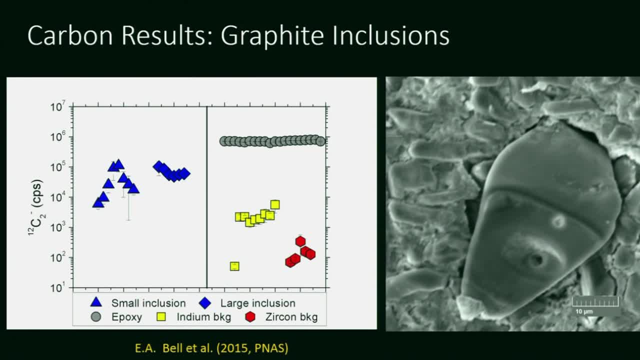 and what that is is. we took our ion beam- since we can move it over the surface of our zircon, just to clean it off, to just really really cut down on the danger of contamination, before we did our isotopic measurements. so you can see this. 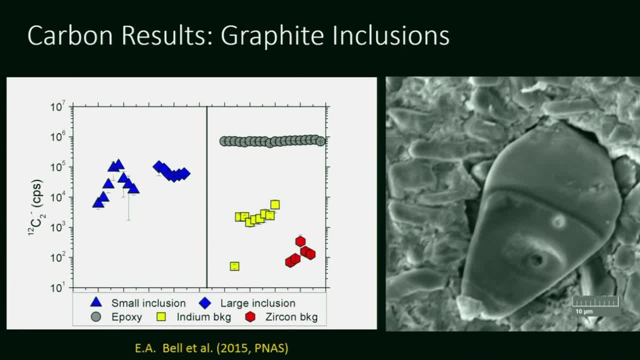 10 micron ion probe pit here and at the very bottom of it. you're starting to see this hole, which is our small inclusion, and the small inclusion is sort of fun. you can see we cut in one side of the zircon drilled into the middle. 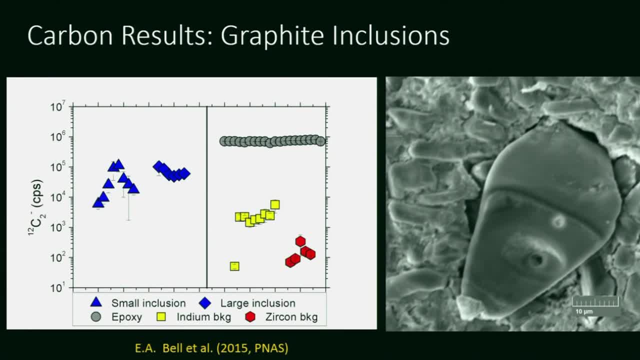 and then drilled out the other side, so you can really see that this was fully enclosed in the segment of zircon and we are for reference. this is our big inclusion that is just starting to be uncovered here, and so because it was okay, so here's a second view. 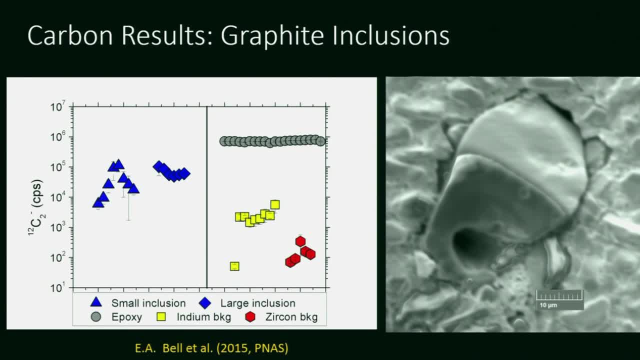 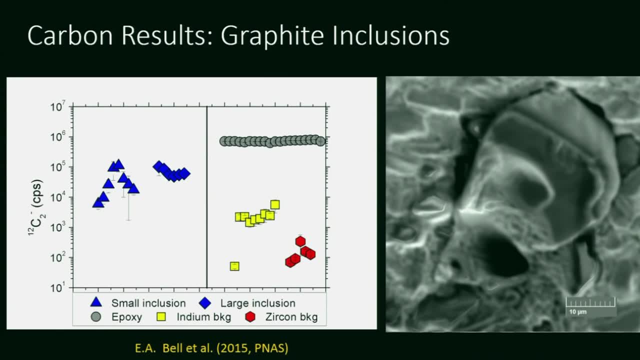 where there's our big inclusion still here and we have now blasted through our small inclusion. now here is a third view where we have- we've moved this pre-cleaning surface much further up the zircon. we have now blasted through our large inclusion. we're not seeing a similar sort of. 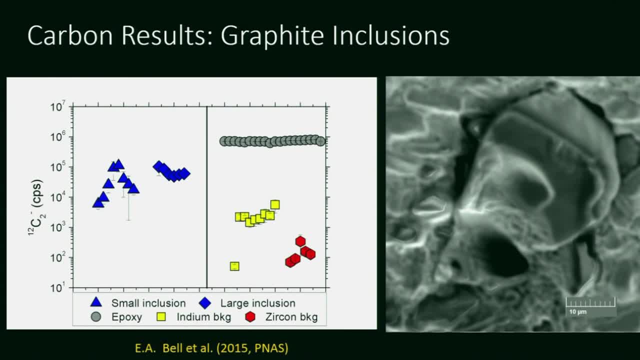 up and down movement with our large inclusion, probably because it had been somewhat uncovered by this pre-cleaning step beforehand. so we see, we are able to measure our graphite at much nicer than our background. our background is not going to be a problem, so let's move on to. 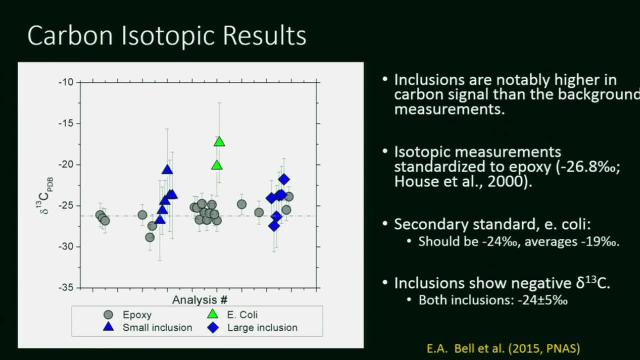 the isotopic results. so what I'm showing you here, all the isotopic results here have already been corrected to our standard here, our standard: the accepted value is shown here on the dotted line and you can see that they cluster about the accepted value pretty well. 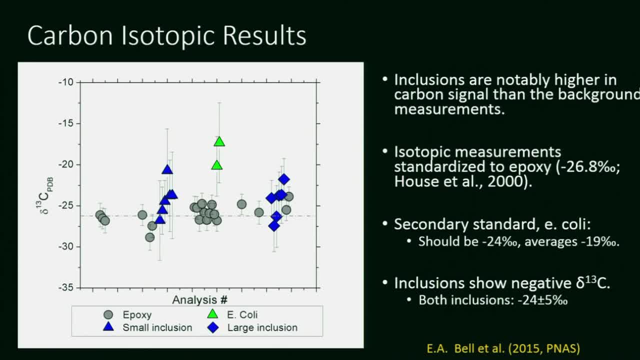 and our, indeed our, graphite inclusions, both plot quite similarly, such that we're going to average them together to get our average delta C 13, which is minus 24 plus or minus 5 per mil. so what does this mean in context? so we have 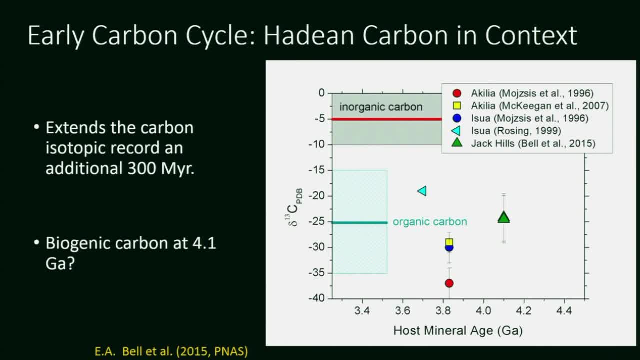 isolated inclusions of graphite in this 4.1 billion year old zircon, and they are minus 24 per mil. so we- this is again. I'm showing you- delta C 13 in this time versus geologic time or versus age, rather, and you can see this field for 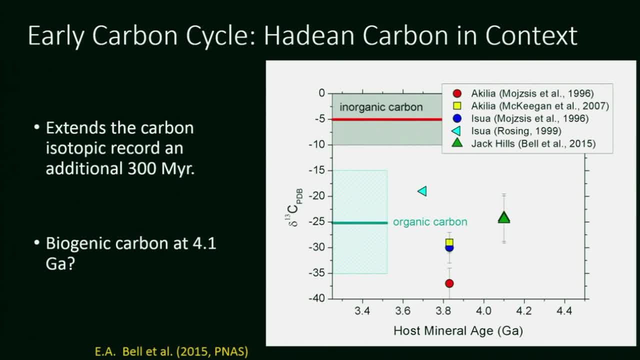 organic carbon coming in here to the extent of the microfossil record I'm also showing for reference inorganic carbon. so at 4.1 billion years we have very negative carbon. it looks very much like biogenic carbon has throughout the time in which. 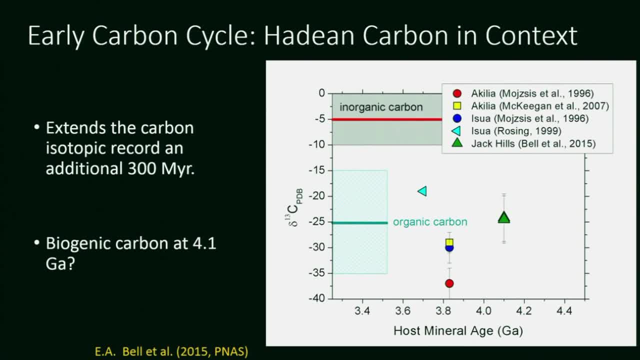 we've had a fossil record. it is very highly offset from the region of inorganic carbon. and so what does this mean? well, for starters, we have extended the carbon isotopic record an additional 7 million years into the Hadean, and this is even in this time before we had 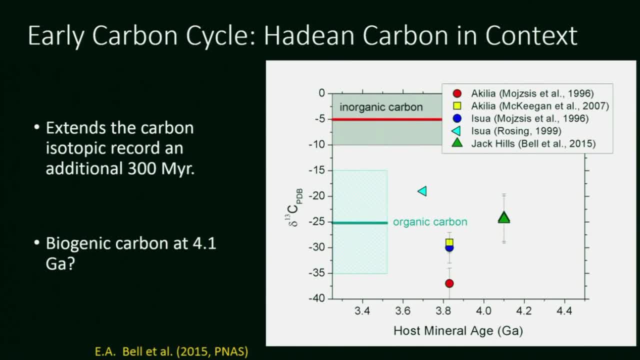 a whole rock record. this is a way forward to really start looking at the carbon cycle in the Hadean. now as to is this biogenic carbon? well, I mean, if you were to find this carbon isotope signal on earth today, you would almost certainly interpret it as: 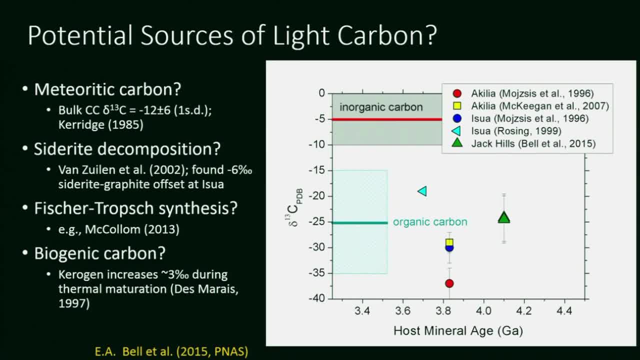 biogenic. but let's look at some other potential sources for light carbon, because this is the Hadean and we don't have previous evidence of life there, because we don't have a rock record. it's very difficult to say so one of the other. 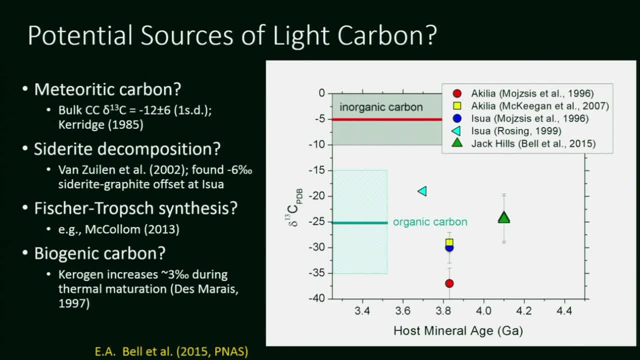 major avenues for getting light carbon into this zircon is if it's meteoritic- and this is nice because we can see meteorites that are falling to earth today- we can look at their carbon isotopic signature, so carbonaceous chondrites is what I'm going to take as an example, because they can 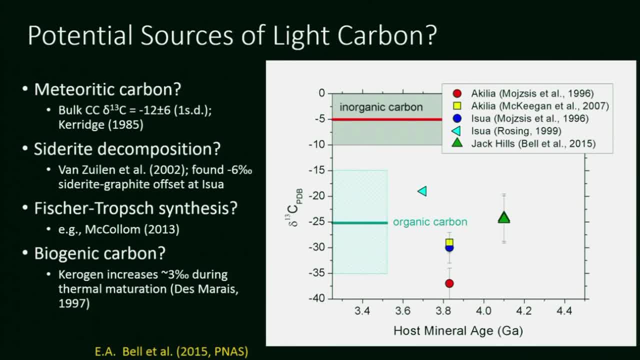 get up to several weight percent carbon, and so, although they have individual chemical components that are organic, that can range very widely in delta C 13, from very, very positive to very, very negative, the bulk carbon of these carbonaceous chondrites tends to be about minus 12. and I'm showing you: 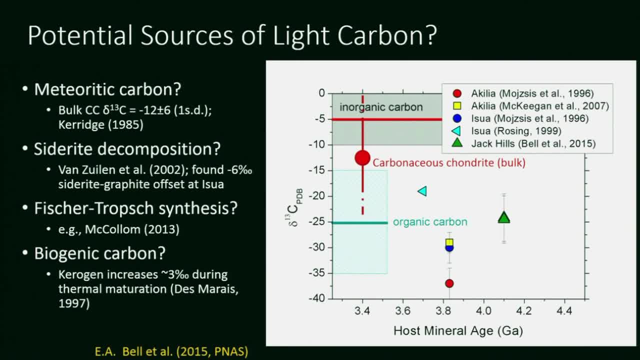 here the average of plus or minus 2 standard deviations here, and so you know this. the lower reaches of this does overlap with the field of biogenic carbon. so the question is, did we just get unlucky and we got the zircon from the place where the carbonaceous chondrite hit? 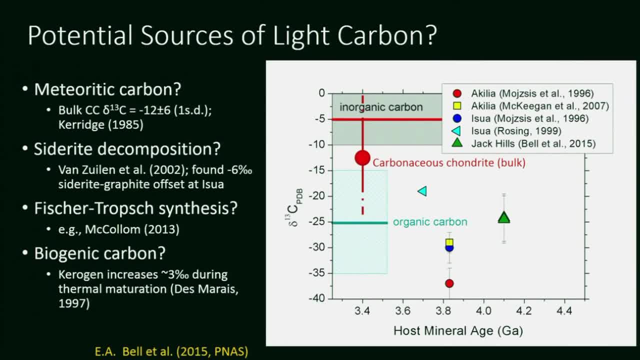 or is this biogenic or does this come from any of these other possible mechanisms? so other ideas that people have come up with to get light carbon: the idea that various minerals like siderite, which is an iron carbonate, their decomposition has. in particular, at Greenland there is 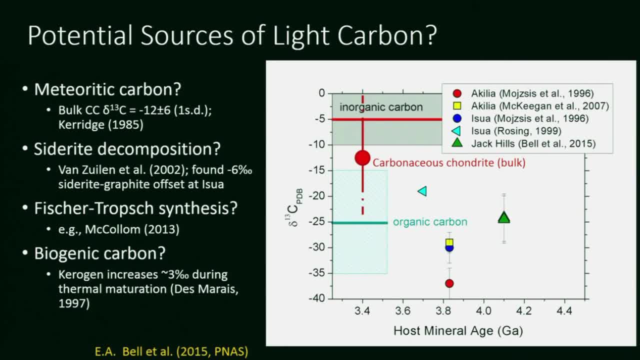 a study suggesting that the disproportionation of this carbonate mineral could have formed graphite. and indeed if you look at these sort of paired graphite and siderite in this location, you can see somewhat lighter, that is, more negative, delta C13 in the graphite, but the offset is not really that much. 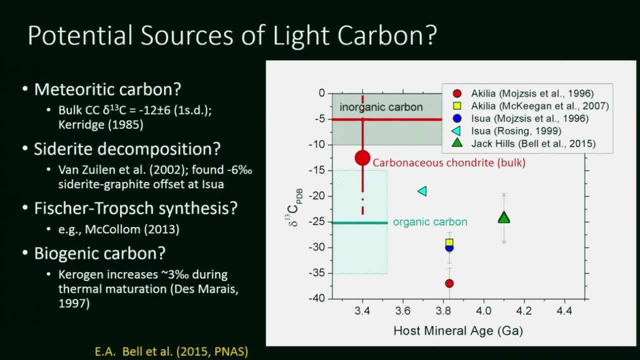 it's only around 6 per ml. other ideas are fischer troth synthesis. this is a broad type of reactions which can abiotically synthesize hydrocarbons and has been variously attributed to forming methane and various other hydrocarbons abiotically in the earth's mantle. 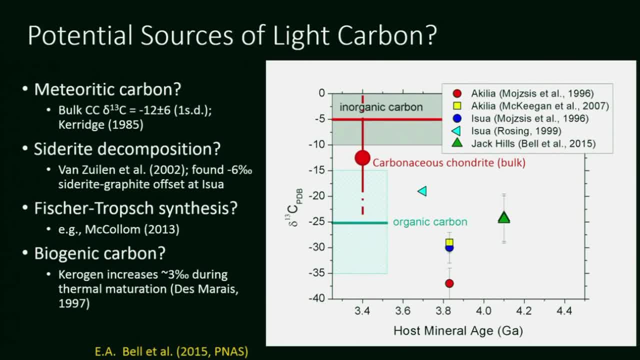 and so forth. so the question is, however: we're going to get this carbon? we need to get it into our zircon. so we have a zircon. it looks like it came from a granite. I neglected to mention the crystallization temperature of it beforehand, but it's 650 degrees. 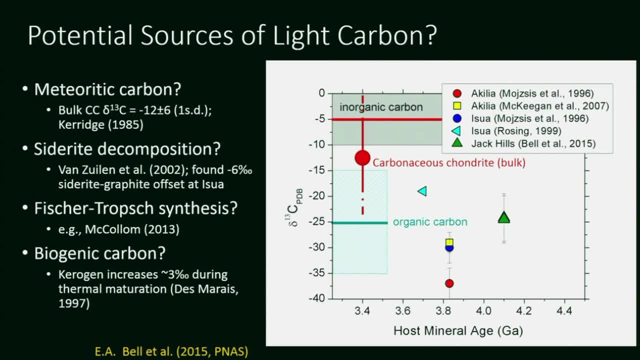 Celsius. so it's again one of those very low temperature looking zircons, very granitic. looking elsewhere in the zircon a quartz inclusion was found, and so this is all evident further evidence that this could be from a granitic magma. so we need to take this. 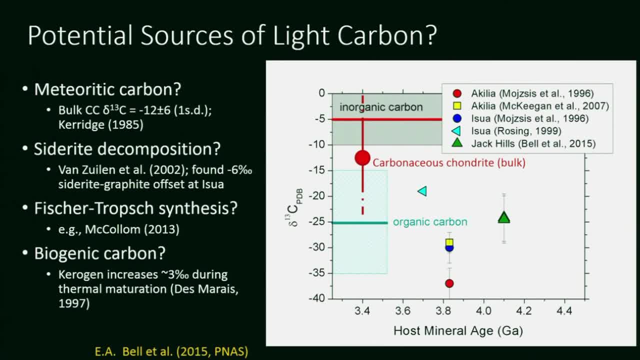 carbon. we need to concentrate the light carbon, put it into a granite magma and then trap it in our zircon. well, here's where the biogenic carbon mechanism comes in and perhaps has an advantage, because we know that throughout the phanerozoic earth, when we look at sediments, we can 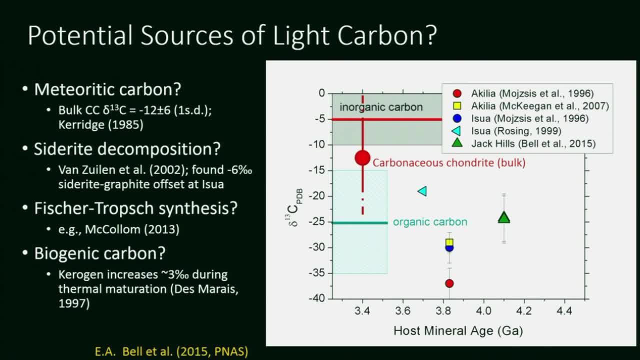 find very high percentages of carbon, so up to 10 weight percent or so, in some sedimentary systems of biogenic carbon, and indeed, when you do melt these sediments and form magmas from them, you can see the chemical effects of this carbon, so that it does. 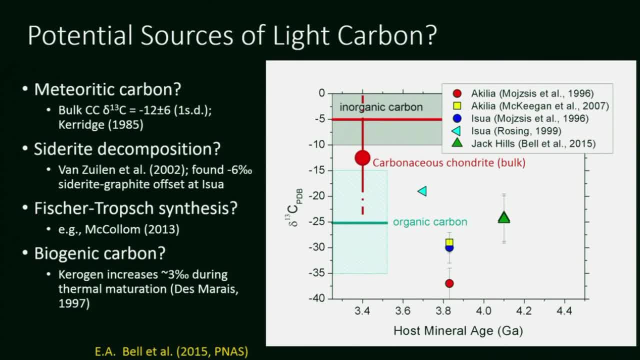 persist as graphite into the melting phase, and so we see the much more reduced magmas coming from these sedimentary type environments versus magmas that are melted from igneous rock precursors, then this is owing largely to the graphite. so if we were to have sediments with biogenic 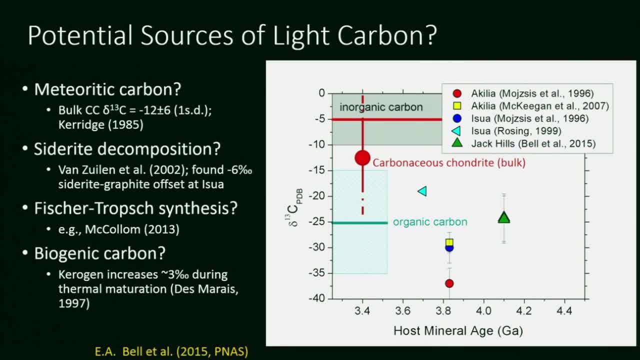 carbon in the Hadean and then this gets melted, because we have previous evidence for sediment melting to form many of these zircons. this is a mechanism by which you could get biogenic carbon into a Hadean zircon. now what can we say with one data point not. 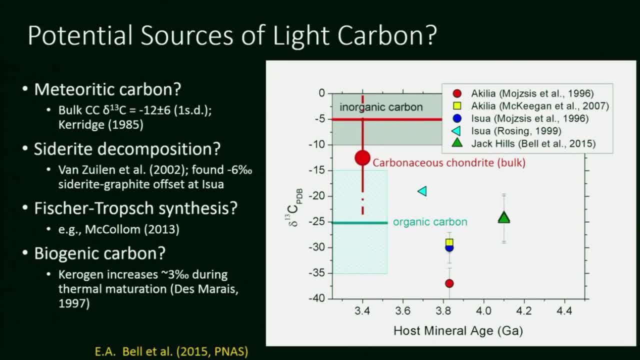 much we can talk about. you know this mechanism, that mechanism, but what we really need is a lot more data. so I mentioned there are several thousand of these Hadean zircons archived at UCLA. we have, as of January 2016- we had looked at about 750. 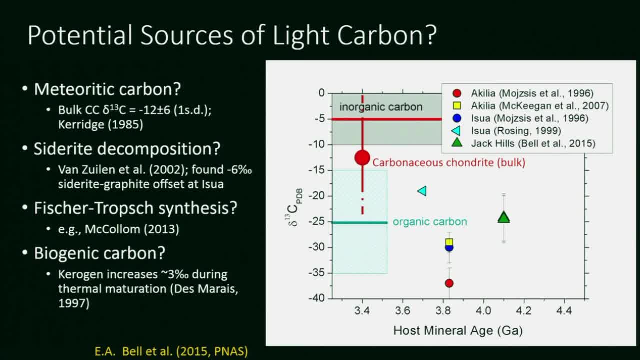 of these zircons with transmitted light microscopy, which is our first screening step for seeing if they might contain graphite. so let's imagine that we are able to build up an archive of ten or tens or a hundred of these inclusions, and then we're really able. 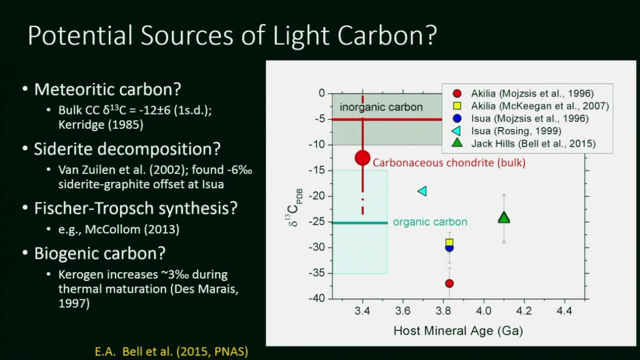 to get the carbon isotopic record, we're able to get the spread in carbon isotope ratios that we're seeing for the Hadean and at that point, if we're seeing something that clusters around minus 25 or lower, or if we're seeing something that looks more like this sort, 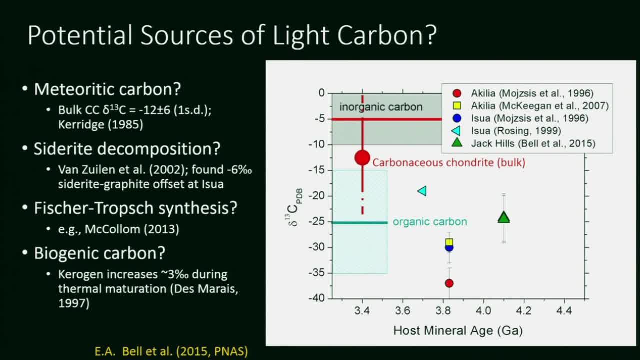 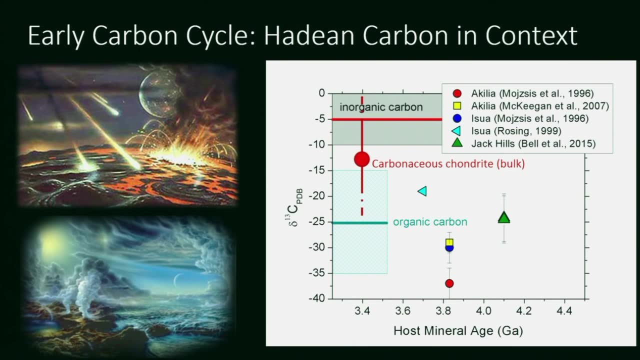 of broad and centered higher meteorite distribution, then maybe we can start talking about probable mechanisms and, with more certainty. so, to briefly summarize, bring around to our initial theme of this talk, which was: what had the zircons been telling us about the early earth? that is different. 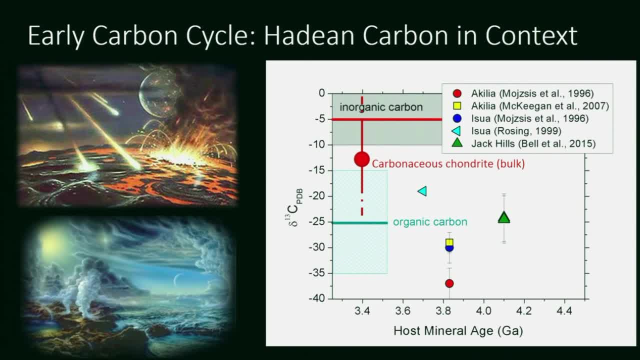 from what we originally thought. the overall theme of what the zircons have been telling us is that the early earth was a lot more clement, in fact, a lot more like the modern earth in many ways than what we had originally thought. so, instead of the idea of a very 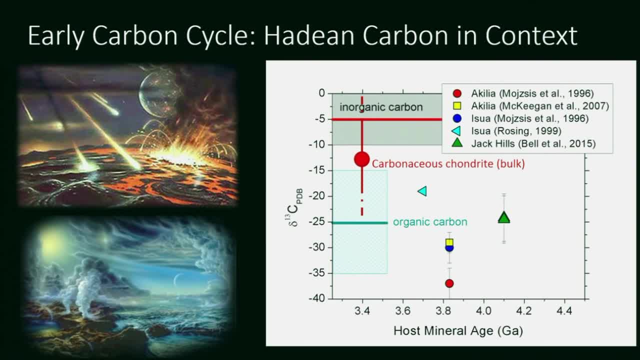 inhospitable environment. we could have had a hydrosphere very early on. and if we have a hydrosphere very early on, if we have this evidence for this evolved sort of granitic like crust, perhaps a bit more stable- of an environment, is this really inconsistent with? 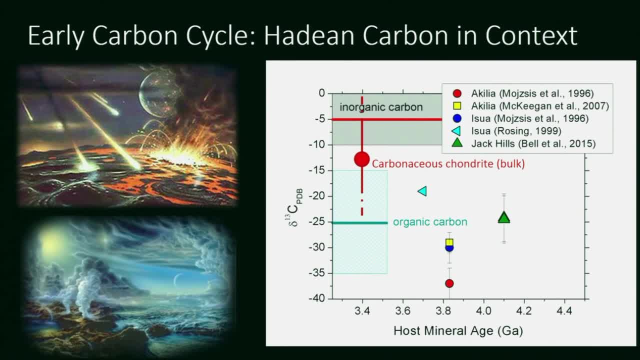 having life at 4.1 billion years or perhaps earlier, if we are able to really go through this zircon record. we have zircons as old as nearly 4.4 billion years at Jack Hills. although earlier than 4.2 billion years, they get much more. 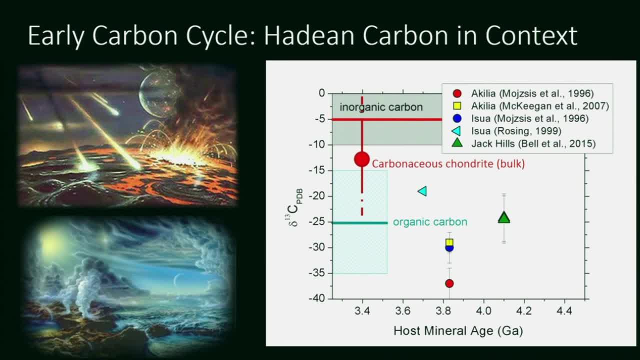 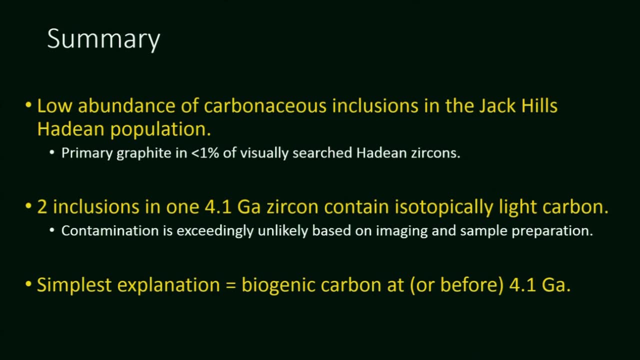 sparse. can we really push back in time the earliest carbon isotopic evidence that we are able to get, and can we this way constrain when the origin of life on earth was so? to summarize, we have found that there is a low abundance of carbonaceous inclusions in the Jack Hills. 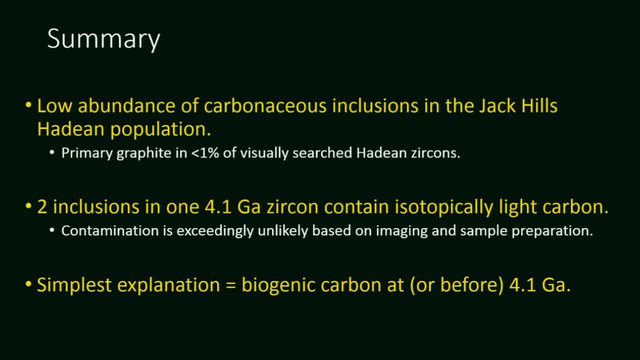 population, but it is present and it is something that we can exploit. we can get carbon isotopic measurements from it and there is some degree of primary graphite in these zircons. in fact, we found primary graphite in, at this point, less than 1% of our visually searched. 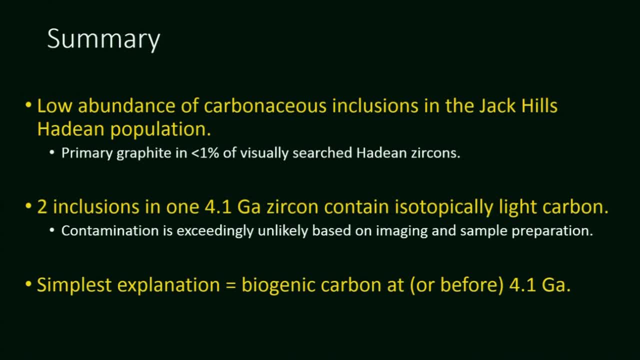 zircons, but we have ongoing spectroscopy to figure out just how accurate that 1% number is. so our sort of star data is 2 inclusions and 1 4.1 billion year old zircon. they contain isotopically like carbon. 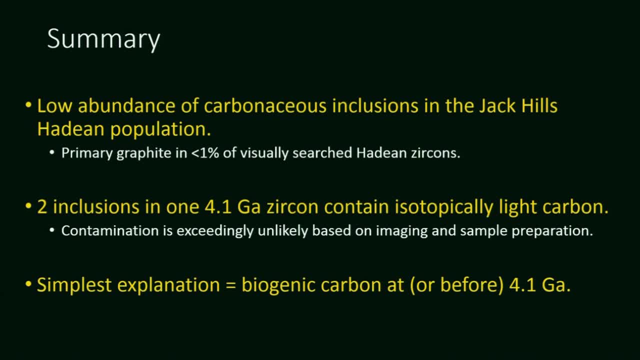 and the contamination of these phases either over geologic time or in the laboratory is exceedingly unlikely, based on the imaging that we have done and our preparation steps. so the simplest explanation we consider for this is that we had biogenic carbon at or before 4.1 billion years. 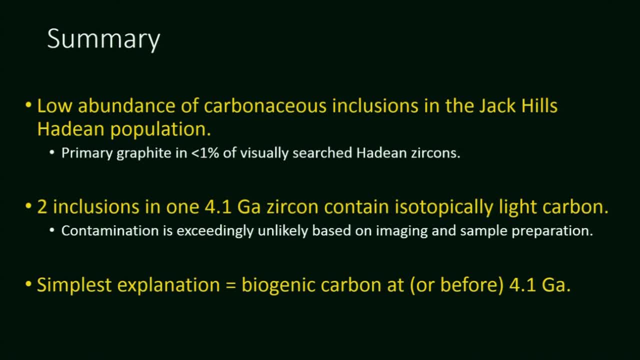 remember. we can't date the carbon directly. we can date the host zircon. we know it was 4.1 billion years old, so the carbon itself could be 4.1 or even earlier. it is impossible to say at this point in time. so where do we go from here? 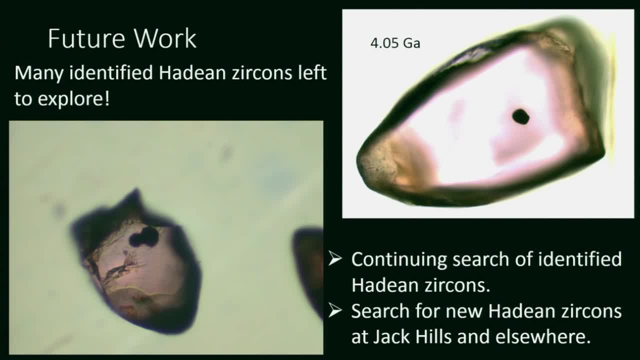 there is a lot of future work to be done. we have many identified hidean zircons that are left to explore at UCLA alone and in particular, so this is a new image that you haven't seen yet, but I mentioned that, as of this January, we had looked through 750 of these. 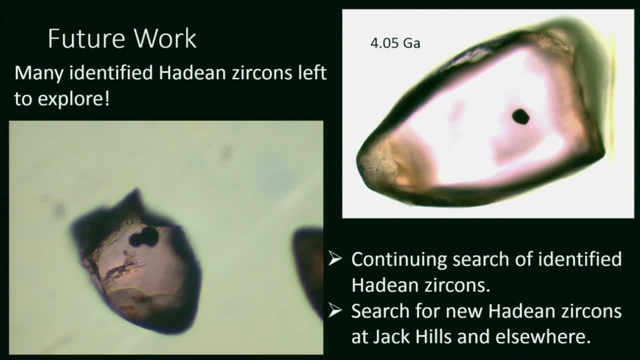 zircons visually, but we actually just started a new phase of this project in which we are doing automated visual search of these zircons. my co-author, Patrick Booka, and I last week headed down to Melbourne in Australia to use an automated microscopy set up in the lab of Andy Gledow. 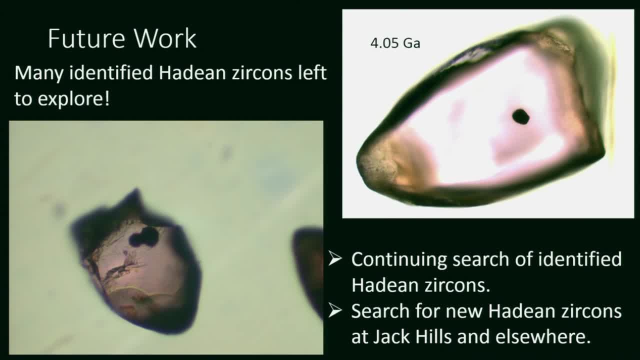 and so we have in the past week looked through 2300 hidean zircons very quickly, very efficiently, and we are even now just trying to process all the data and figure out. so this is one of the very nice inclusions we found. you can see, there is no visual evidence for cracks. 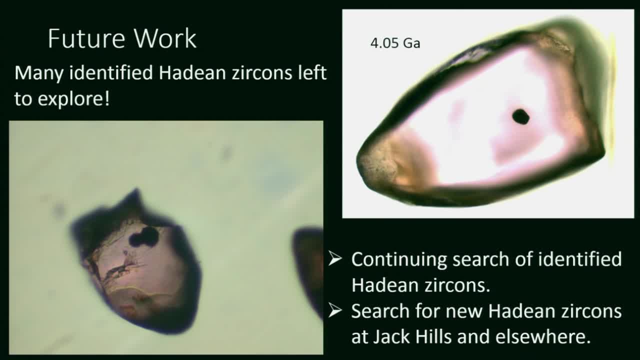 this is a very nice dark inclusion. we haven't done Raman spectroscopy yet to see if it is graphite, but this is in a hidean zircon, so this could be our next target for isotopic analysis if it turns out to be graphitic. so we have 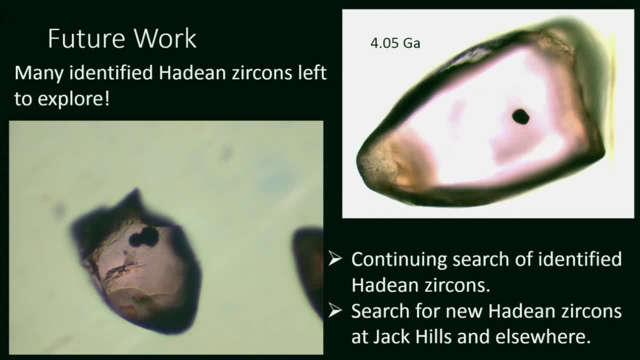 this continuing search of identified hidean zircons, we have now begun a new campaign of dating at UCLA. we are looking through several thousand more of these jack hill zircons. we have mounted up around 10,000 so far that we are steadily going through on the ion probe. 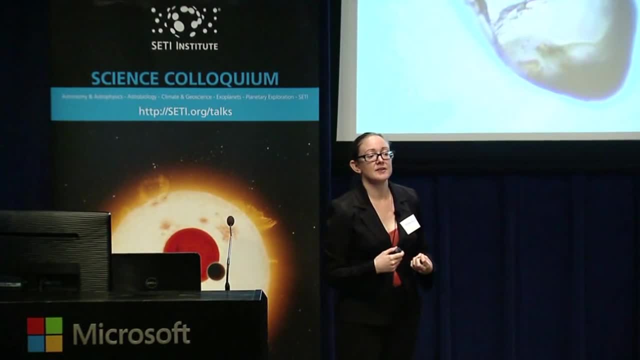 to find the hidean ones, and this is going to this in particular- was this particular study was motivated by looking for evidence of paleomagnetism. this is a study led by Ben Weiss at MIT, but we are also going to be able to then have these for our search for. 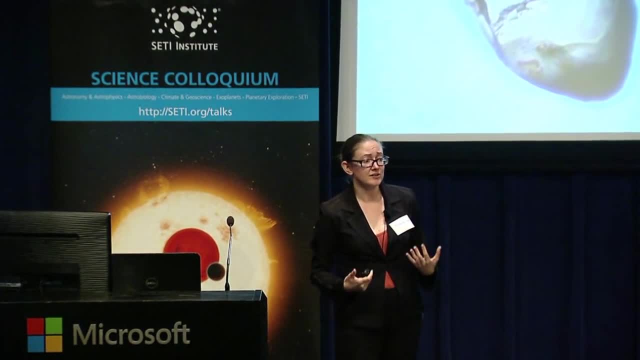 hidean life as well. and also the jack hills is not the only locality on the earth where we find hidean zircons, it's just the only one where we find them in such great amounts that they are really able to be exploited in a systematic manner. we have 3-5% zircons in that rock that are older than 4 billion years, but there are scattered hidean zircons that have been found in various places, often in sediments from the Archean time, so before 2.5 billion years ago. the north china creton has yielded several of these. recently, a single 4.1 billion year old zircon was found in brazil coming out of the amazon creton, and so there are a number of different places where we could potentially find more of this hidean material, and indeed, 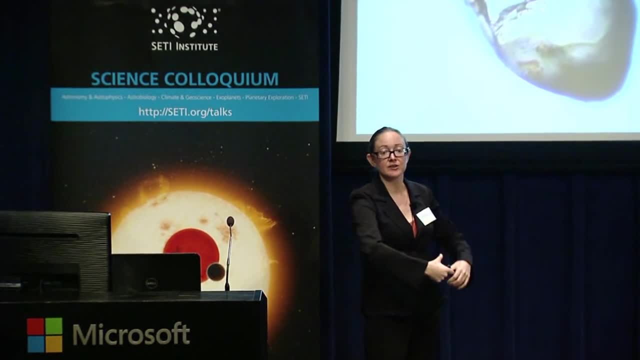 this would make a nice counterpoint, for so at jack hills, this is one locality where we are able to look at the hidean, but if we can counterbalance that with other localities around the planet, if we are seeing different geochemical stories or a more coherent 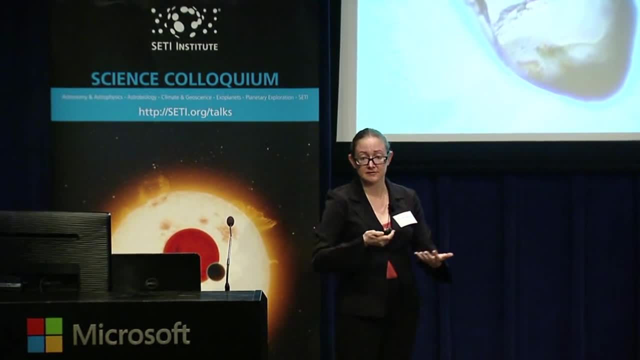 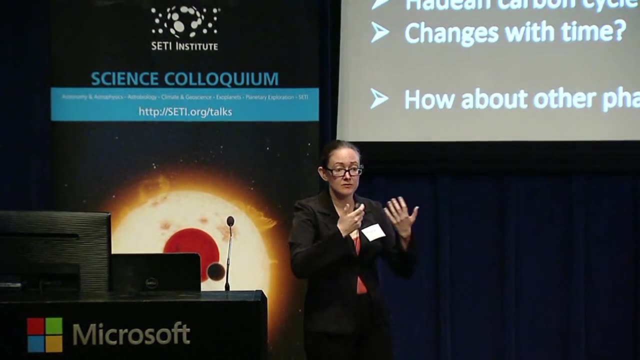 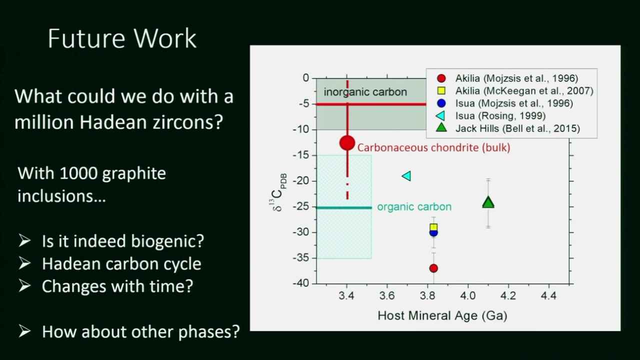 geochemical story. if we are seeing graphite in these various localities as well, this can very much help make the case that we are seeing a hidean carbon cycle. that was sort of a global implications, and so what could we do if we had looked through a million hidean zircons? 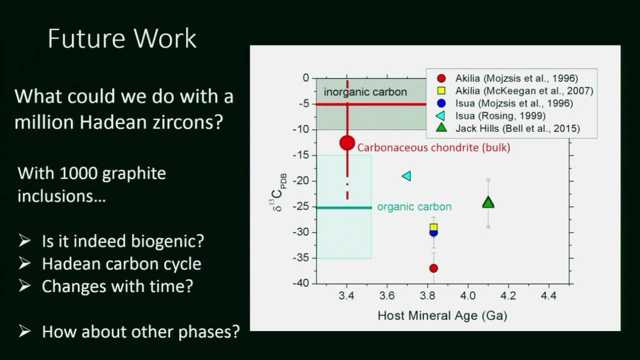 so let's say we have looked through a million hidean zircons and we found graphite inclusions. at this point we can really start to talk about whether this really looks biogenic. are we seeing a biogenic like signature distribution in the zircons? 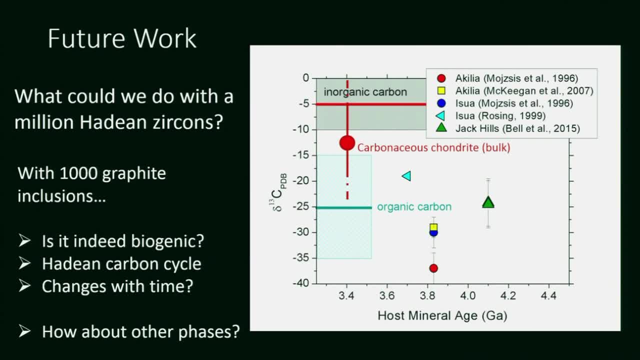 are we seeing a more meteoritic looking distribution or something altogether different that tells us there were other processes we haven't thought of yet going on in the hidean, and can we then get a time series? can we see the change in time, both to push back further and further? 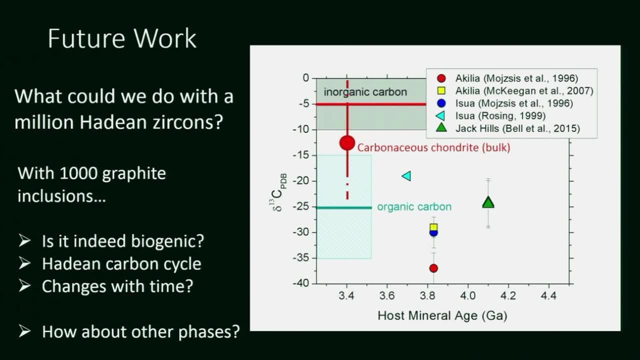 towards the origin of our planet and see if we can talk about the origin of life, or so there are various events proposed at around 3.9 billion years, this idea of a late heavy bombardment or a major spike in meteorite impact rates. some people want it to start at 4.2. 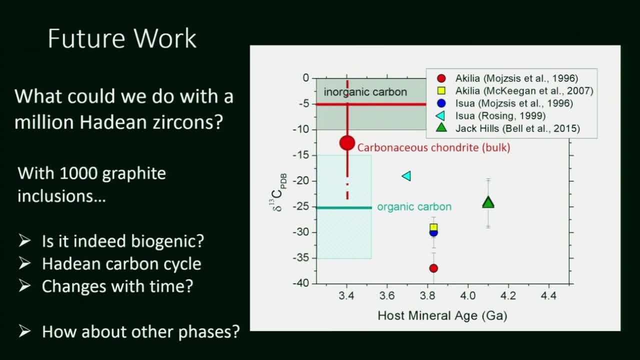 or 4.1 billion years now, or for there to be multiple spikes, but the idea that there could have been cataclysms in the inner solar system with much higher impact rates. there's a lot of argument in the literature about what effect this would have had on life. 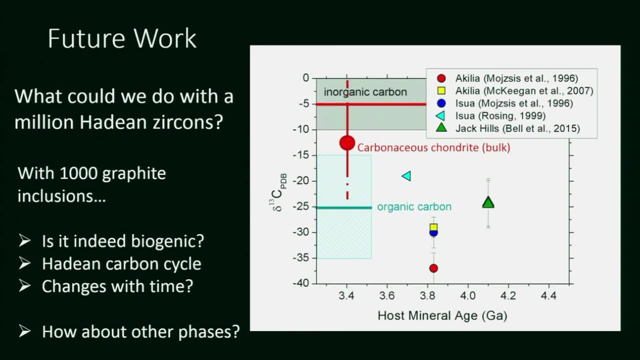 would this have sterilized the planet's surface? just so much material coming in that it would have wiped out any biosphere. so would we be seeing sort of an early, 4.1 billion year old biosphere? if this is indeed biogenic, that then got wiped out. 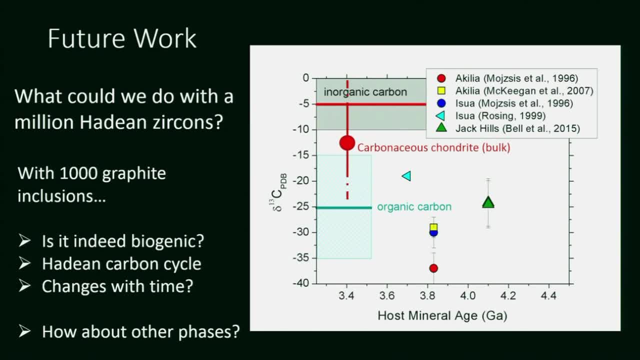 and an entirely new one came up that gave us the 3.8 billion year old measurements. or in fact, do we not see a response or a change in the delta C-13 during this purported late heavy bombardment time period? and in fact there are some studies that suggest that? 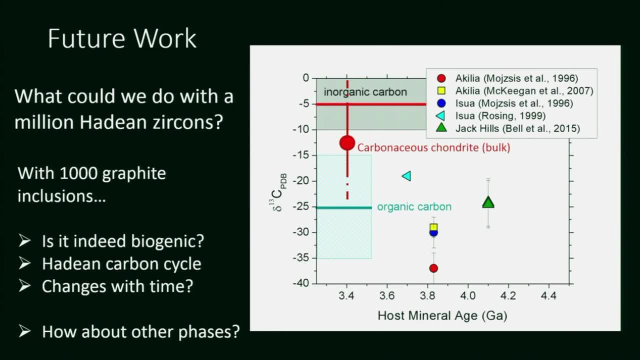 for hyperthermophiles at least, these impacts might have set up big hydrothermal systems that might have in fact been nice habitats for a select subset of microbes. so there are a lot of questions to go through with this, that we really need a lot more Hadean zircons. 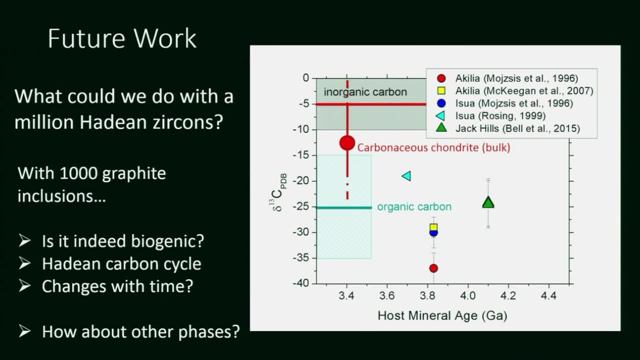 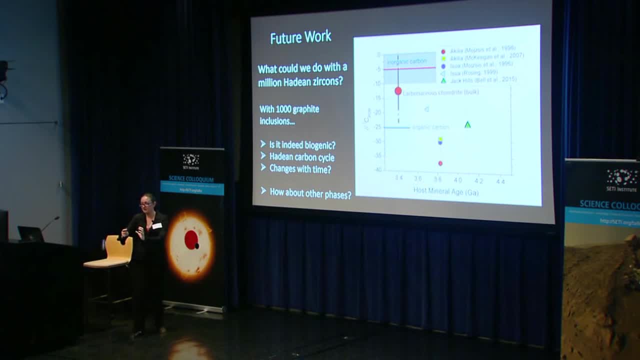 and a lot more Hadean graphite to answer, and so this is a very exciting field of study we have now. we see our study as sort of the proof of concept we can find this stuff, we can isotopically measure it. so where do we go from here? 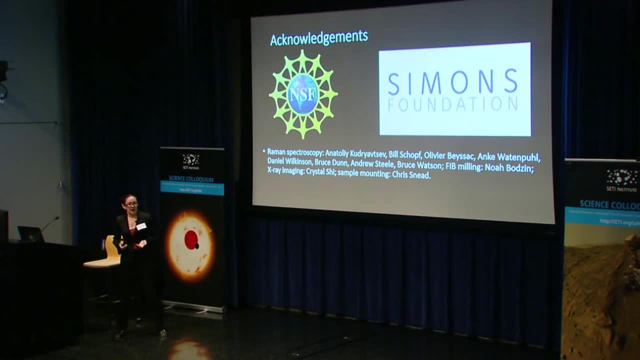 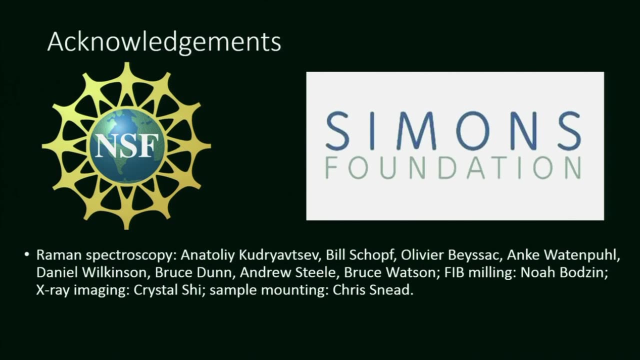 and before I take your questions, I would just like to briefly acknowledge our sponsors. so the Simons Foundation has funded my post doc fellowship, on which I've been doing this work over the past two years, and the National Science Foundation has been funding the Hadean project at UCLA for many years now. 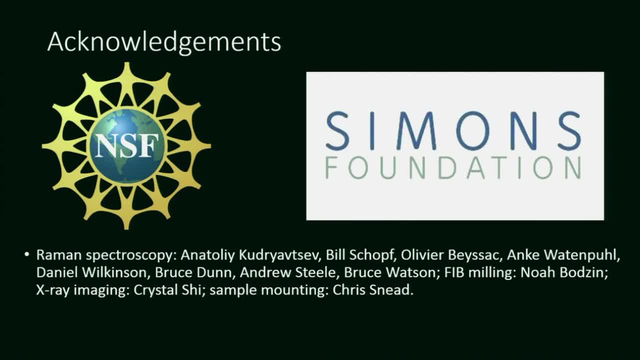 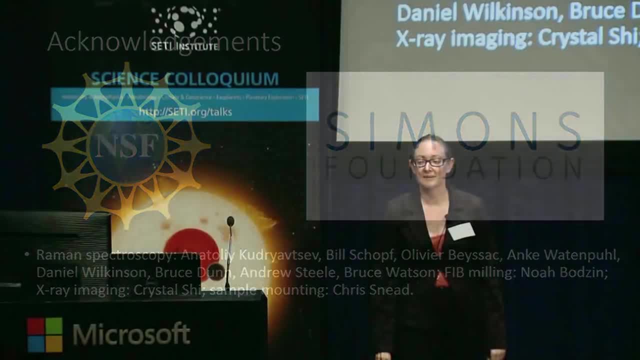 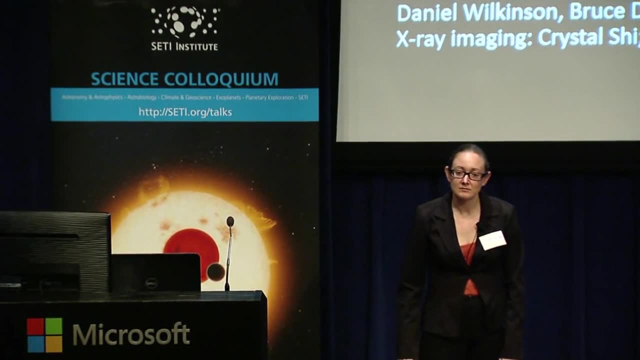 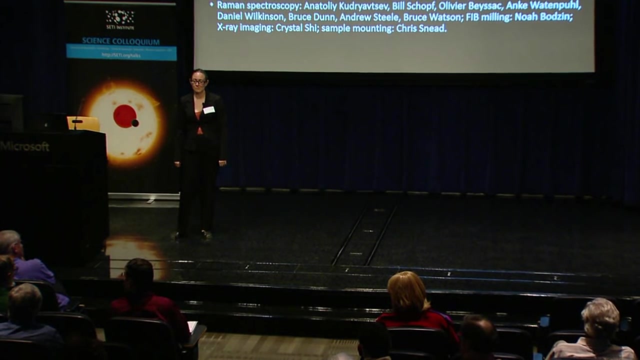 and thank you. thank you, those people have questions. can you tell anything distinctive with regard to the meteorites and biogenic terrestrial using buckyballs or or perhaps some other form of graphite? so I don't know about looking at other forms of graphite. I don't know the extent. 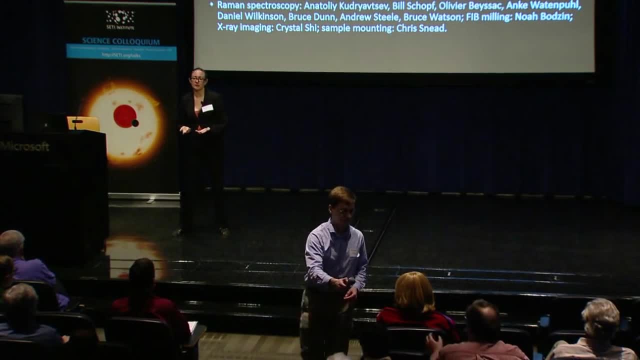 to which we'd be able to tell this. it would be a matter of if we can see it in the realm of spectroscopy. one thing we have thought of is that if we have large inclusions, like one of the inclusions we've just identified- this January is like 50 by 30. 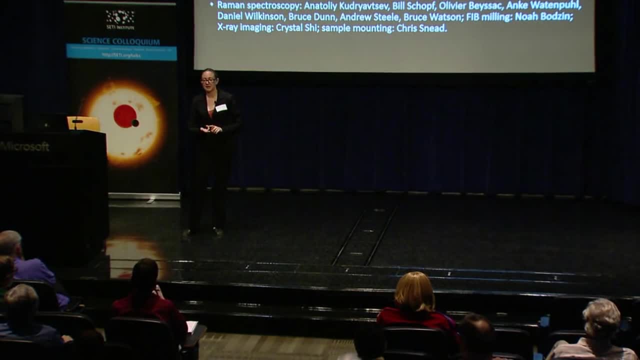 microns. if there's a lot of material there. after the carbon isotopic analysis we might be able to look and see if there are other elements present- nitrogen, sulfur hydrogen- that might be more indicative of one origin or the other. that's something that we want to look at in the future. 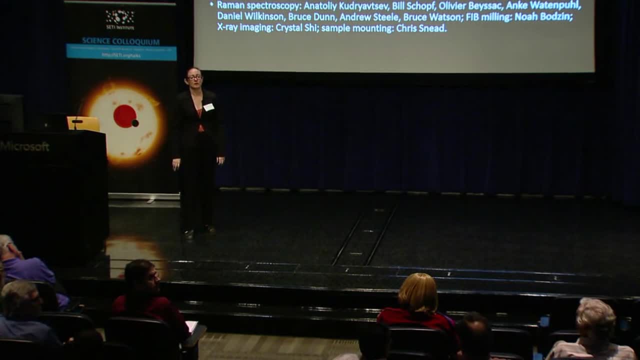 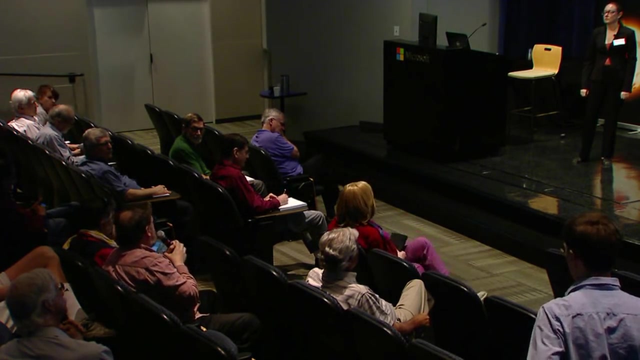 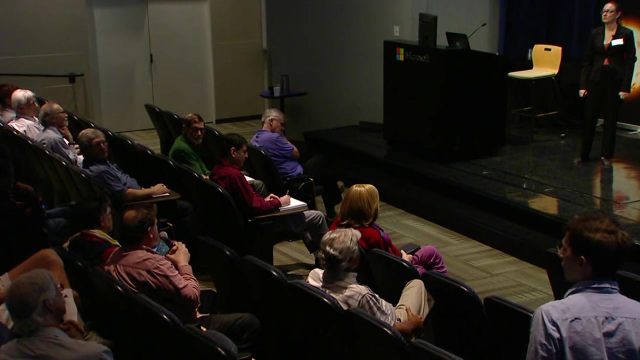 hello, thank you for a really fascinating talk. as a secondary thing, in addition to searching for life, you're helping to characterize the Hadean with this work, and if you were able to get a wider range of ages, would you potentially be able to do? 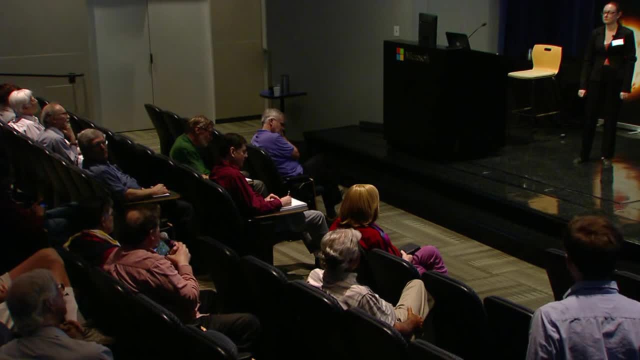 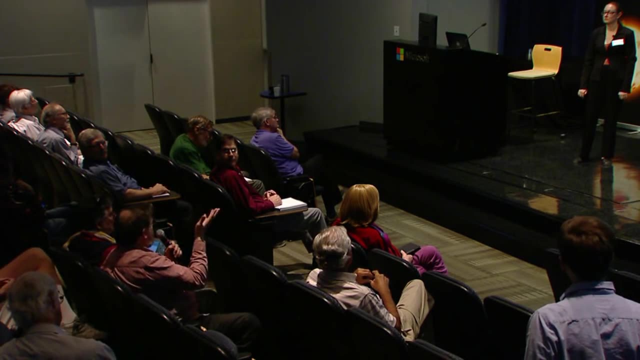 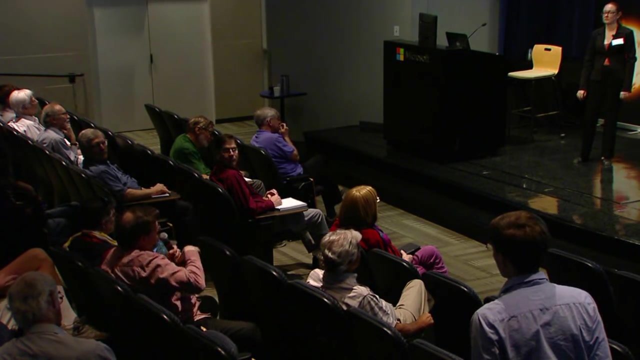 characterization of the environment during the late heavy bombardment or even pinpoint. help pinpoint the exact time of the late heavy bombardment and see if it's consistent, like if the carbon isotope ratio drops lower or goes higher, like spikes in one direction or the other. would that be? 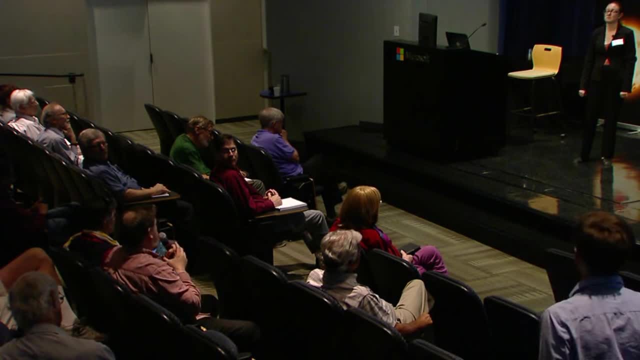 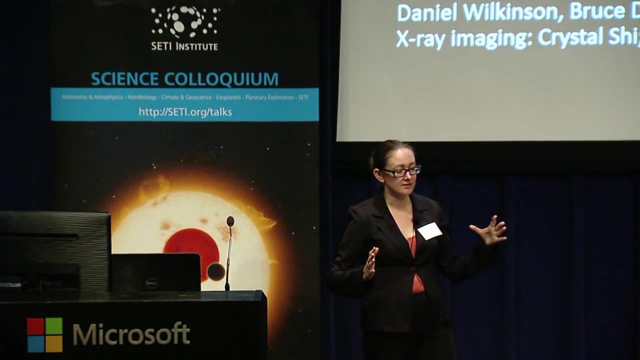 help you figure out whether a hydrosphere could have survived at least parts of the bombardment. yeah, so we have that span, the time period that is suggested for the late heavy bombardment. they are pretty much continuous between 4.3 billion years. 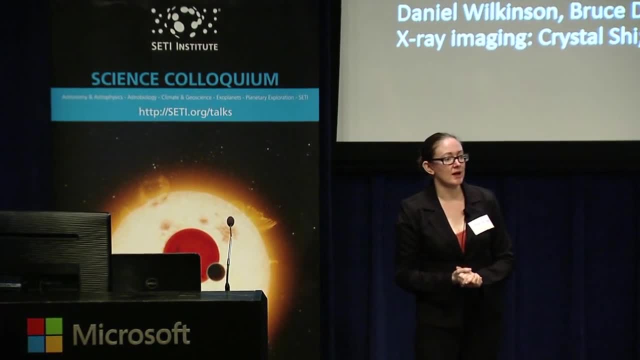 and about 3.8 billion years, so we have zircons throughout that time period. and, yeah, it would be really interesting, I mean, if there are excursions in the carbon isotope record during that time, that would be really, really exciting and probably have these sort of. 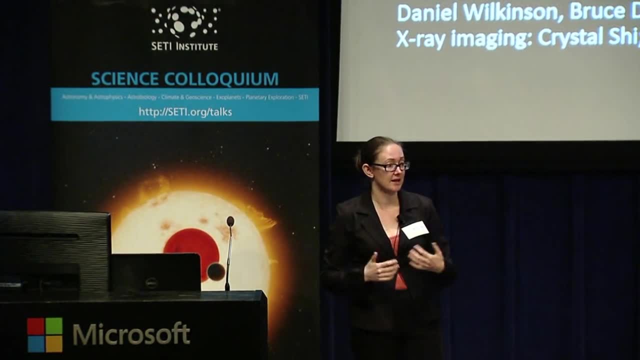 biosphere implications for what was happening during the late heavy bombardment. if there was indeed such an event, we could maybe help characterize it that way. other geochemical systems in the zircon show interesting things happening around the time period of 4 to 3.8 billion years. 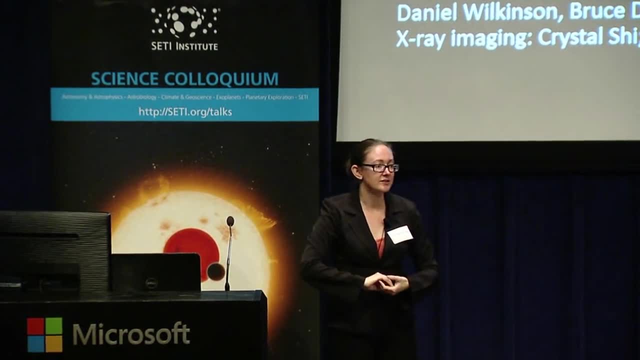 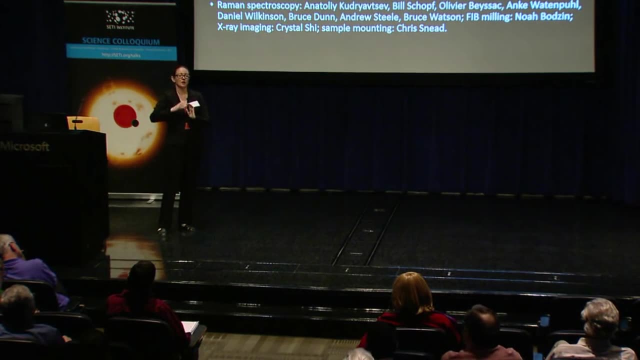 so it looks like it might have been a period of some sort of tectonic transition. if you look at hafnium isotopes, there's a loss of some older crust during that period. you have a new, juvenile crust being melted from the mantle and coming in. so 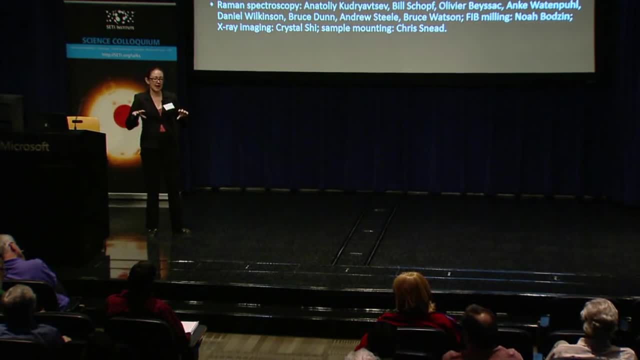 it might be a little bit complicated to sort that out from any changes in the carbon signal, but that would definitely be something to look for. Thank you for the talk. it was really good. I learned a lot about zircons here, which I am completely not an expert on. one question I have- and you might have mentioned this, and it's multiple questions actually- is the only way to form the zircons in a magma chamber, and if so, you're kind of assuming that there's already plate tectonics at about 4.2 billion years ago? 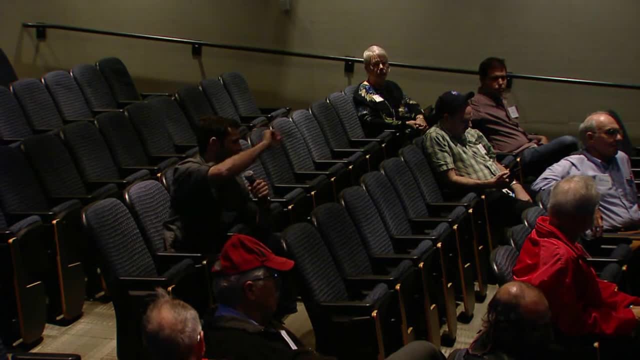 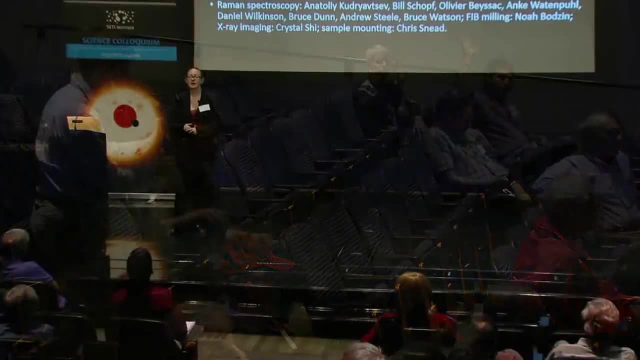 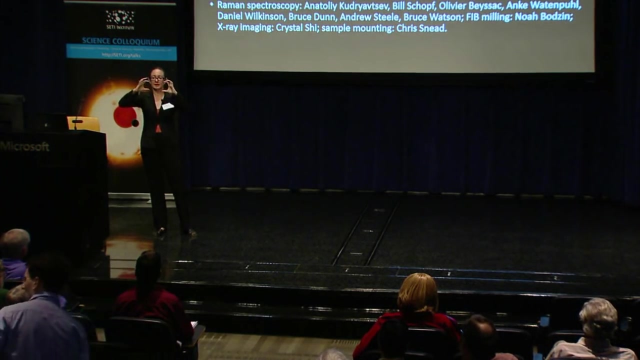 and if that is the case, what is the time scale for this carbon being formed on the surface, being subducted and formed into zircon? that's a good question. so we do. we have many lines of evidence that these zircons are magmatic, both from the fact that 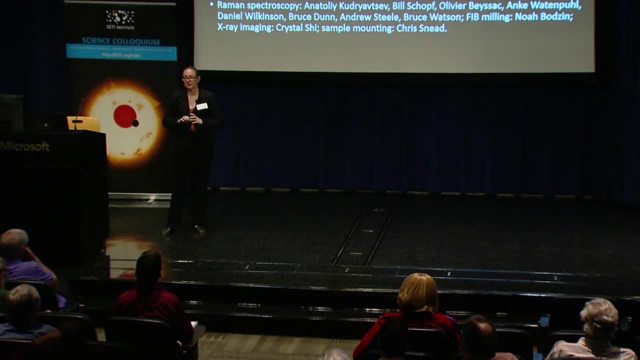 characteristic magmatic oscillatory zonation is preserved in a lot of the zircons and various trace element ratios, like the thorium to uranium ratio, which is characteristic of magmatic zircons we see. so in terms of time scales I honestly don't look too much into. 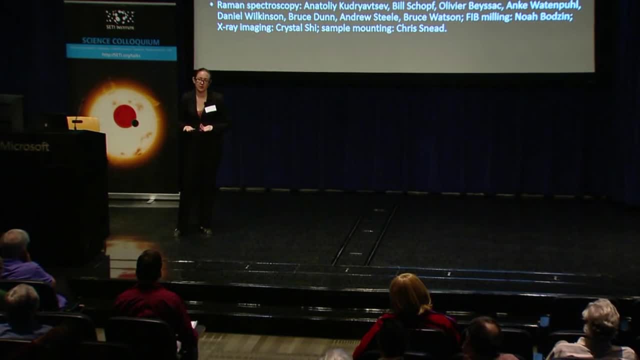 how time scales of if we had an under thrusting environment, somewhat like a subduction zone, how that would differ from the present to the Hadean. at present, it is thought to be on the order of 10 million years to get material subducted and then it can come out. entrained in a magma, but I'm not sure. there almost certainly would have been a much warmer early mantle due to higher rates of radioactive decay or contents of radioactive elements that hadn't yet decayed away. so it's it's hard to say if that same rate would have held. 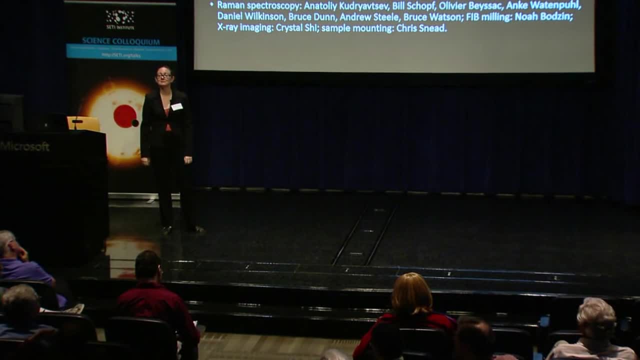 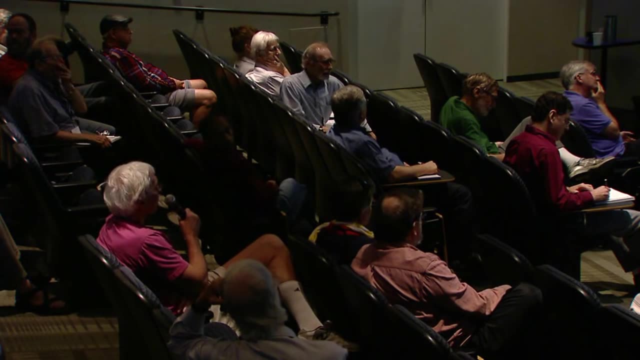 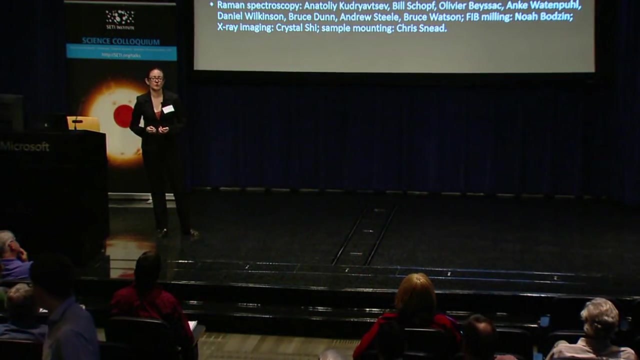 yeah, ok, planet formation is an accretive process. how does science define the actual formation of the earth at 4500 million years back? right, so that's a good question. so usually it will be: when geochemists talk about the formation of the planet, they'll mean the. 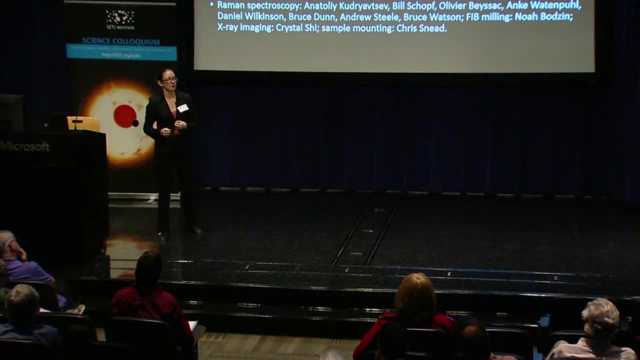 sort of the setting of a certain isotopic system and what I'm using to talk about. so I put the formation of the planet at around 4.5 billion years, and that's based on Lutetium-Hafnium isotopes that we can see in the Jack Hill zircons. 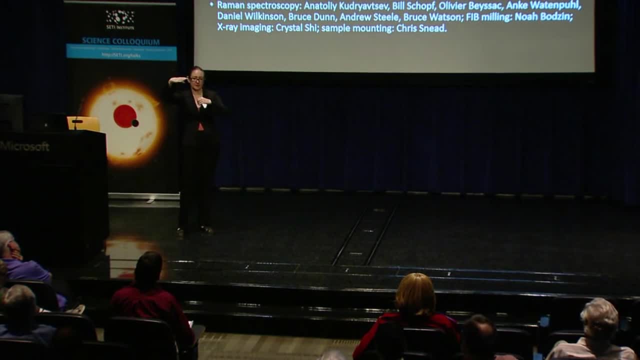 so basically so you have Lutetium-176, which decays to Hafnium-176, and as you melt rocks in the earth's mantle, they sort of like the mantle of the crust- diverges over time and we see the earliest materials, the Jack Hill zircons we see. that require sort of a separation event like that. it must have been pretty close to 4.5 billion years ago, and so that would be my estimate for putting a bound on the formation age of the planet. other people will try to get more specific. there are other isotopic systems. 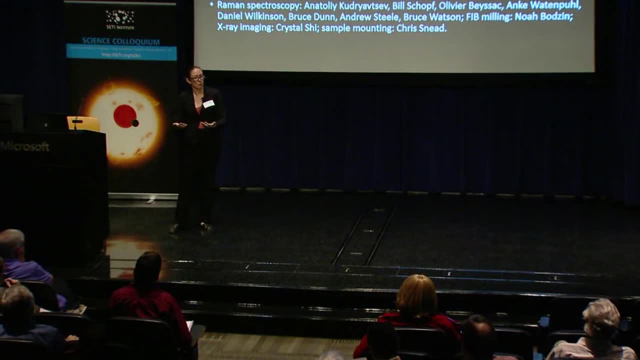 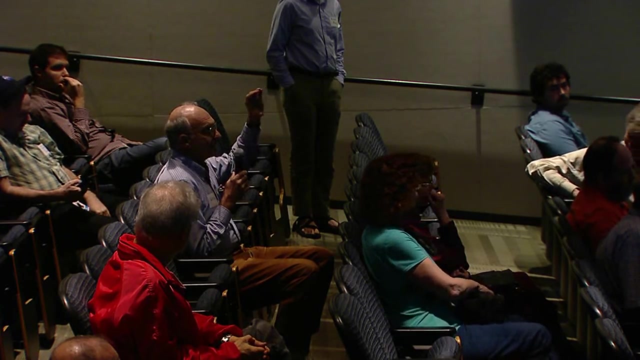 that can give you different information. that's not entirely clear when exactly the planet formed, but that's the number I would stand behind. I'm concerned that there may not be any chemistry approach to produce graphite with the high delta values characteristic of the carbonates. are there any natural? 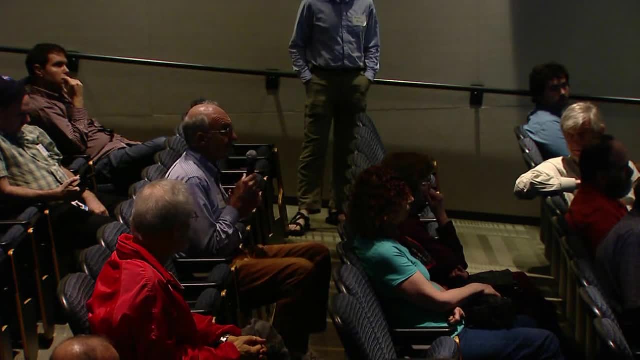 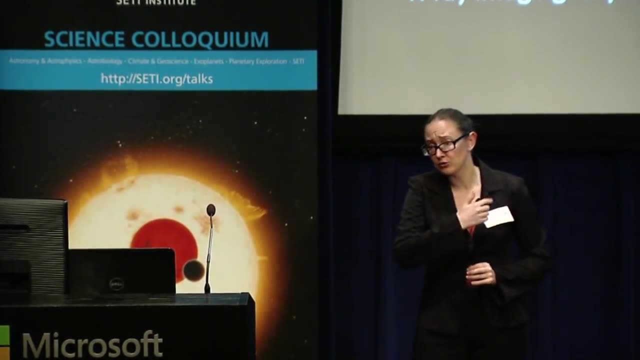 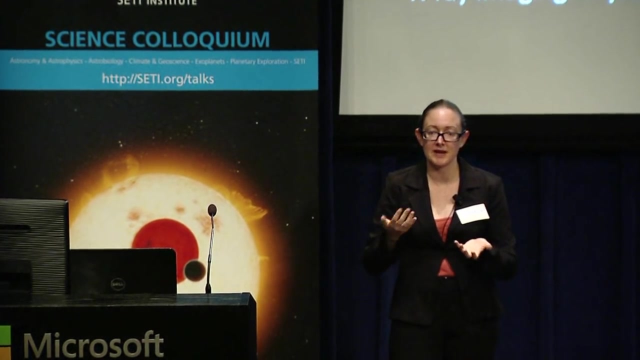 graphite samples that have been found with that property of high delta? oh, that's a good question, so let's see. so there is in Greenland where some of this earlier isotopic evidence in the graphite has been found, while there are the very negative graphites like minus 25 and below. 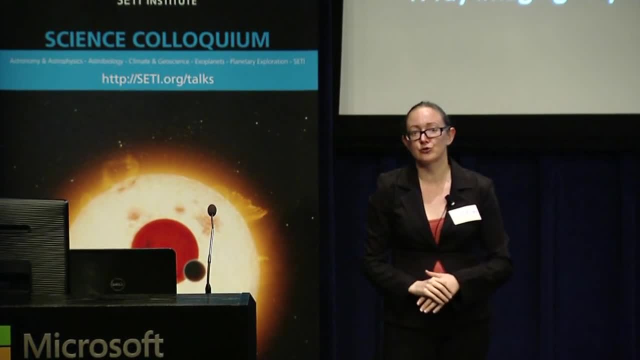 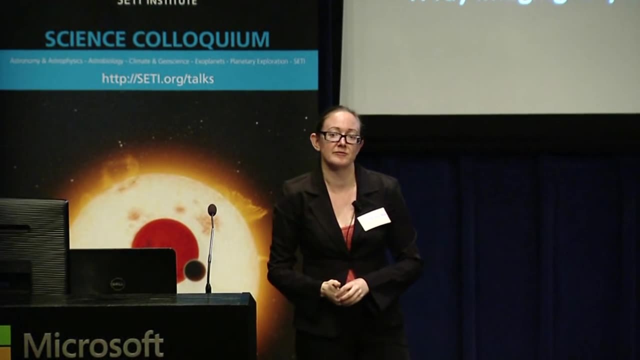 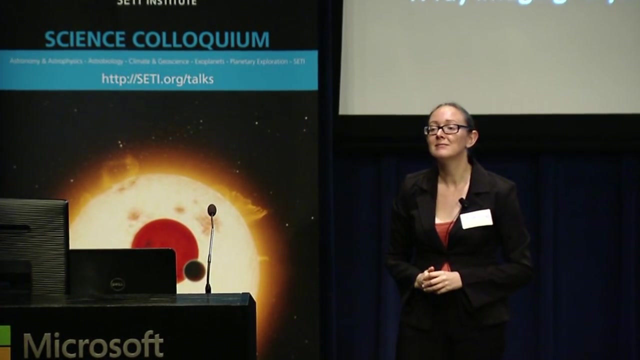 there are also graphites that are much heavier or closer to about minus 10, so that's still not up at zero, but it is much up closer to the inorganic carbon field, so you can get relatively heavy graphite. I've got a. thank you for the talk. 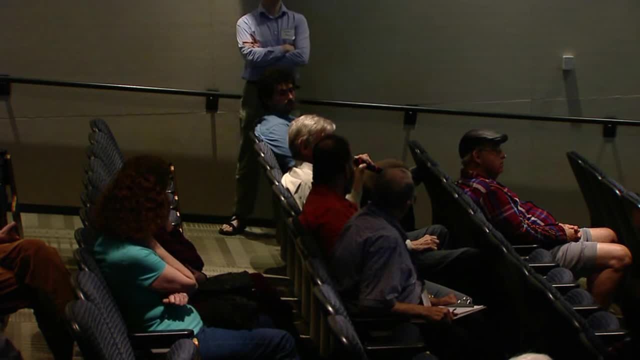 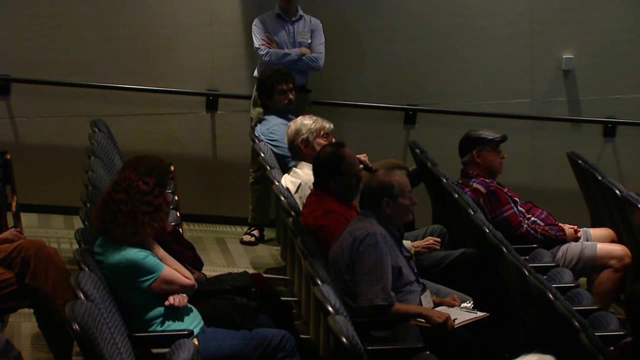 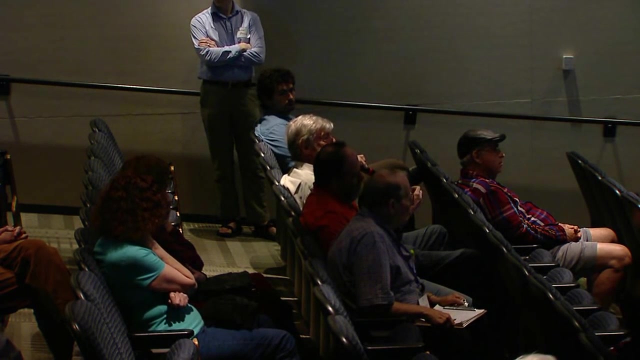 I've got a comment, more than anything else, kind of an editorial comment. to me the term biogenic is it's a pretty high bar. you have these samples, these samples of graphite, and they have interesting properties. isotopic ratios are interesting, but to label them as biogenic. 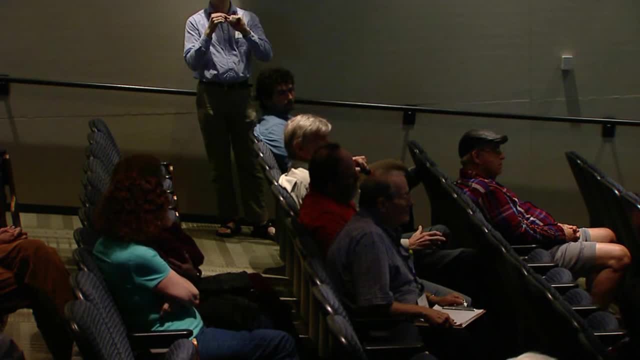 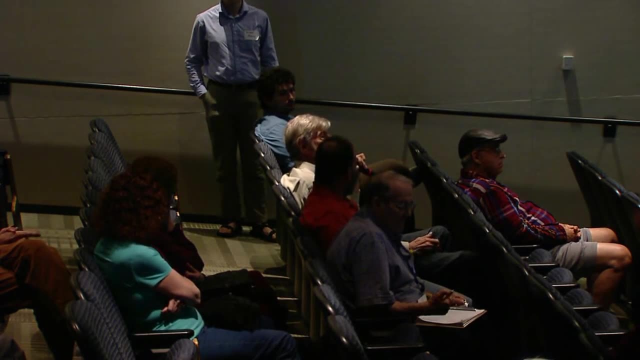 I mean you could say maybe biogenic or biogenic like or possibly biogenic. I mean it's just a personal issue with me. astrobiology is a pretty undefined. it's a pretty wide open field these days and I would hope that we could be a little bit. 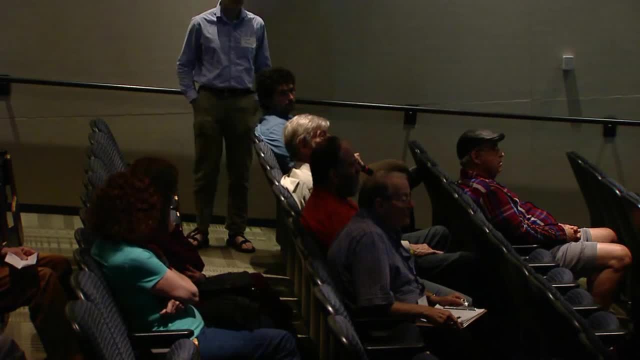 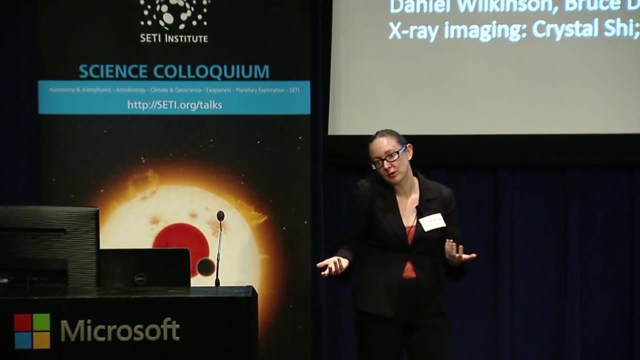 careful with terms like that. that's just again an editorial comment. we do point out this is potentially biogenic carbon at 4.1 billion years, especially with one data point we can't say for certain. I'm wondering the ANU group that ages gives you the ages for the zircons in your collection? 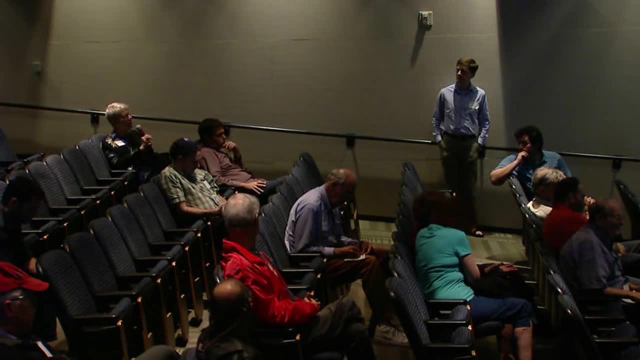 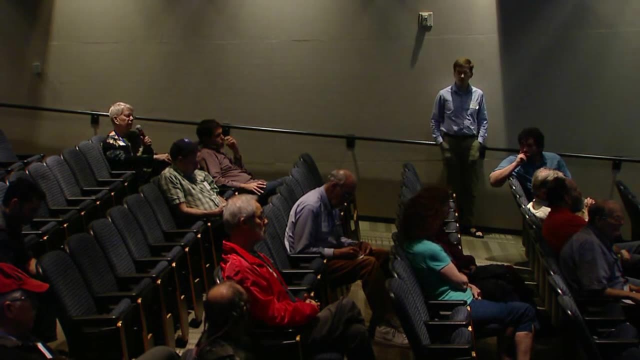 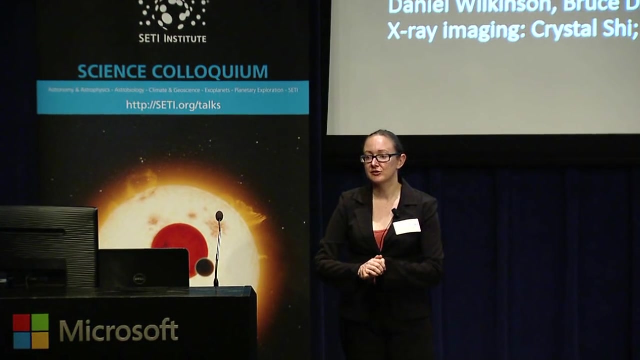 and gives you the ones in the age range. do they do anything in that determination of the age process that could alter what you're seeing? yeah, that's a good question. so what they do in the determination of the ages, basically what they do- they mount up the zircons in epoxy. 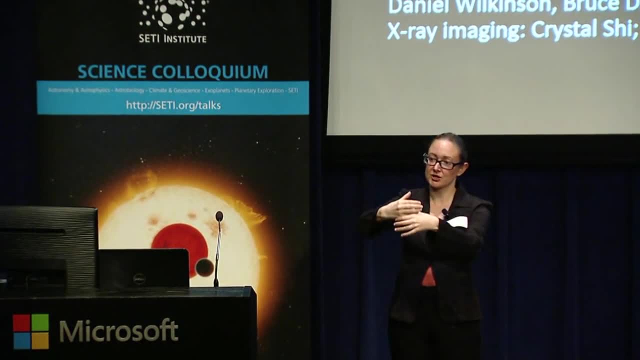 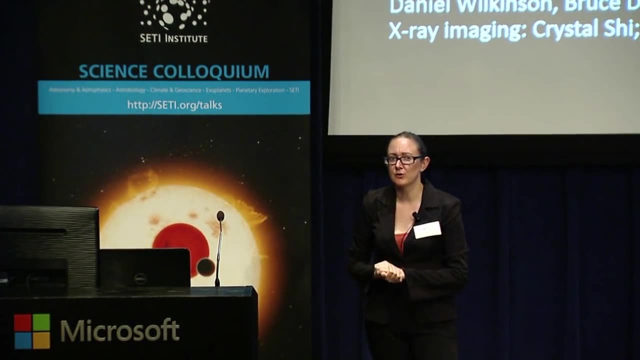 and then sort of polish them so that the midsection of the zircon is exposed, so sort of a primary oxygen beam comes in. there's also a process in which it's coated with gold, so these samples falling underneath the polished surface of the zircon- I mean the ion probe- is a very 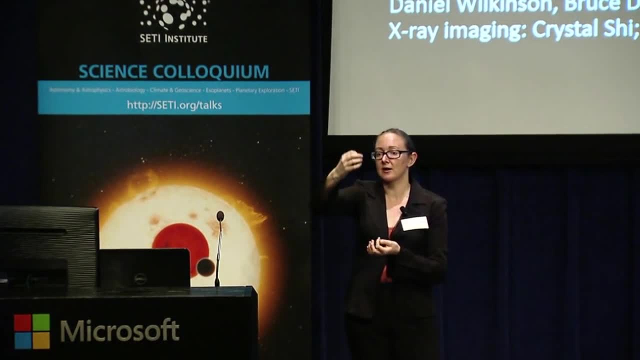 surficial technique. if you drill sort of our typical ion beams in one spot for an hour, you can get a micron or two deep, whereas our particular inclusions were around 5 microns deep, we think beneath our polished surface. so it's not something that would have.